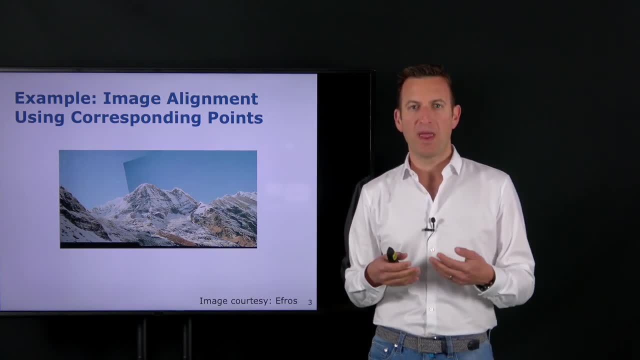 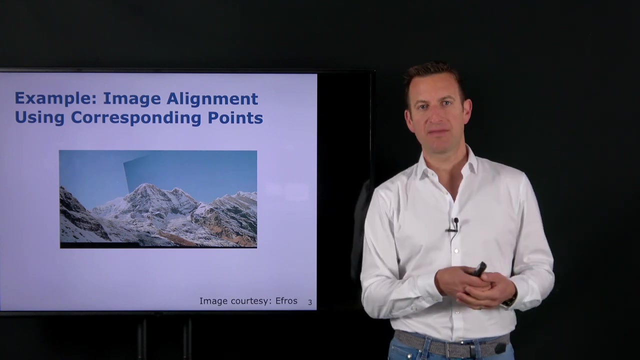 So there's one example where you have some information in image number one, a local image patch, a distinct point, something that you want to localize in the other image, And then you're looking exactly for that local patch of image information in the other image And 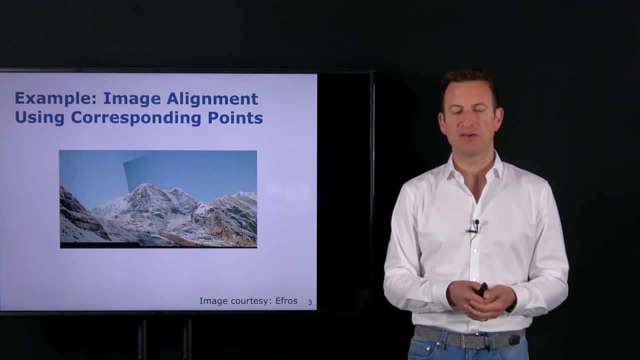 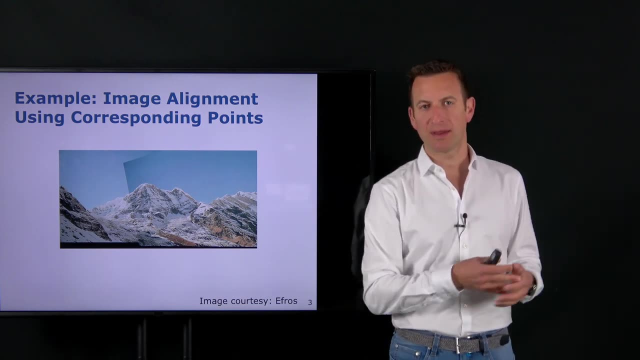 if you do this multiple times you get multiple of those data cessations saying which pixel in image number one corresponds to which pixel or which local area. So if you look at the image number one, you can see that there's a lot of data in the. 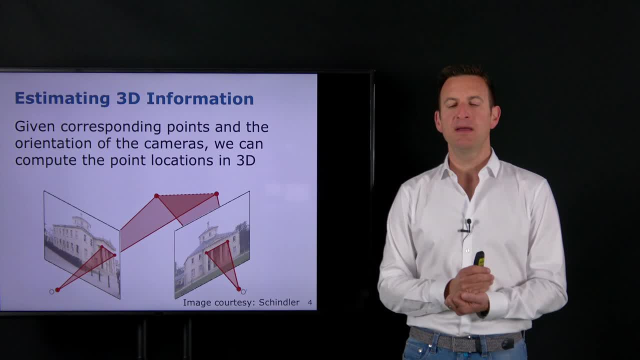 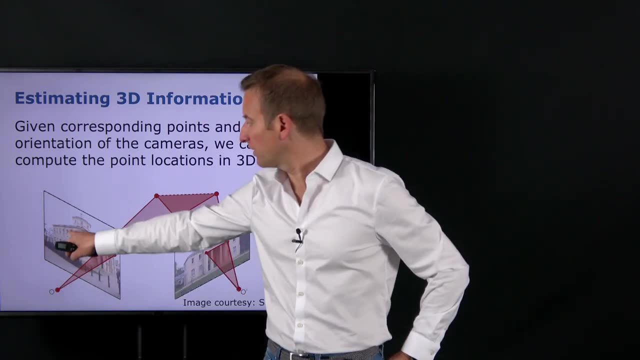 image number two. That is also pretty relevant if you want to estimate 3D information from image data using multiple images. So, for example, you have two images. It's kind of a stereo setup. So one image is taken from here picturing this building here from the one side, and the second 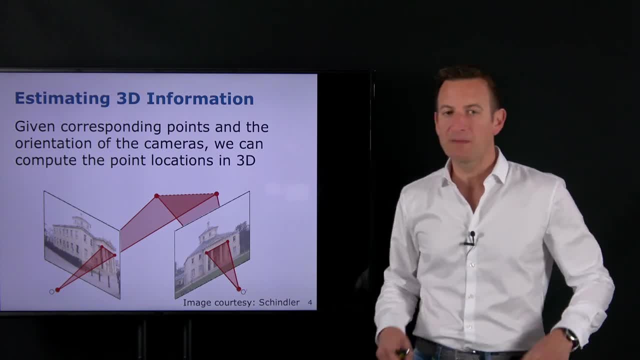 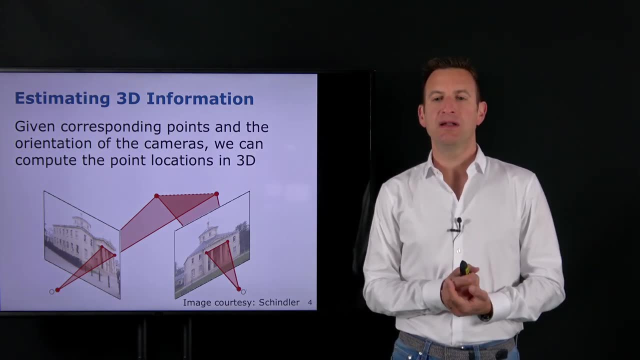 image of the building here, looking to the portal directly from the front, And you know where those images have been taken, Then you can use the images, as well as the location information, in order to perform a 3D estimation. So if you look at the image number one, you can see that there's a lot of data in the 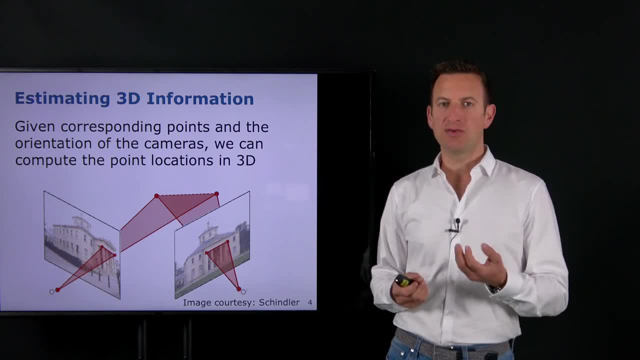 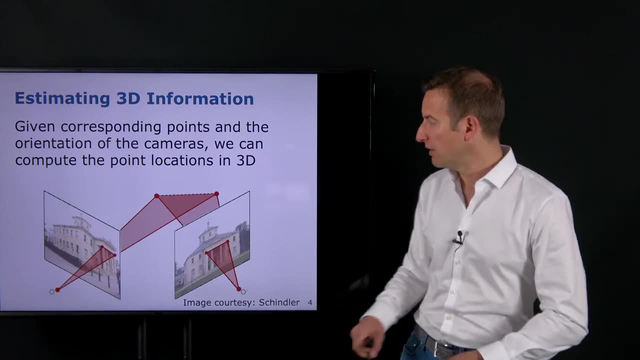 3D reconstruction. In order to do that, you need to know which pixel in image number one corresponds to which pixel in image number two, or kind of observes the same point in the environment, So that you, for example, know that this part of the building over here. 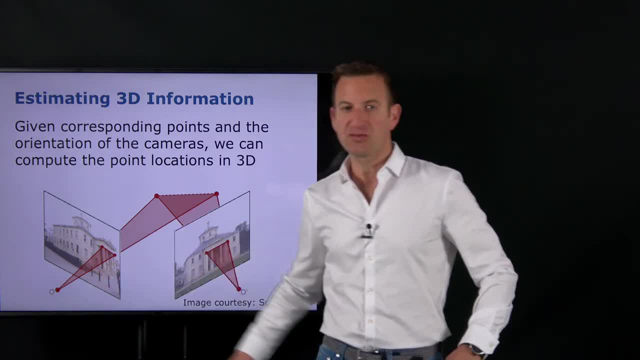 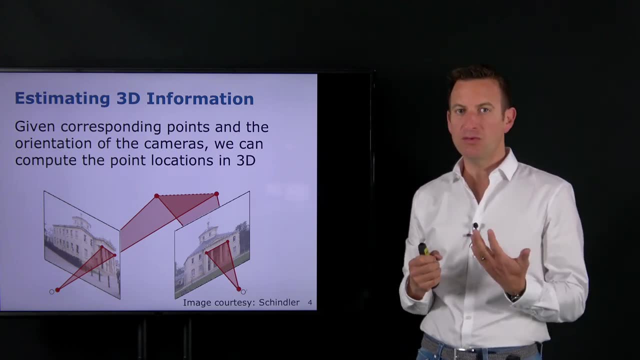 is exactly this part of this- building over here, so that you can perform this triangulation, So kind of intersecting those rays and then estimating the 3D location of that point- What you need to do for that is given you have kind of cut out, let's say one point. 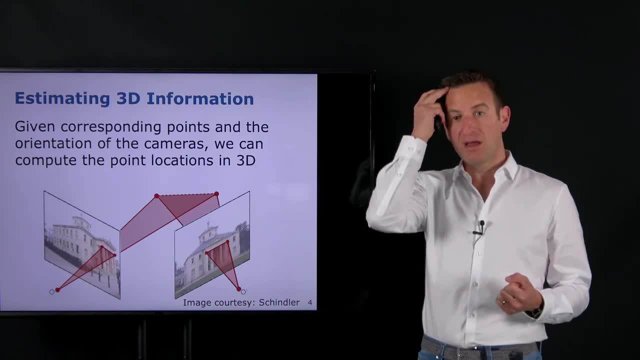 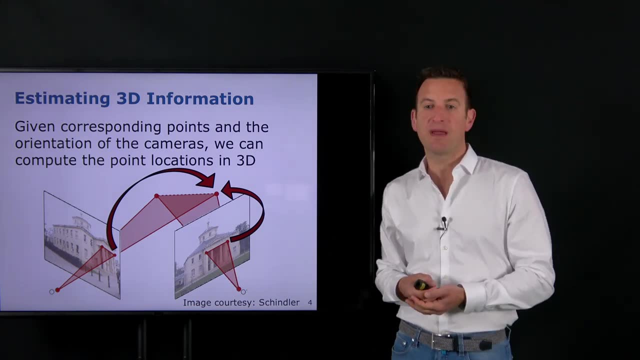 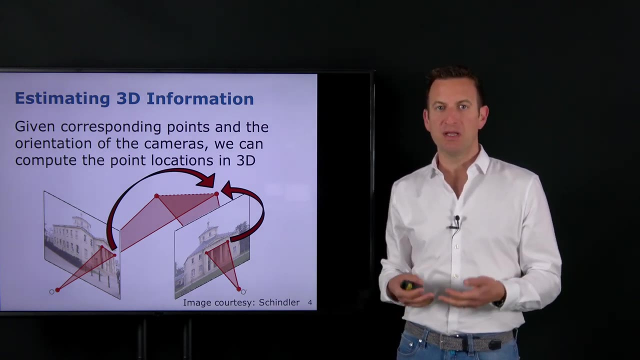 in image number one. You need to find where does this point sit in image number two so that you can use this correspondence information to then perform, for example, triangulation and estimate the 3D location of that point over here. So making data association between parts of an image is a pretty frequently done task. 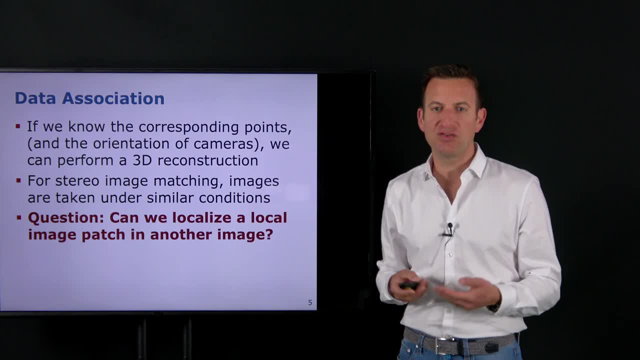 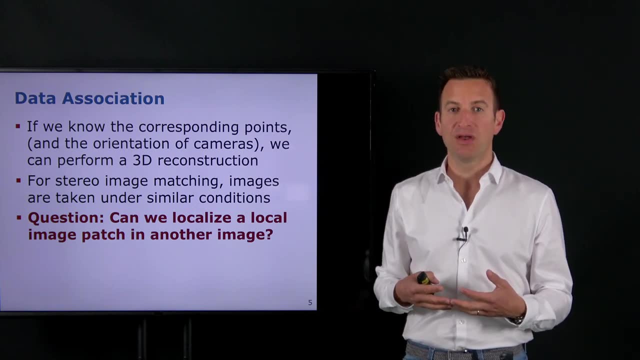 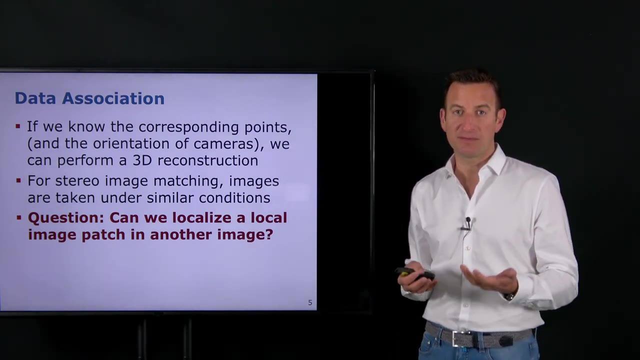 especially if you want to look into 3D reconstruction And data association is a challenging problem because there are so many different opportunities or possibilities that you have and also so many opportunities for actually making mistakes and making wrong data associations. And wrong data associations are harmful for state estimation algorithms. So if you have 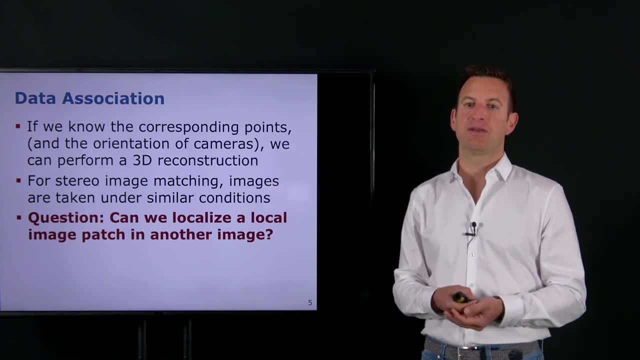 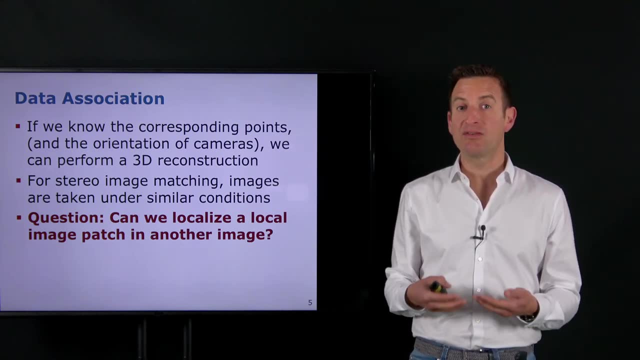 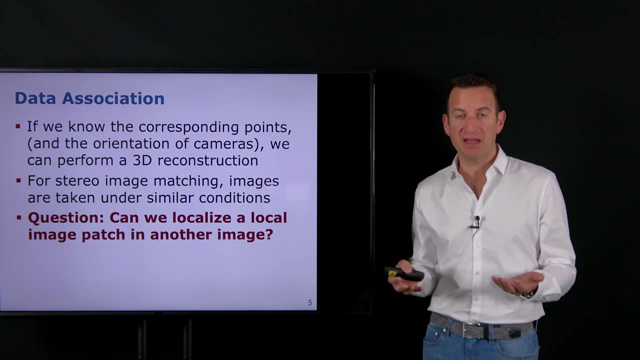 outlier measurements. this can negatively impact your state estimation. Therefore, you want to invest quite some brainpower in your data association scheme in order to get as good as possible data association. You will not be able to kind of avoid data association mistakes all the time, but you 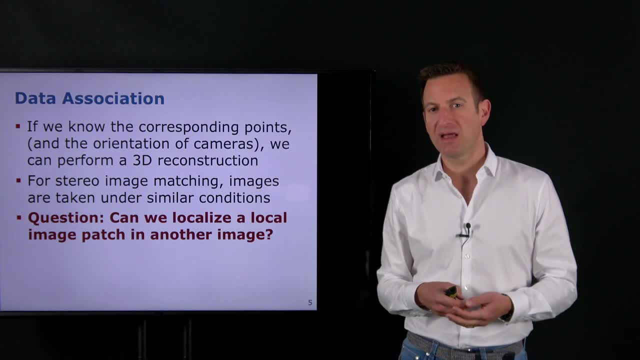 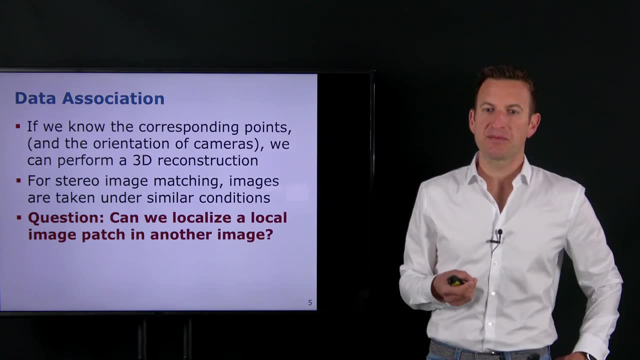 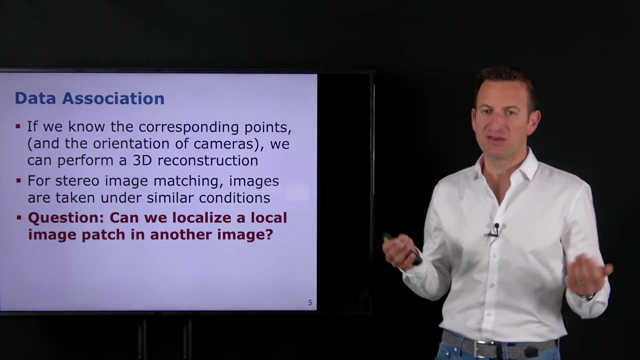 want to look into your data association- Next slide data station to see how can we do that as good as possible. So, and we need that data station, for example, for estimating three locations of points, estimating geometry, but also for other tasks, if you want to find kind of similar images. 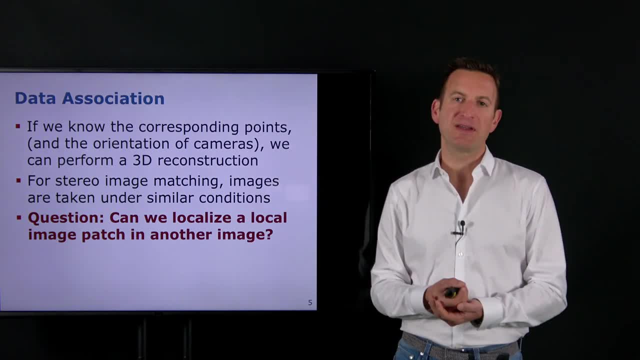 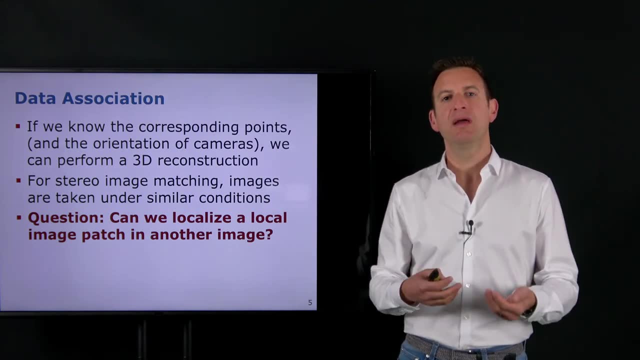 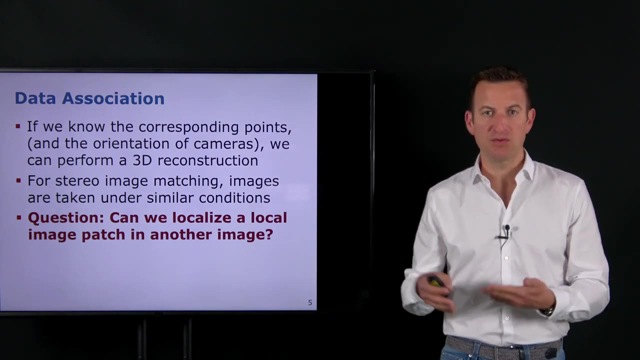 those kind of data stations play an important role, especially, but especially, if you have multiple images taken from the same scene with exterior camera or with a moving camera and you want to identify what you've seen in image number one. to which pixel does this correspond in image number two, three? 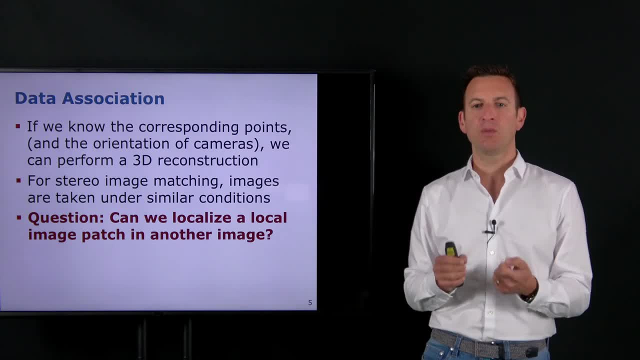 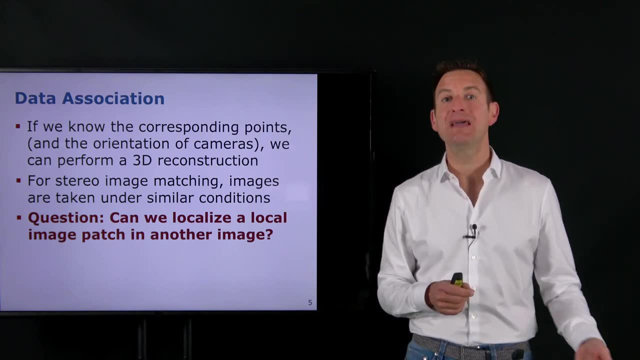 four, five and so on. So the question is: how can we locate a point or, let's say, a local patch of a local region that I have given from one image in another image? So you basically have a small query or template image, which is tiny. 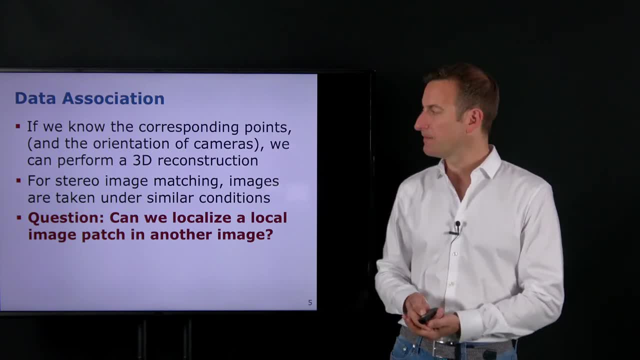 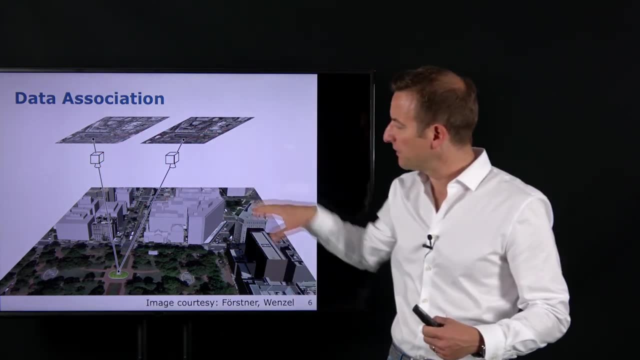 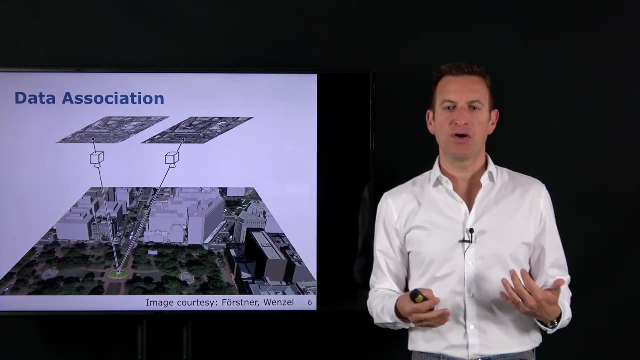 small region and you want to locate that in the other image. So what another task we may want to do? this is, let's say, you have an aerial vehicle and you're flying over the ground. you're taking pictures from the ground and you take images at two different points in time where your airplane or your drone? 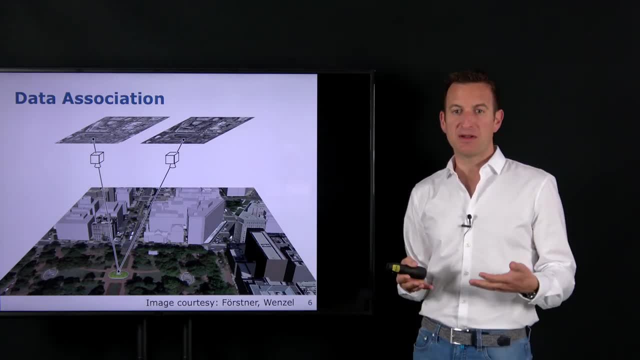 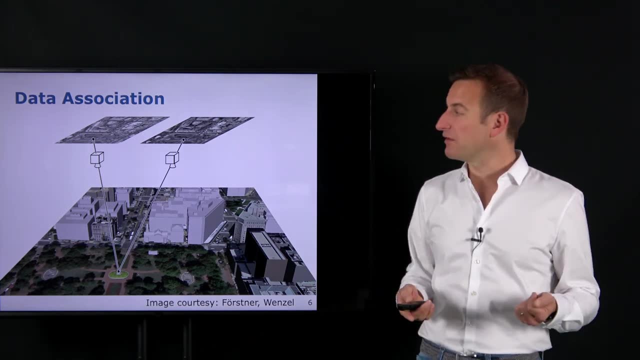 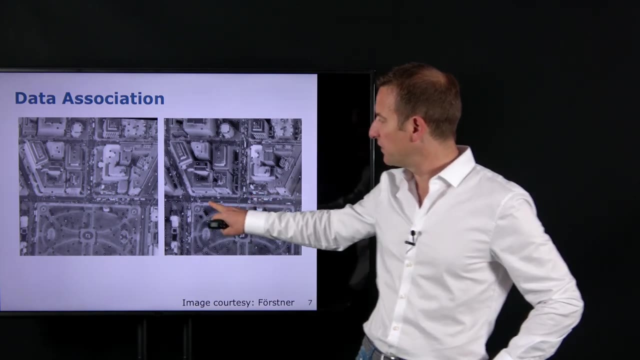 has actually flown a bit and you take an image, so it's picturing the same scene, let's say, a few seconds later, but from a different location, and you now want to make this data station. So these are two examples of these aerial images, also showing some kind of distinct points here. So some areas where some 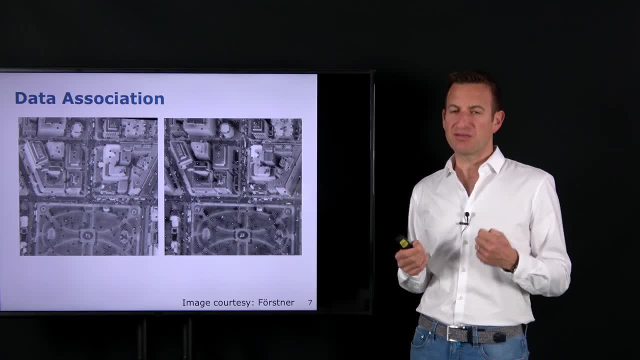 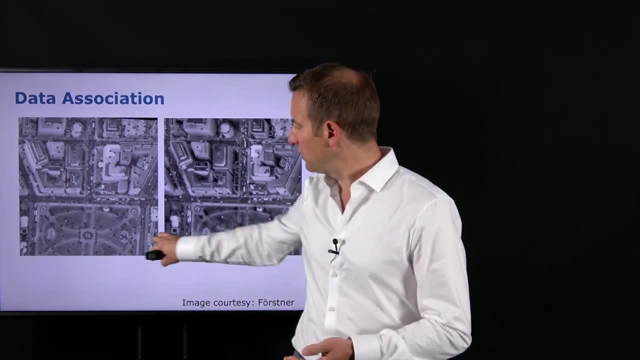 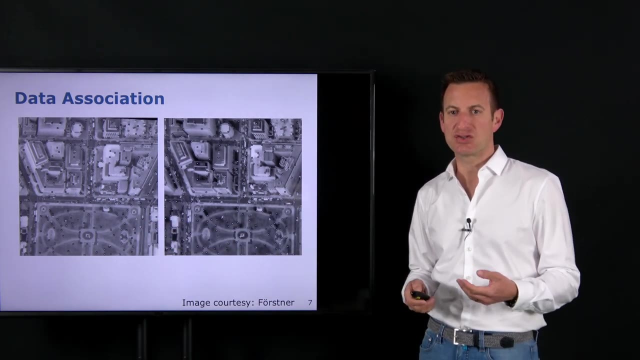 algorithm has said: okay, that's a point which kind of locally stands out, so this may be a good point in to find that location in the other image. What you can also see here- hope you can actually see that in the video- that the brightness and contrast between those images has slightly changed. So you also want to do. 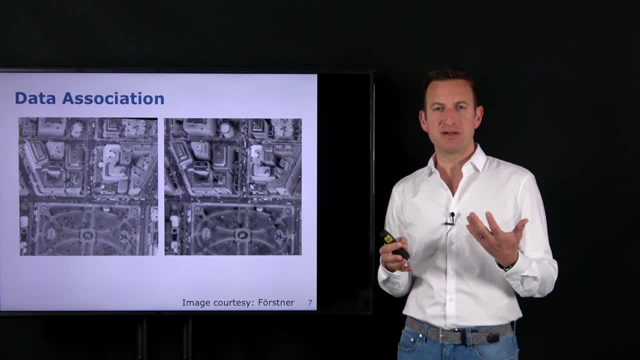 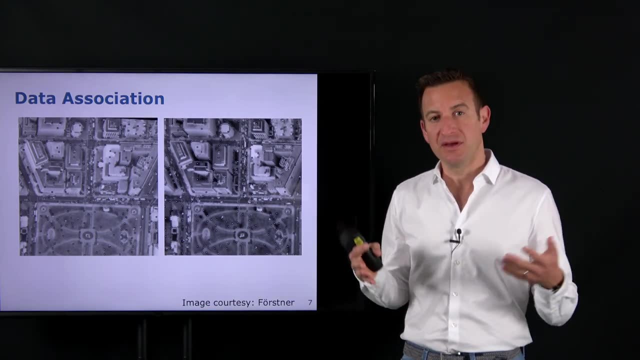 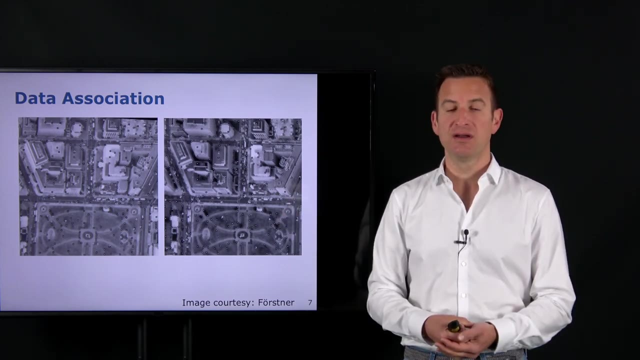 this form of matching under similar conditions, but not exactly the same conditions. Obviously, you want to have pictured the same scene and most of the time, the time spent between taking image number one and taking image number two is not too large, at least in this application over here, So it's maybe a few seconds or minutes. 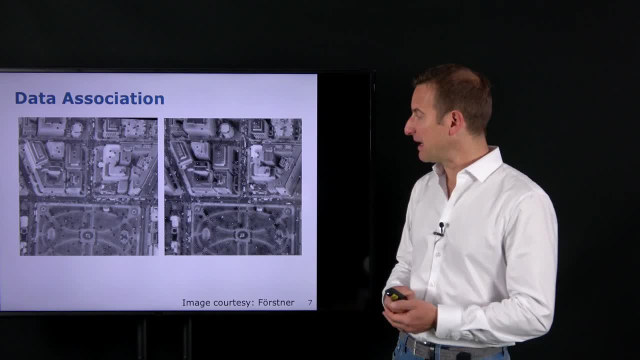 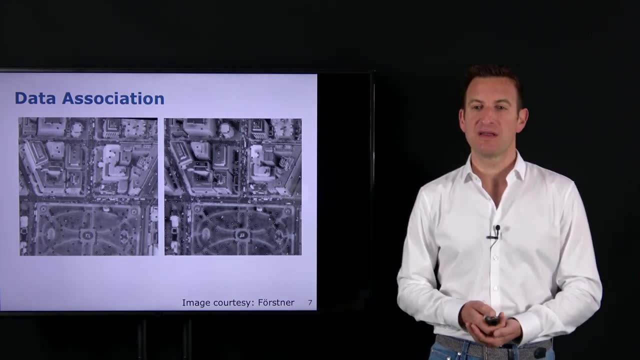 but not days, weeks, years or decades, Although there are clearly applications for doing this, but then maybe cross correlation. the technique we are discussing today may not be the best choice, But what we have, even after the, in this short time spans, is that we have different exposures of our 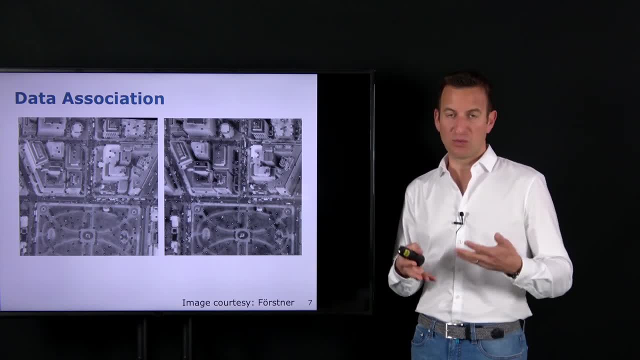 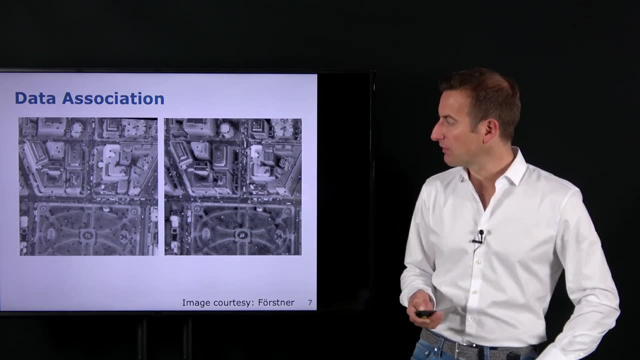 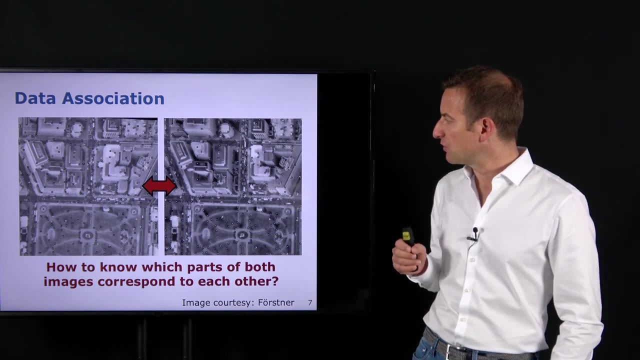 camera. Sun may come out, your camera might trigger different exposure. so there are reasons why the images, for example, change in brightness or also in contrast. And the key question is here: how do we know? how can we know which part of the of these images correspond to each other? So, for example, if you look, 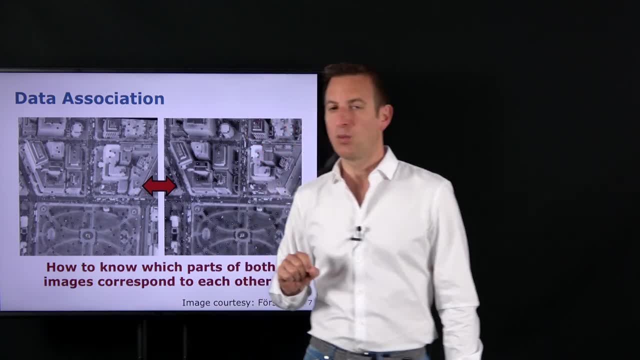 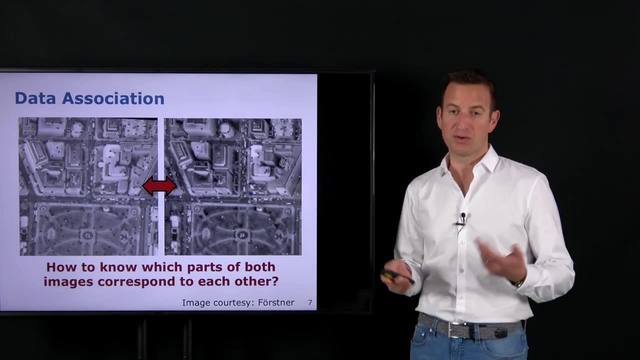 to one distinct point at this point over here. where do I find this point? the other image, image. How can I figure out that this is actually this point? And that's what the approach template matching with cross correlation is all about, and that's what 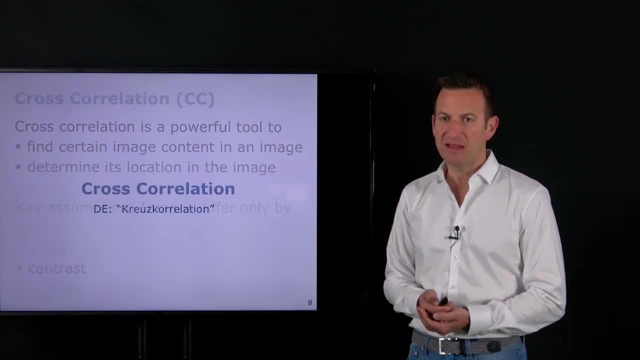 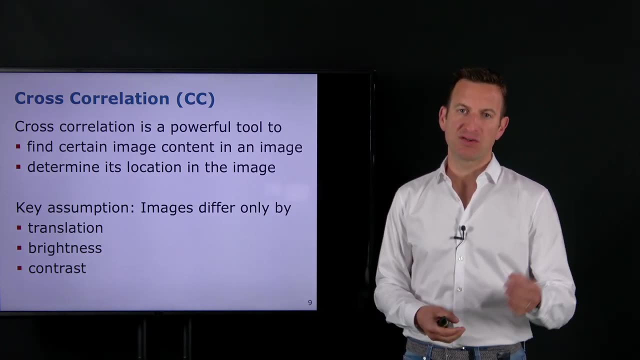 we're going to discuss here. So cross correlation is a technique that I can use in order to find image content in another image and also find its location. So I have a small image region. I say, okay, I want to find this and I don't. 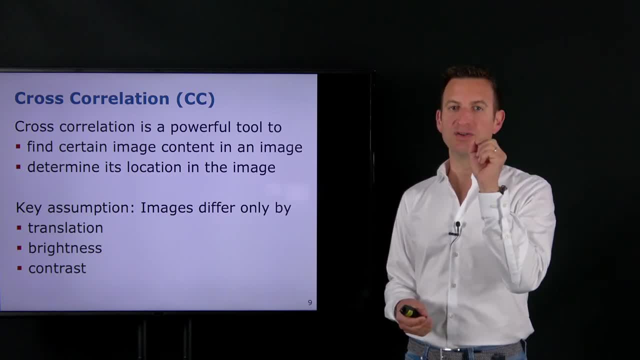 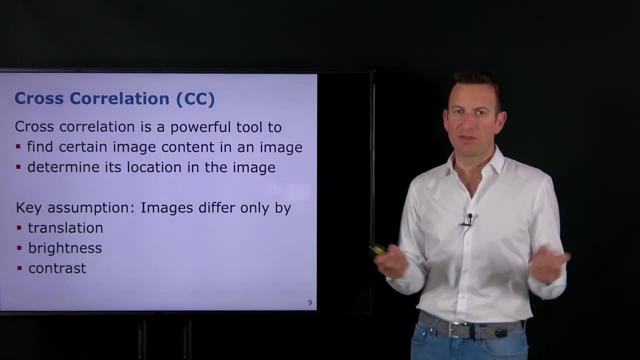 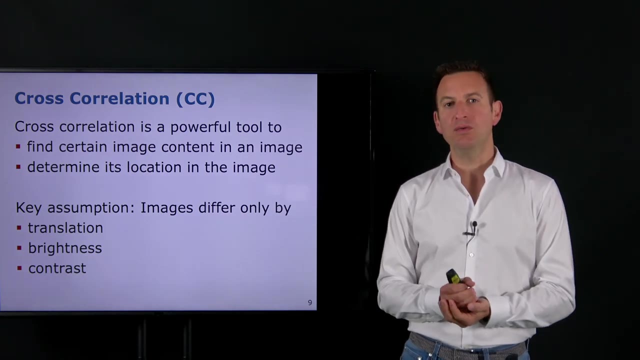 only want to know that it's in the other image, I also want to determine its location. So, okay, it's exactly at pixel 100, 180, for example. And with all those approaches, we need to make assumptions and the assumption basically tells us under which transformations we want to do this matching and what cross. 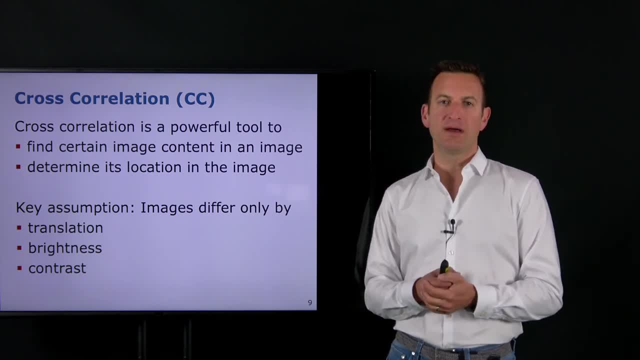 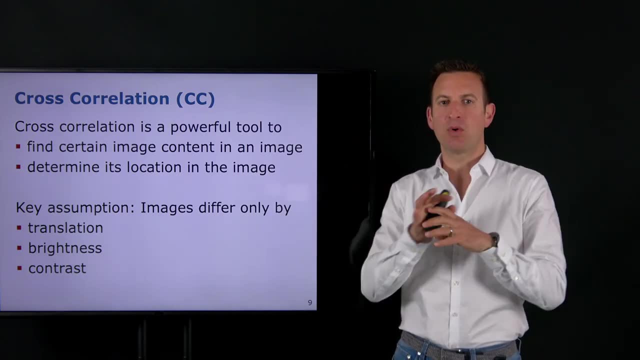 correlation takes into account is that there's only a translation, so a shift in the image. so both images have just shifted, not rotated, for example. So if you have an image, number one- and you rotate your camera or you're flying a curve with your UAV, you make many 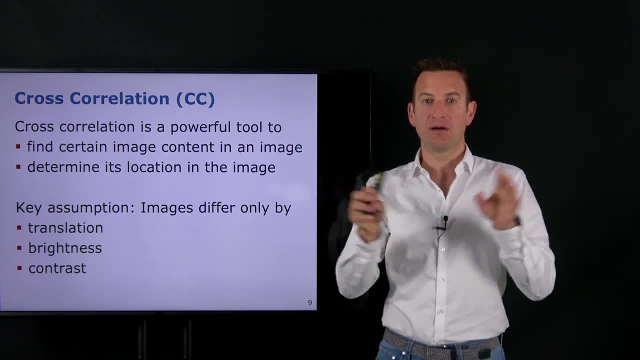 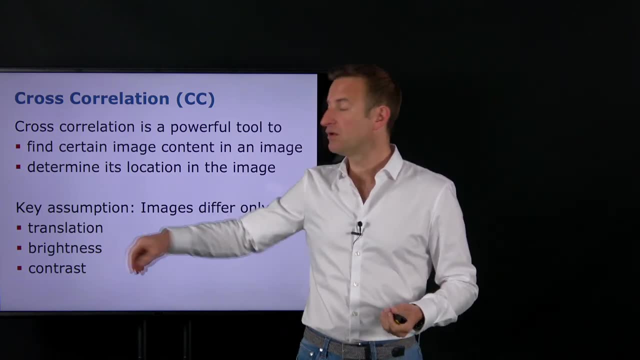 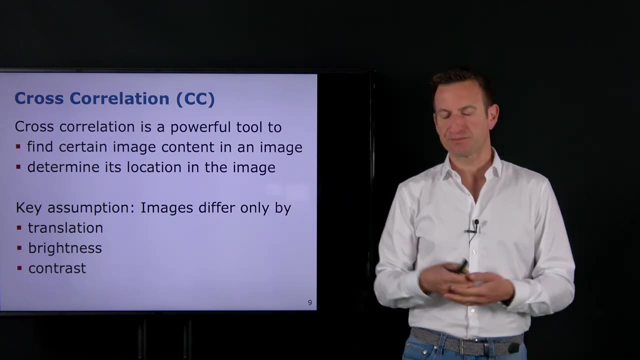 you're kind of rotating your image, let's say by 45 degrees, and although those images overlap and you want to be able to find correspondences, this would be the wrong approach because it takes only into account translations over here You can extend cross-correlation to also take rotational offsets into account. 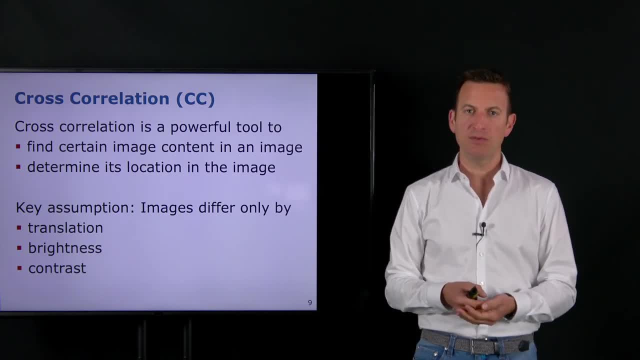 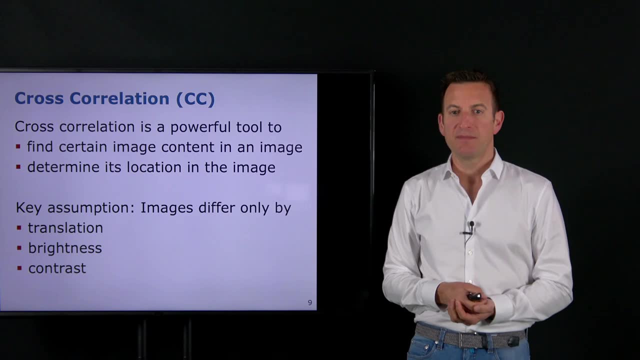 so you can extend that. It gets computationally more complex if you do that, but you can do that. But the basic cross-correlation, as we discussed here, only takes into account translation. The second thing that the cross-correlation takes into account. it says: 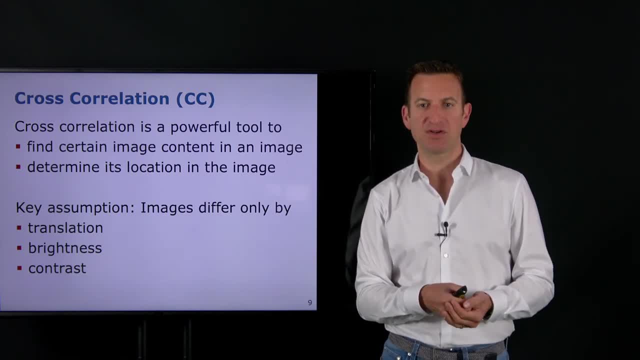 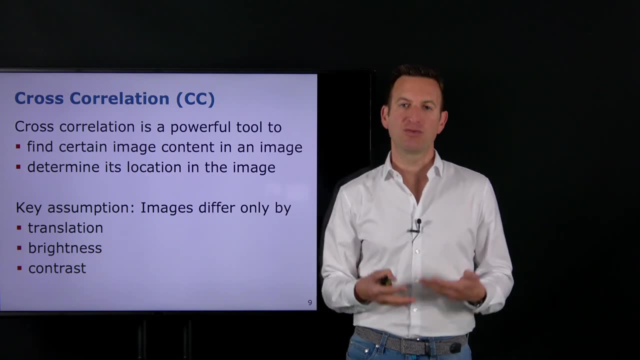 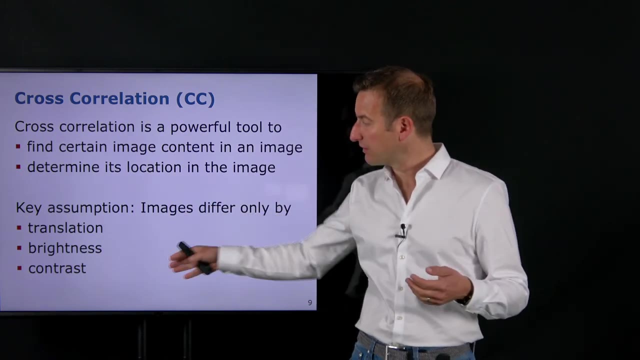 it should be okay to have brightness changes and changes in the contrast in the image. So you want to find two images which differ only by a translation, in their recording location and by contrast and brightness changes, And if you do that, then, or if you want to work under these constraints, 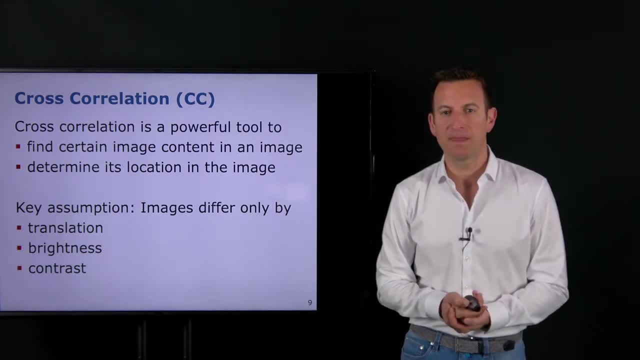 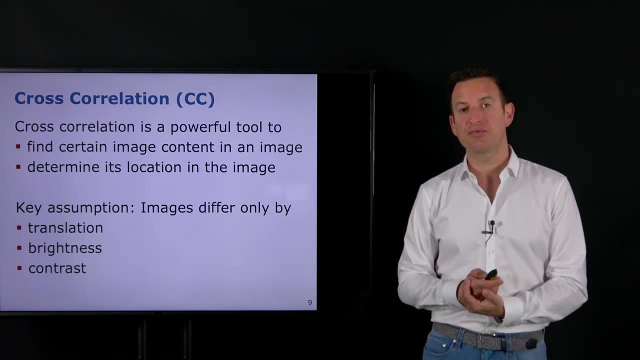 cross-correlation is the standard technique to do that. Okay, So now let's go into a concrete example, because cross-correlation is actually fairly easy to understand if you simply go through the individual steps and can actually explain that in a rather straightforward manner. 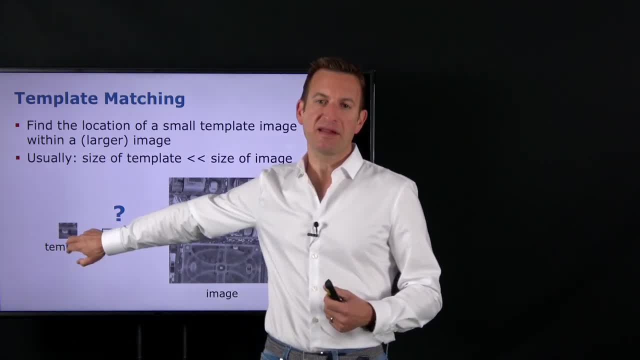 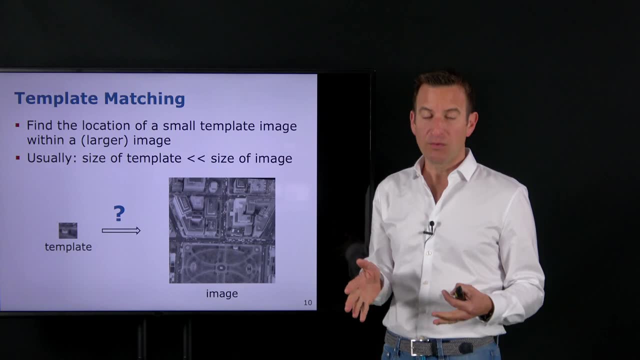 So what we want to have? we have a template, a local region, the thing that I want to localize in my larger image. Typically, you have a large image and a small template, or the template is smaller and often much smaller than the original image. 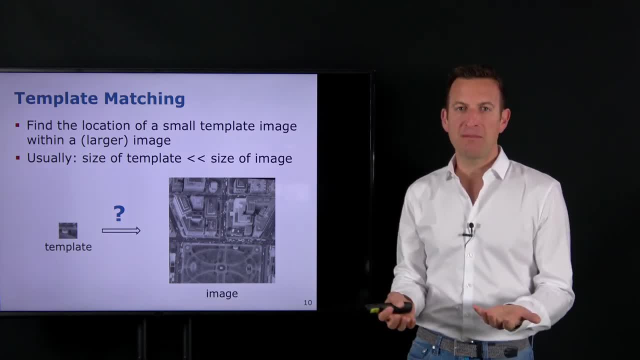 And the goal is to find this template in that art image. This template, again, is typically generated by a large image. This template, again, is typically generated by a large image. This template, again, is typically generated by a large image. 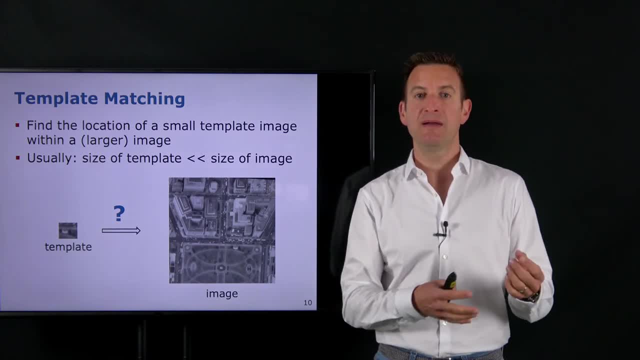 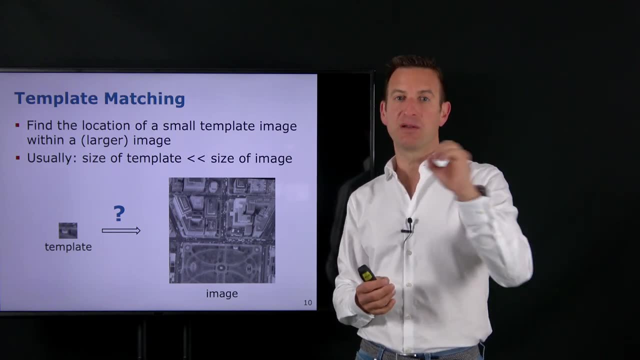 This template again is typically generated from your image number one, from your initial image. for example, You cut out a part. we say, okay, that looks interesting. that's a distinct point. that's the location or the patch that I want to find in the other image. 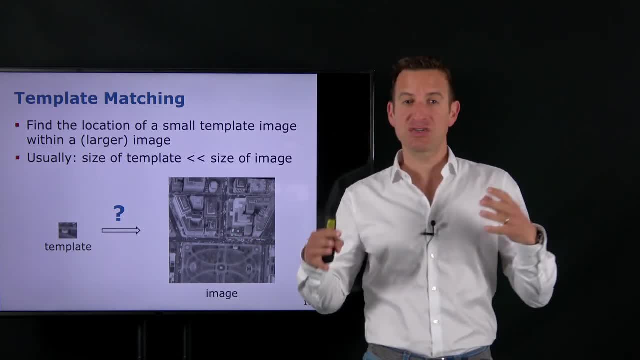 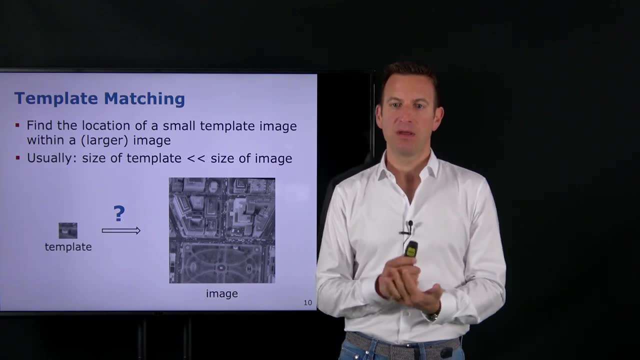 So that's your template. And then you take the second image, which is now the large image, and you say, okay, where is that template or that local patch located in the other image? And what you want to the information you want to get out, say, yep, here it is at that location. 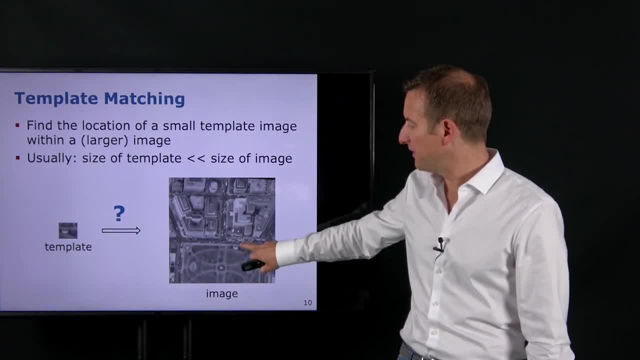 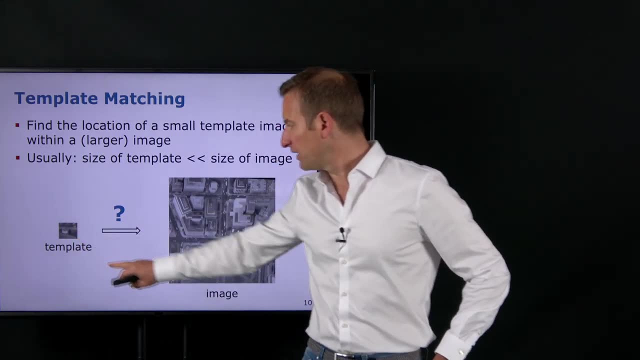 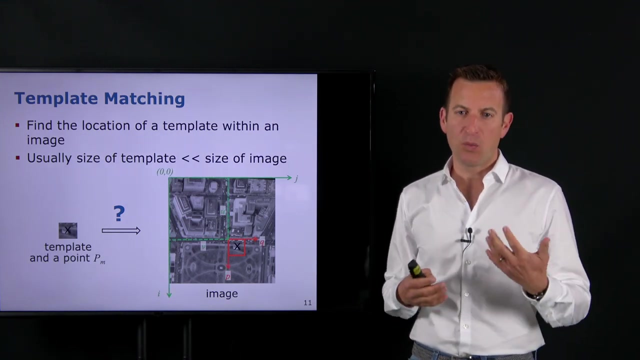 So if you look to this template, then we may be able to identify that this actually is this location over here. So this red box over here shows the overlapping area of the template with the image. In order to locate it. we want to have an offset where that location, where that patch, is. 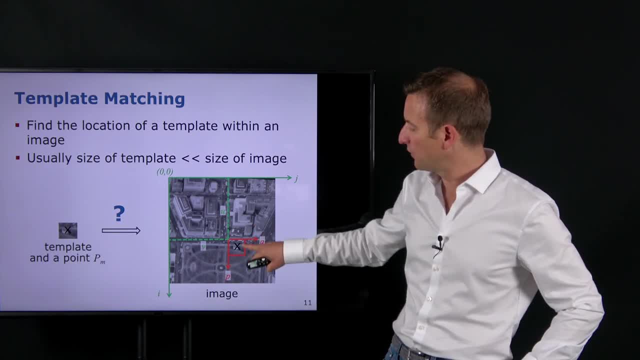 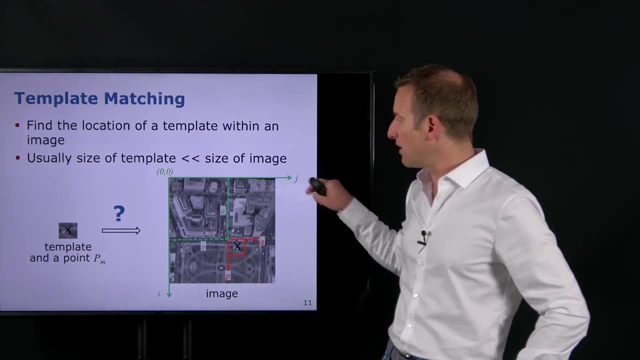 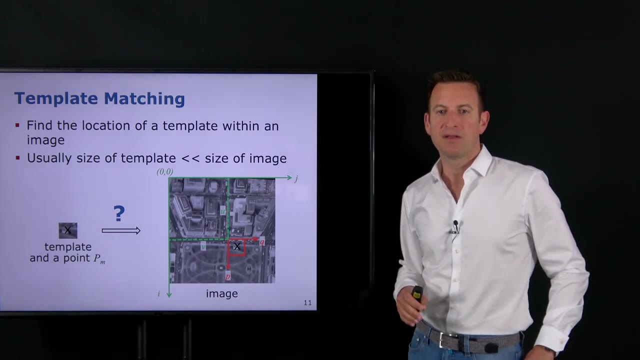 So there should be a transformation between the local coordinate system of that template over here, which is here written as Q and P, and we have I And J over here in our original image. Then there's an offset indicated by U and V that describes where the 0, 0 location of my patch is. 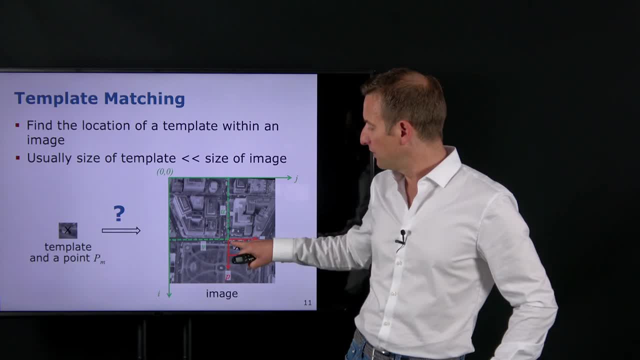 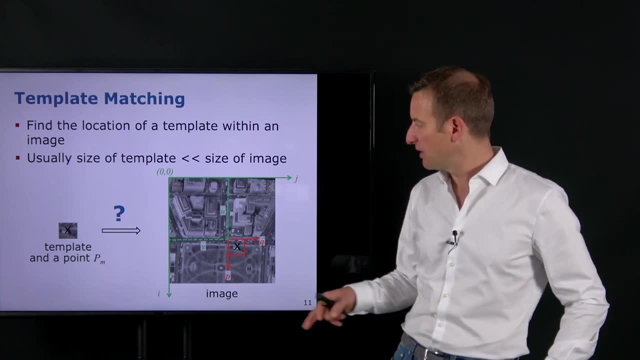 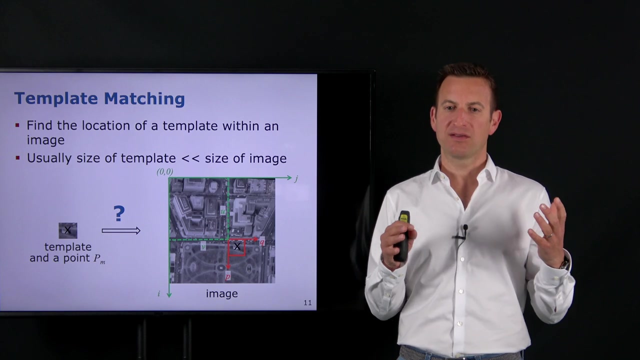 So let's say 0, 0 in the red in the template. where is it matched to? in the original image That would be V and U. Okay, So the U, V or V U vector is basically the shift vector. 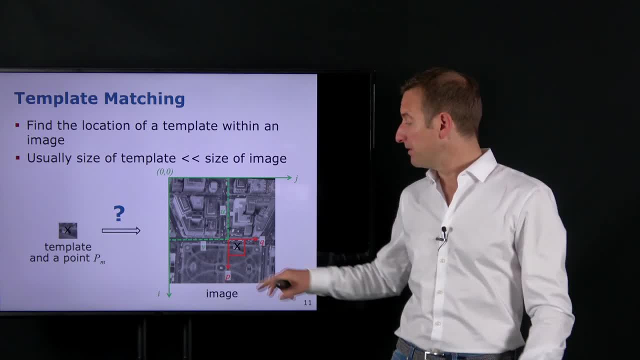 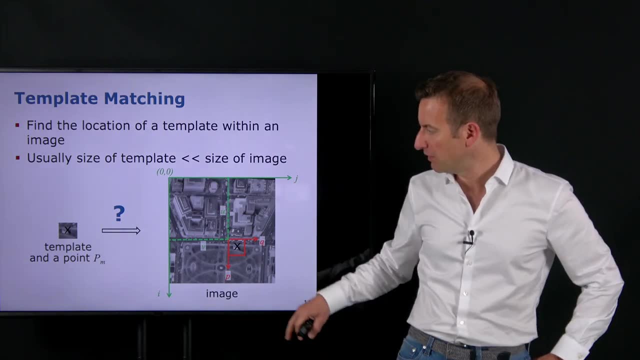 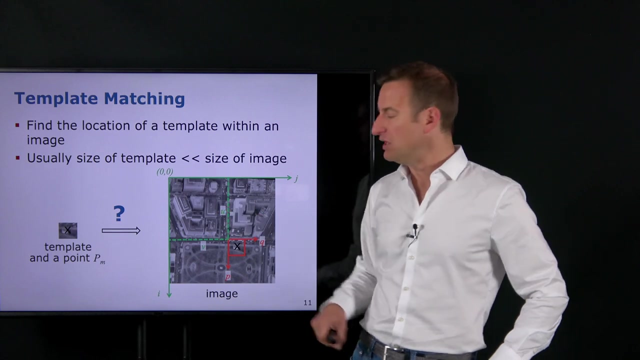 that tells you the translation of the template and let's say a point in that template with respect to your original system. So you have a point P which is expressed in this kind of red coordinate system and by adding V and U to these coordinates. 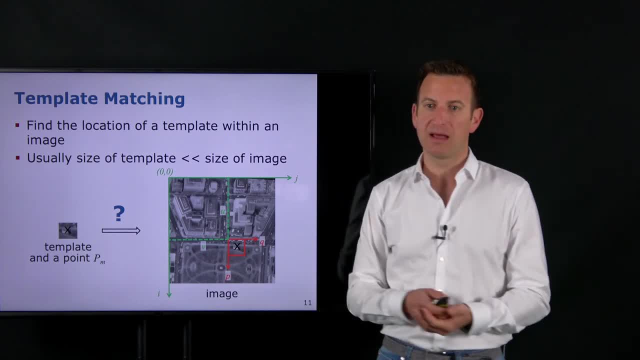 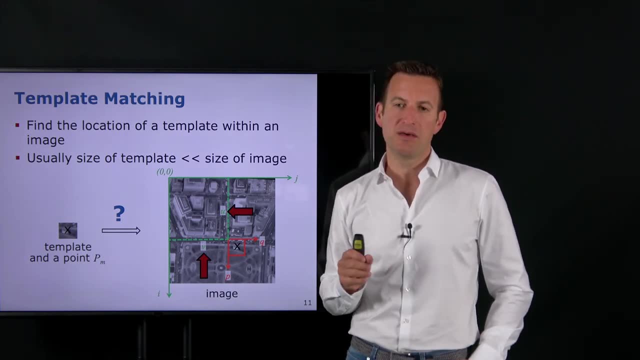 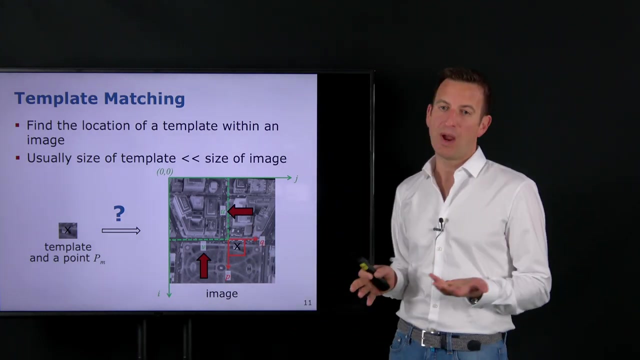 you can express where that point is in the larger image over here. So finding those offsets V and U are those two things which I'm interested in. So I want to find those offsets because once I have those offsets then I know where that patch is located in the other image. 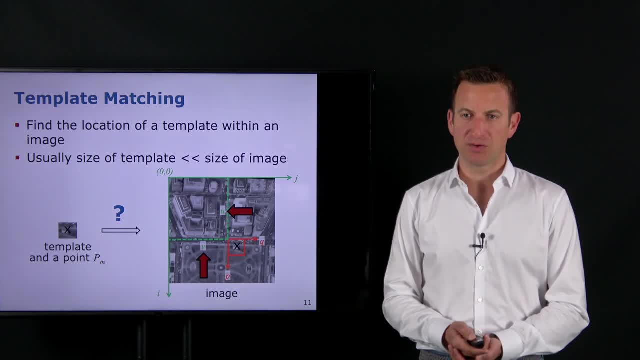 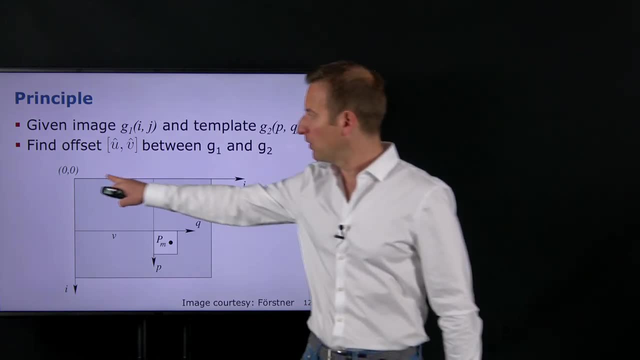 and I can exploit this information for my further state estimation processes. Okay, so, given we have an image which we call G1, this is kind of our large image, so the big one over here that's G1, and we have the template G2, this is kind of my. 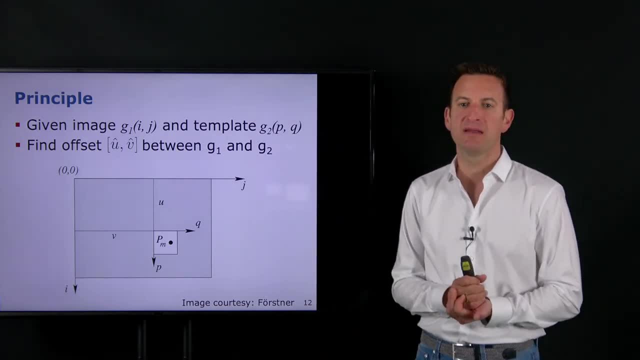 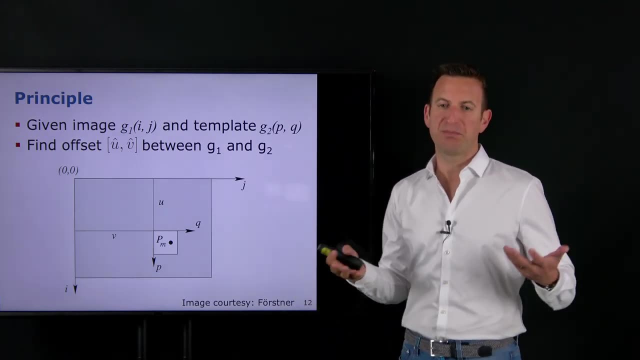 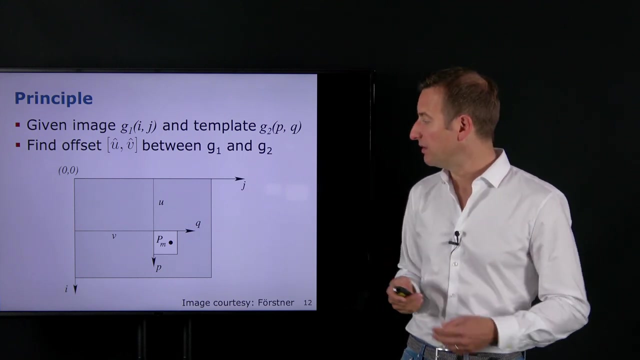 my small patch, that I want to find my template. Then I'm interested in finding the offset U and V, between G1 and G2.. So I basically want to find the offsets in the X and Y direction or I-J direction for computing. 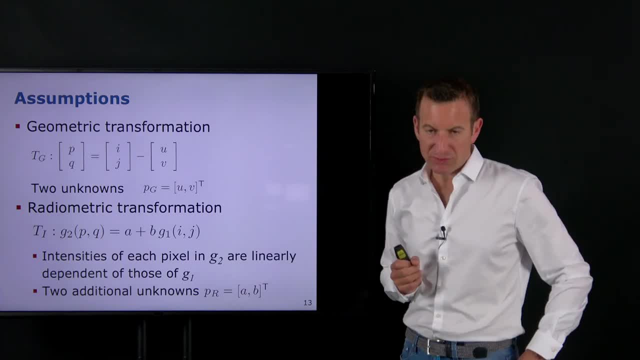 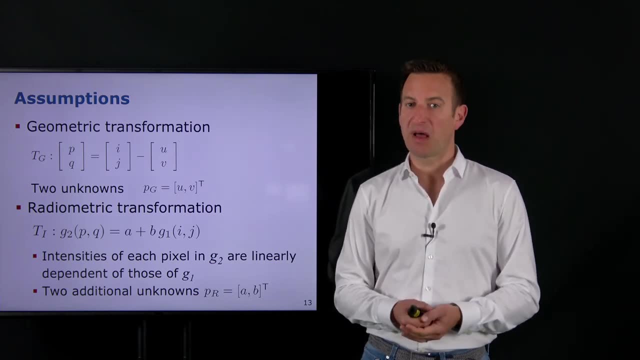 this offset vector over here, So we can express this as a geometric transformation and if you remember geometric transformations, these are different ways how I can transform one image into the other, and you can do this, for example, with an affine transformation. 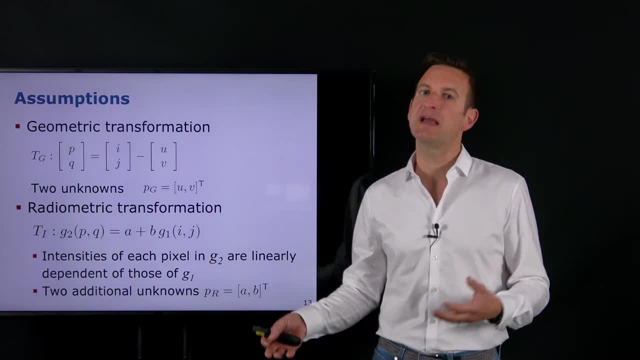 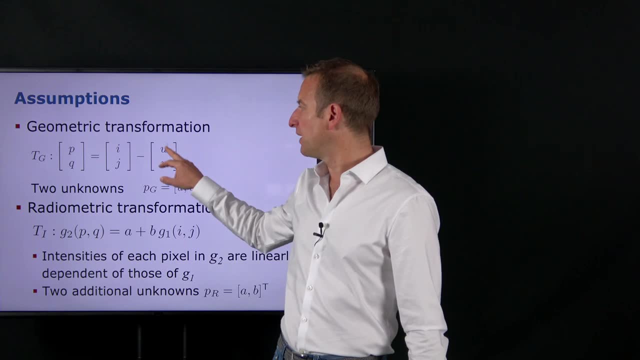 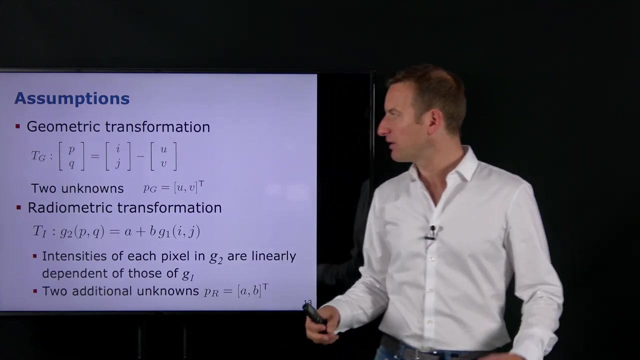 or similarity, transform or rigid-body transform or rotation or translation, And again, we are looking here only in translation. So we say one coordinate is the other coordinate minus this offset, this shift vector. So this here is our shift vector, which tells us how one is mapped into the other. 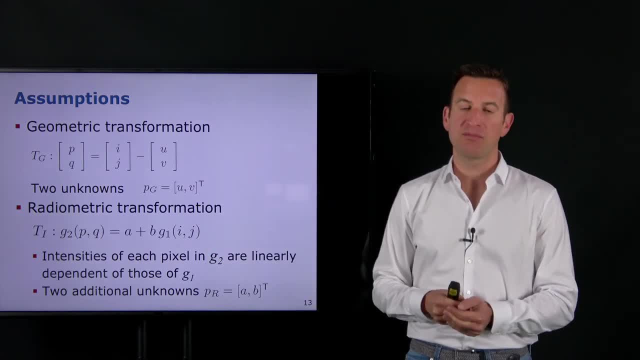 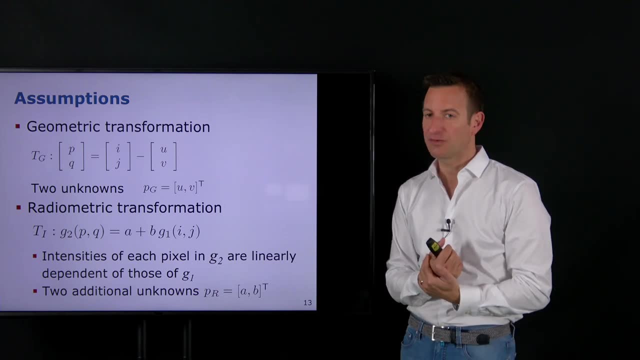 That means we basically have two unknown parameters for our transformation, which is just this two-dimensional shift. So I'm just shifting this small template in the other image, I'm not rotating it. Well, this is kind of the geometric transformation that we are taking into account. 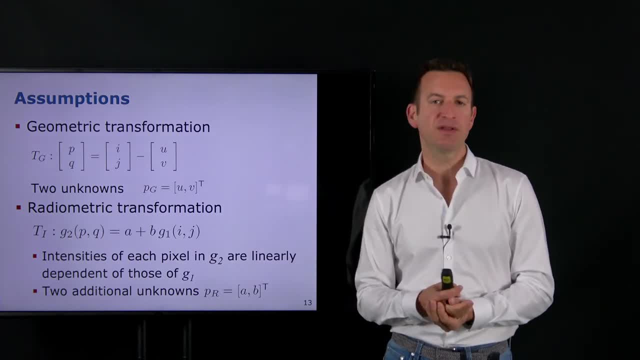 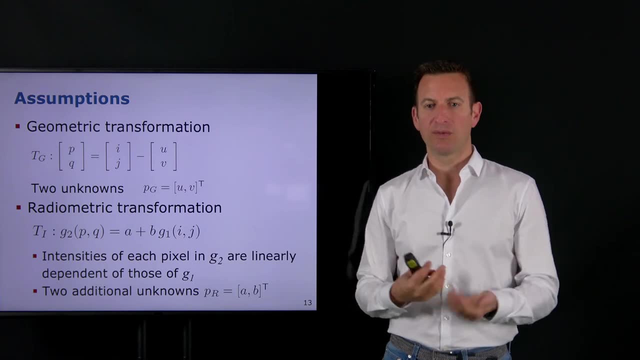 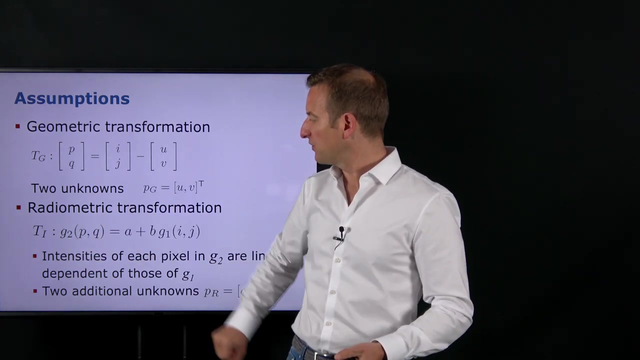 There's also a radiometric transformation we want to take into account, and this is a transformation that accounts for the difference in brightness and in contrast, That's what we want to be invariant under. So we say the grayscale value in the template must be a constant offset plus a scale factor. 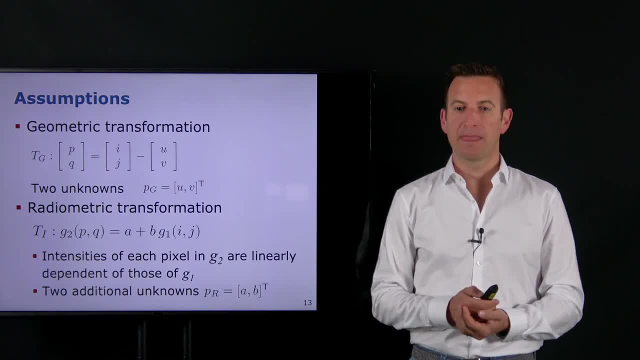 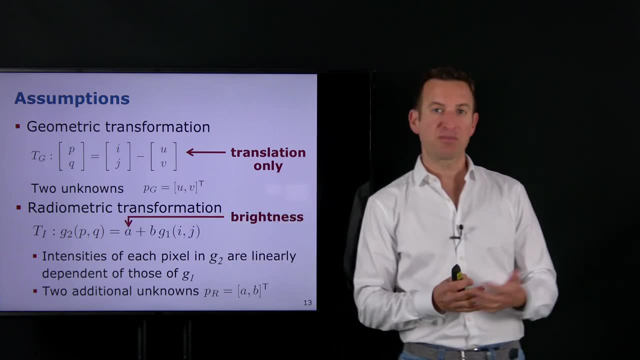 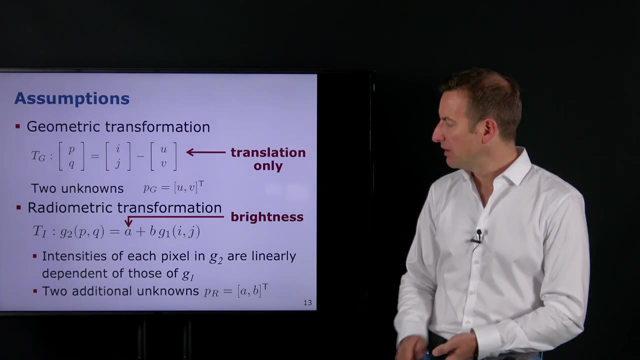 of the intensity value in the template In my large image. So this is our translation-only constraint and this A indicates the brightness, because by adding a constant I'm increasing the mean. By increasing the mean I'm increasing the brightness of the image. 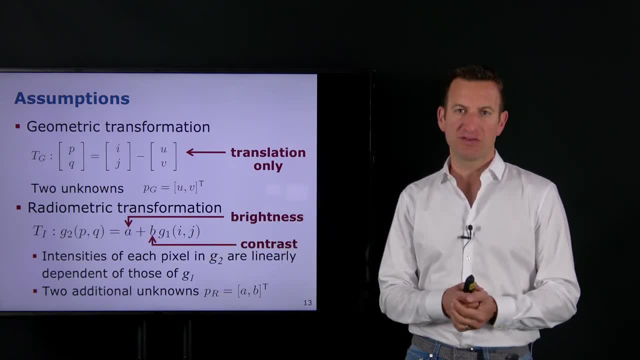 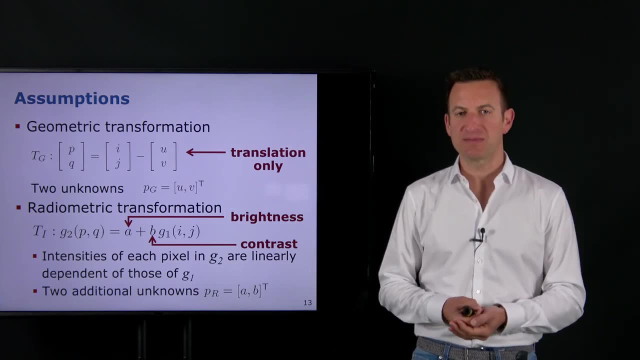 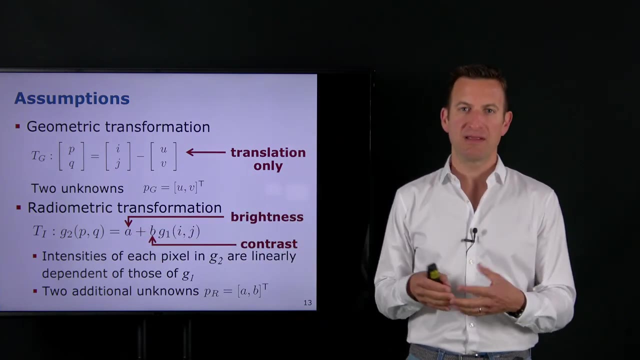 And the factor in front of the intensity value changes the contrast of the image, increases or decreases the contrast. So it's something that we have seen in our initial operations when looking into histograms and transformations of images, That the change in brightness is a change in the mean value of our intensity values. 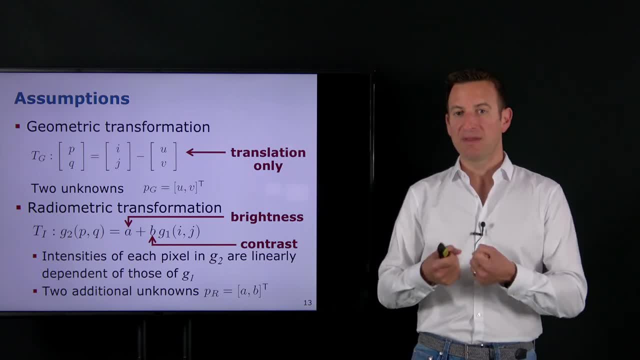 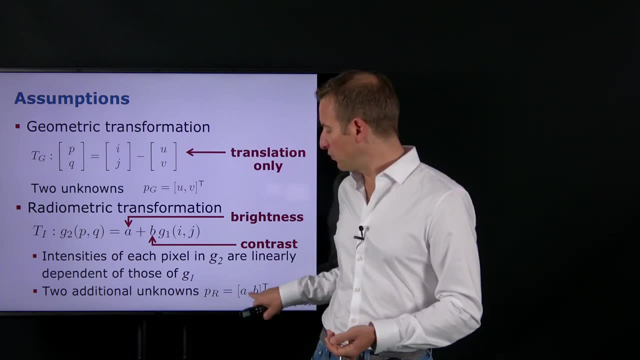 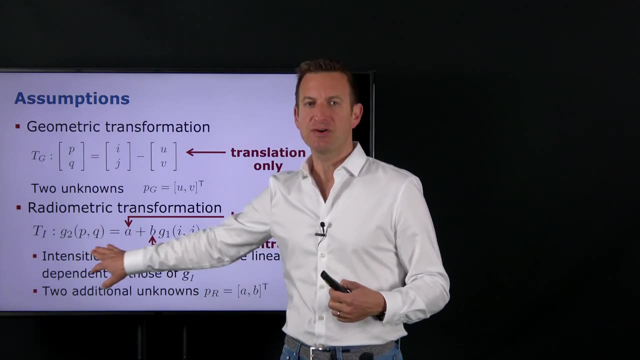 and by multiplying this I'm actually changing the variance and thus changing the contrast of my image. So again, this gives me two further parameters, A and B. So in the end I have four parameters. I want to be invariant under those parameters. 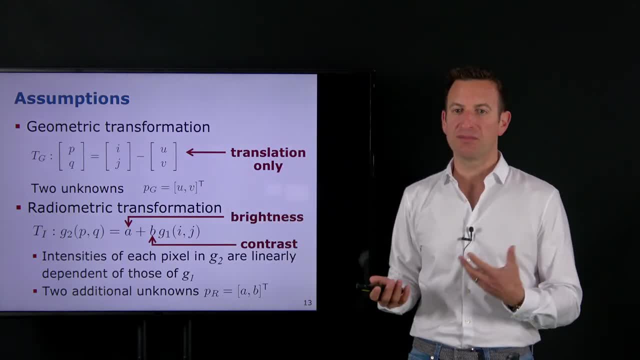 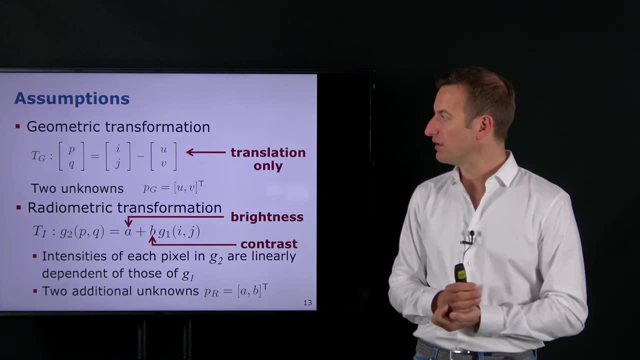 and I want to return those two parameters over here, But these are kind of the free parameters. These are the parameters that I need to take into account in order to find a solution over here And again. this is the result, And those parameters A and B I may not be explicitly interested in. 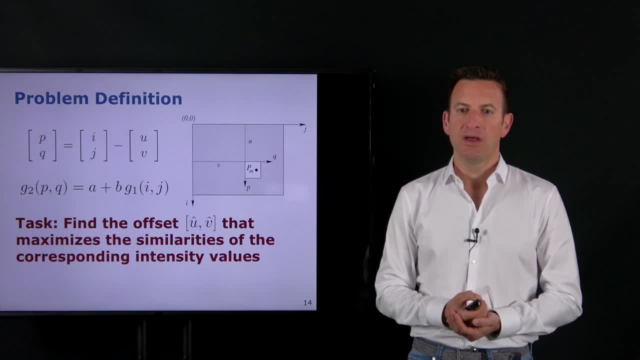 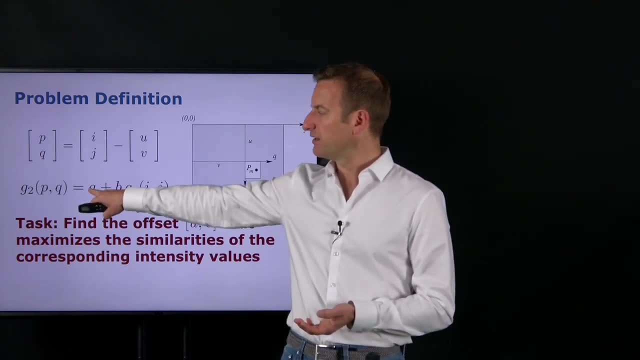 but I want to be invariant under those two parameters. So my problem definition is basically finding this UV vector, this offset vector, under a transformation of the intensity values, which may look like this: And what I want to do is I actually want to find the location. 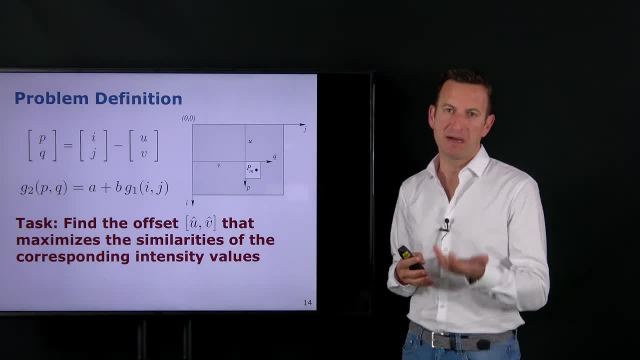 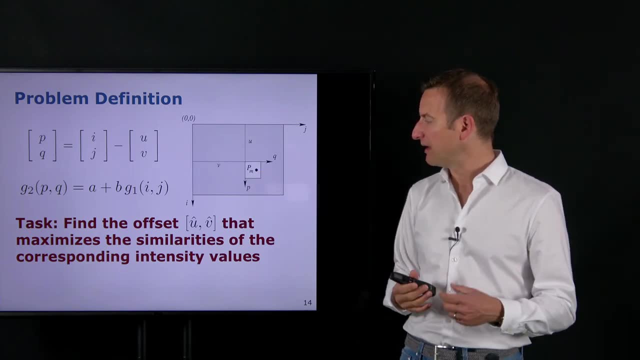 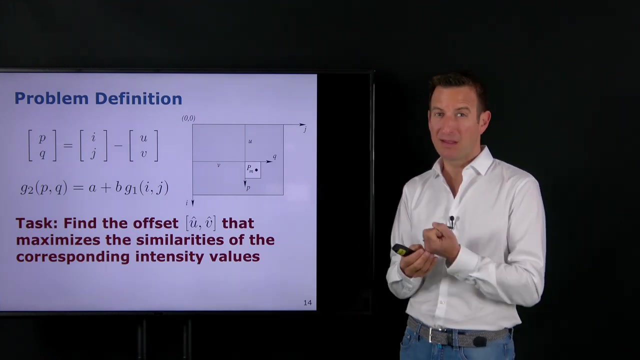 so that I'm maximizing the similarity between my template and my image. So if I compare that template with the overlapping area in the original image, then I want to maximize the similarity. It may not be perfect. It may not be an absolutely perfect match. 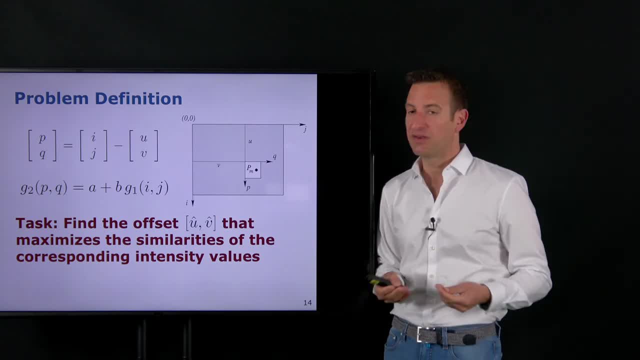 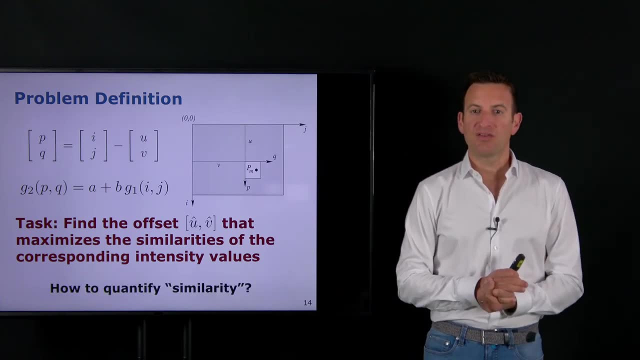 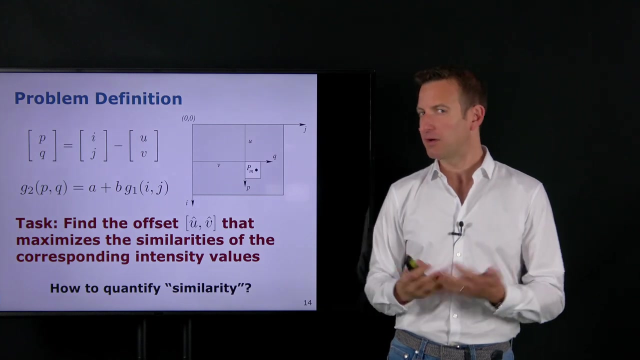 There may be some noise involved in this, but I want to maximize the similarity or minimize the difference between both. So the key question then is how to quantify actually similarity, How to say that two images are the same or are similar Or the same, would probably be easy. 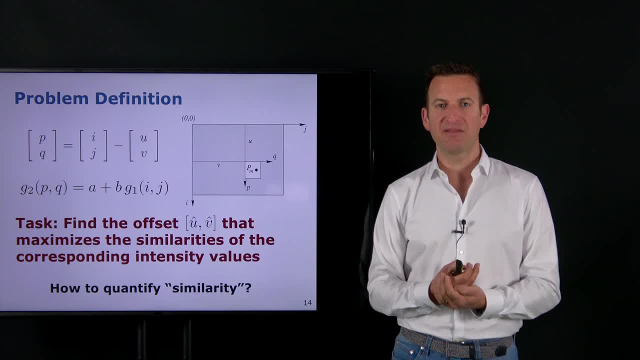 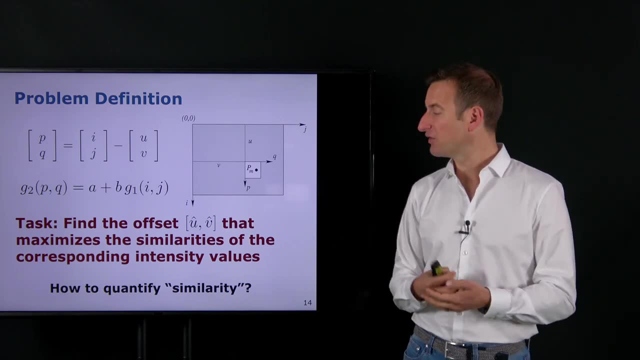 because we can just see if the intensity values are identical. If so, we say yes, it's the same, Otherwise it's not the same. But typically, again, we don't have the same characteristics, and especially that we have a radiometric transformation here. 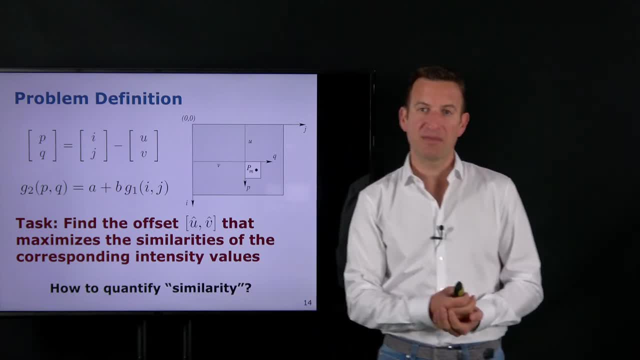 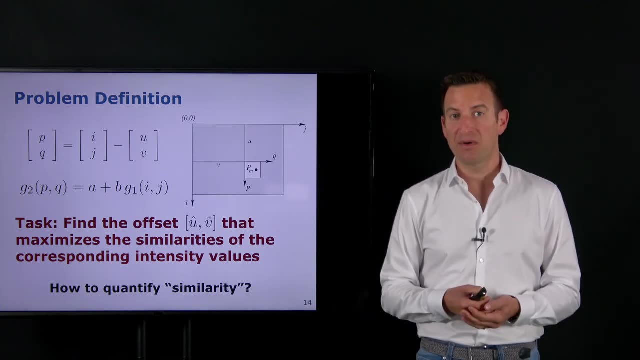 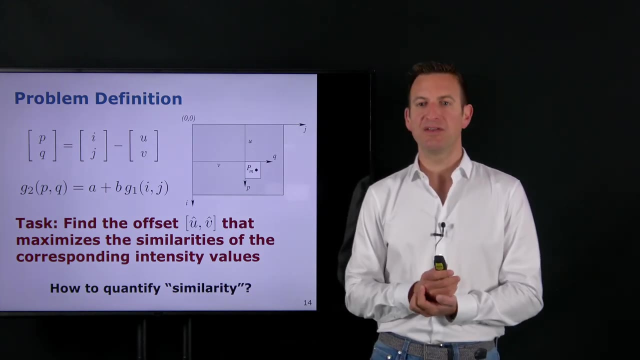 We want to have the similarity under this transformation. So if I'm just changing the intensity value, adding one to every intensity value, I still want to get the same similarity because I want to be invariant under this transformation. Okay, so what are typical ways for computing similarities? 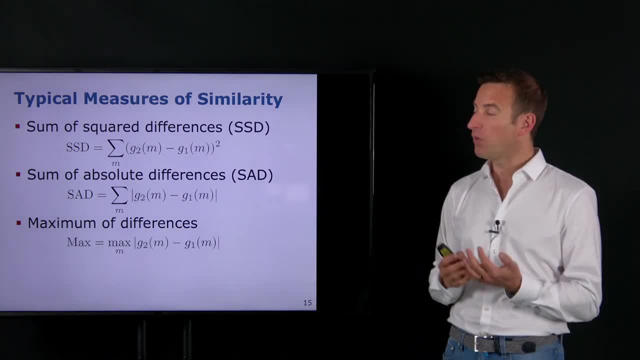 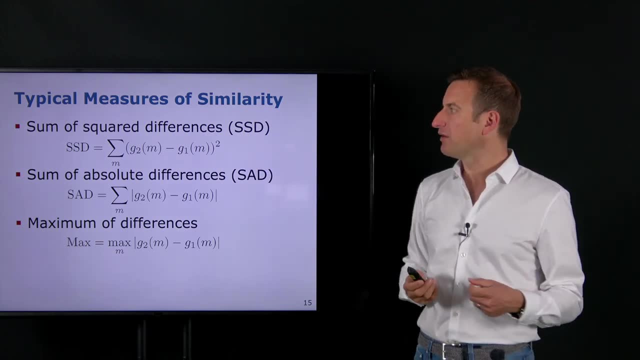 between images, between intensity values, And there is a quite large set of ways you can do this and just let's go through the most standard ones. So, first, sum of squared differences, or SSD. So we take the intensity value in my template. 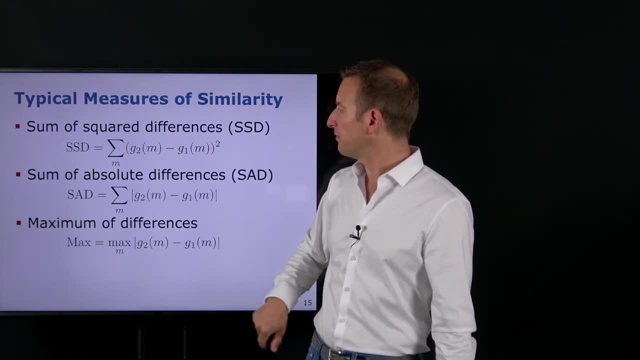 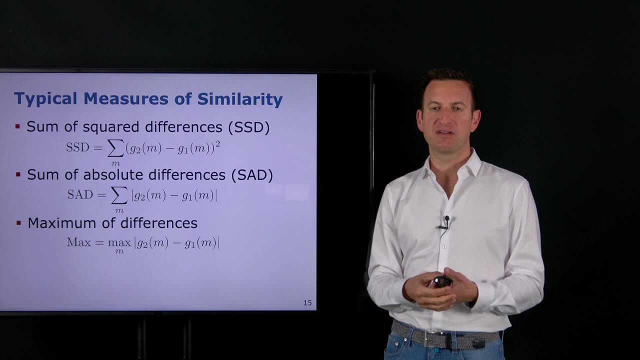 subtract the intensity value in my original image for every single pixel, I compute the difference between them, I square them and I add all of them up, So basically the sum of the squared difference in intensity values. So if one intensity value is 100, 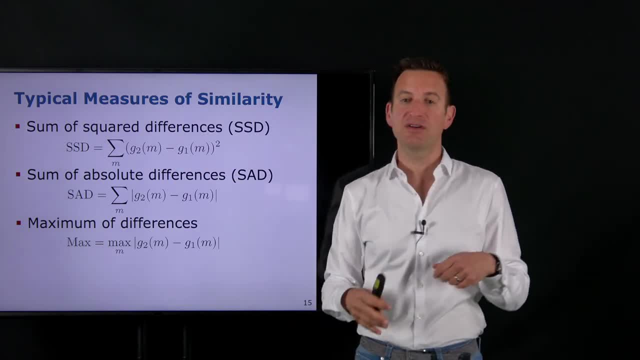 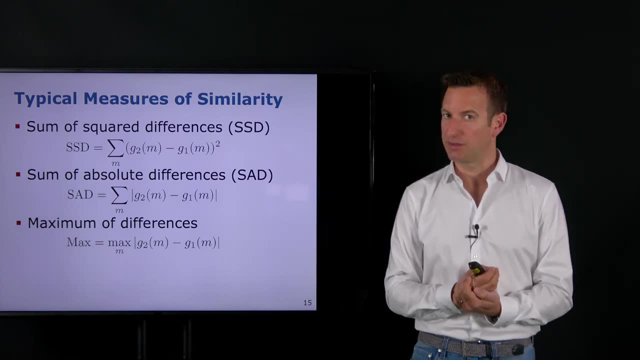 and the other one is 200, then it's kind of 100 minus 200 squared: 100 squared equals 10,000 for one pixel, and then I'm actually summing up all those values And that's it what my sum of squared differences is. 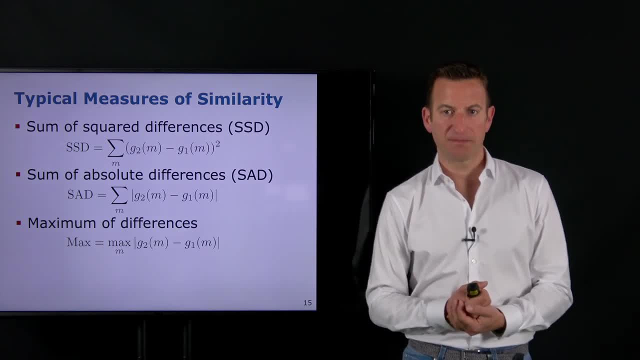 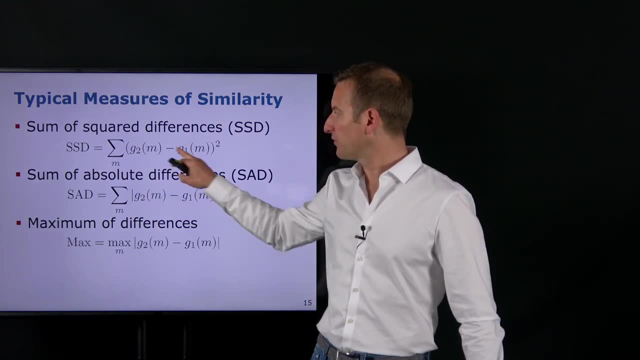 The smaller the sum of squared difference, the more similar the images are. Maybe I don't want to take the sum of squared into account, but the absolute differences, So I'm basically just subtracting those two. Let's take the absolute value. 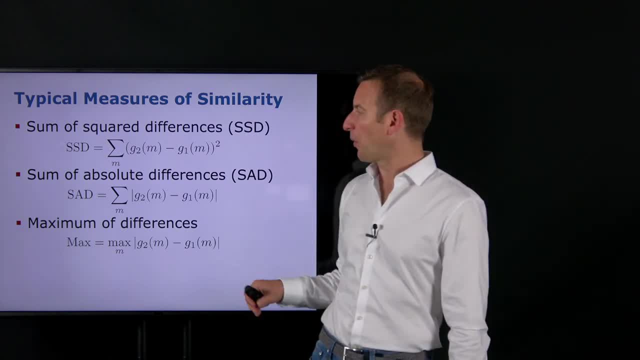 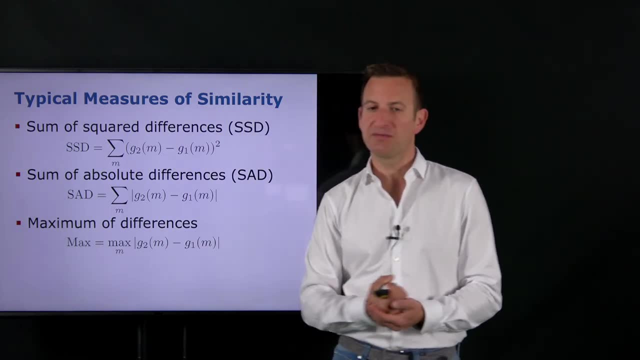 So if the value is negative, I'm flipping it to the positive side, but I'm not squaring. It's also called SAD. Or I'm taking into account the maximum difference, just saying what the maximum difference in intensity value in that local region where the images overlap. 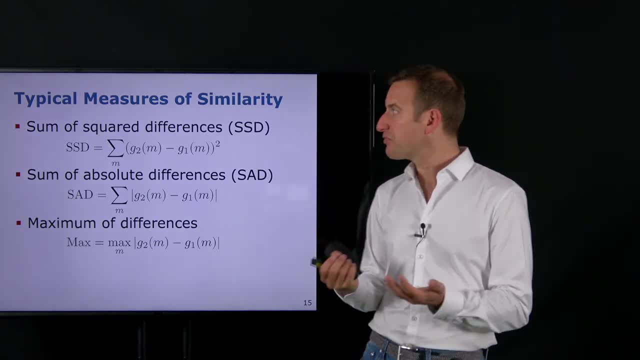 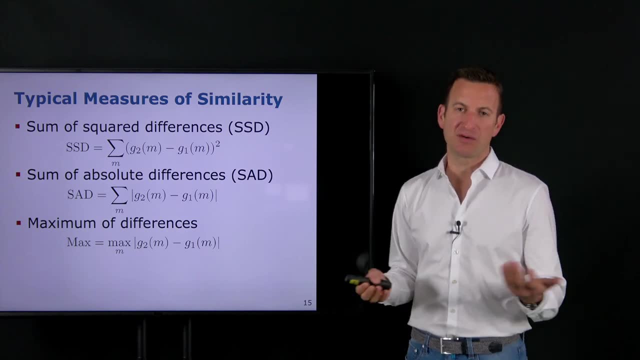 I'm just looking for the maximum difference of those intensity values. So there are three different ways how I can actually do that. These are standard ways for comparing images with each other or images with templates, But the problem with all those techniques is that they're actually not invariant. 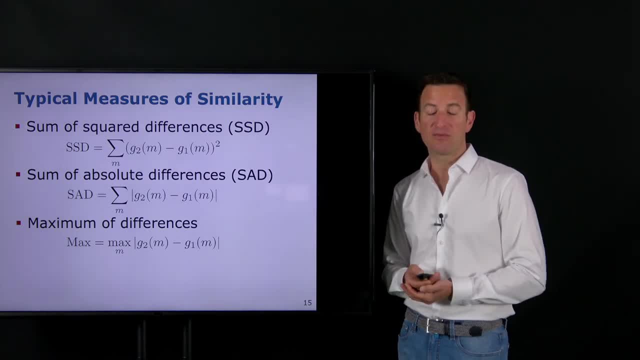 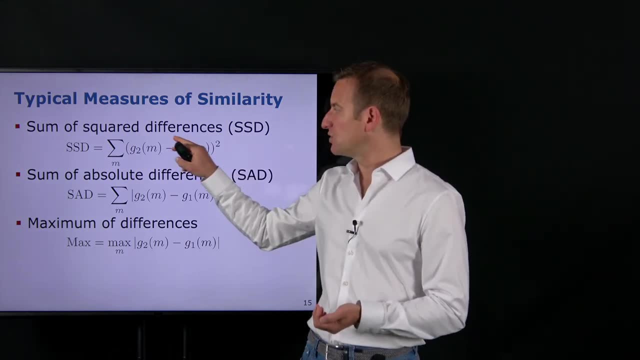 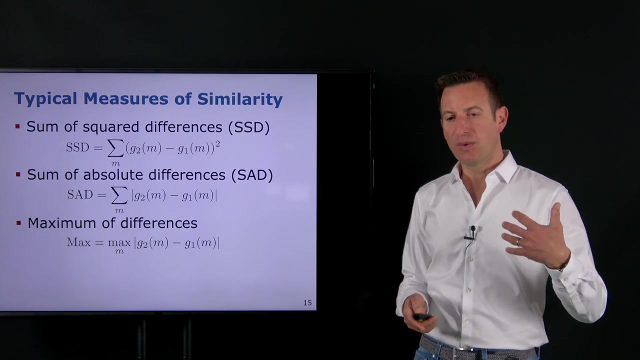 under the radiometric transformation that I've introduced before. Mainly, if I'm changing the brightness of, let's say, the image and not the template, this will actually lead to a different cost. So one image where I'm just kind of changing: 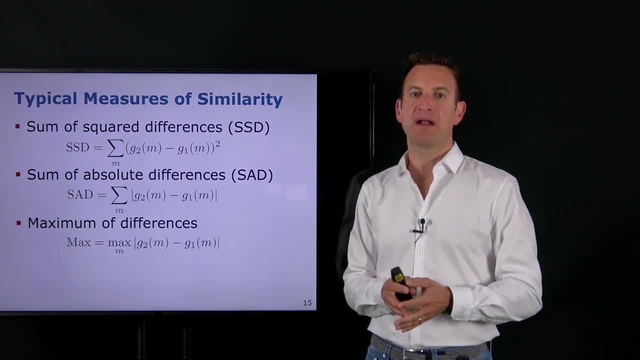 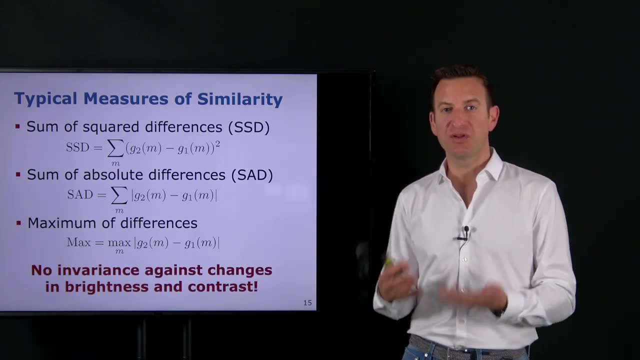 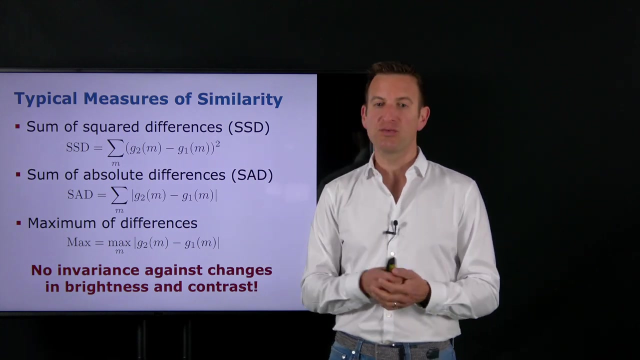 making the image brighter, making one image brighter and comparing those images will actually give me a different measure of similarity, And that's something that I would like to avoid, because I explicitly want to be invariant under this radiometric transformation that I defined before. So all these three measures do not provide me. 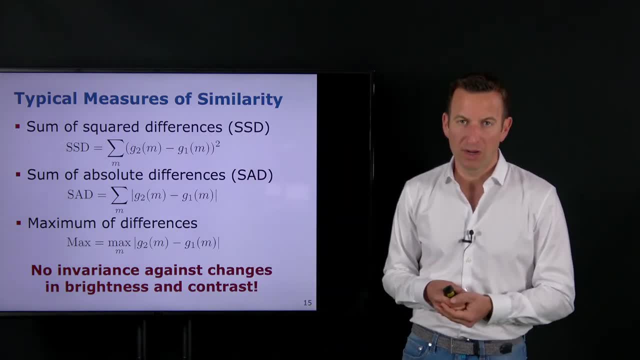 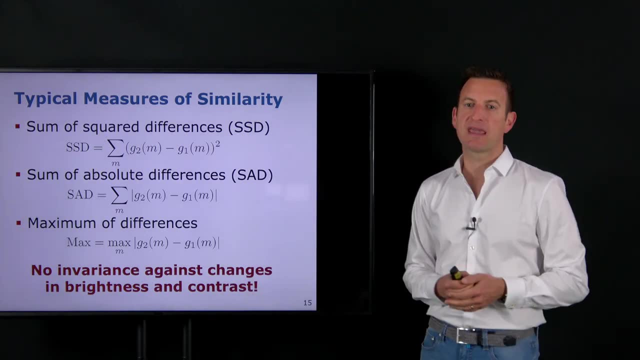 an invariance against changes in the brightness or contrast of one of the images, And that's something that I would like to have. Therefore, we are in cross-correlation, not taking into account those standard measures over here, but we go to a different, take a different approach. 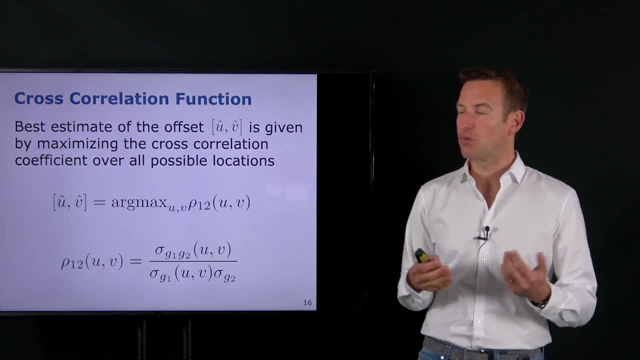 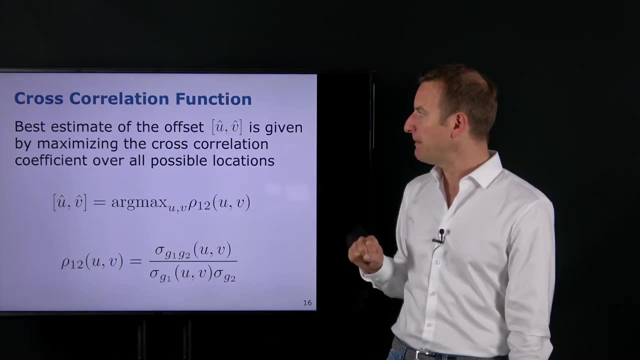 and let's take the cross-correlation function into account. This is what it gives this approach its name. So what I want to do is I want to again find the best offset by maximizing the cross-correlation coefficient over all possible location. 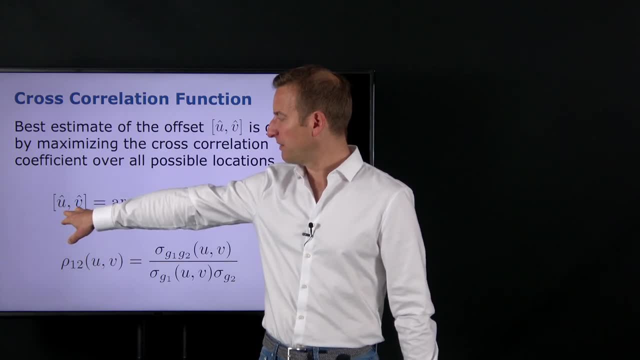 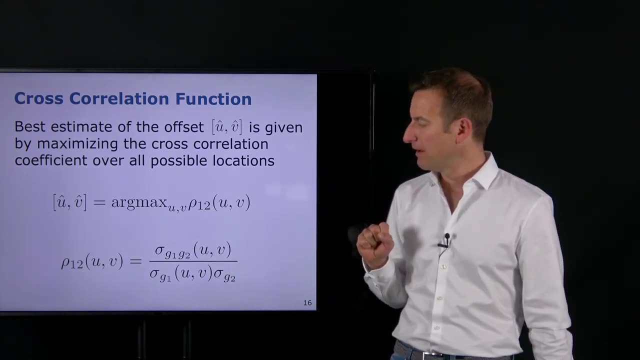 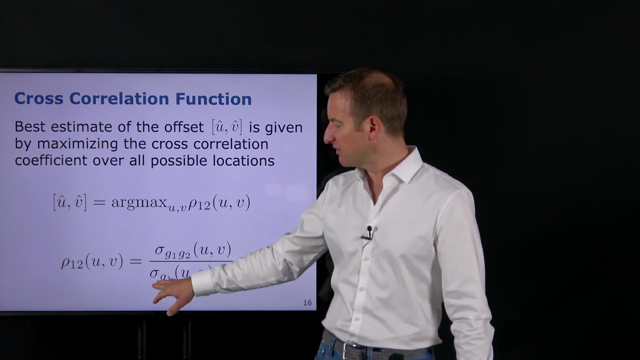 So I'm basically saying I'm returning as the best possible estimate those UV parameters that maximize this function over here. And this function, as you can see, has something to do with variances or standard deviations between the two images. And I want to go now a little bit more. 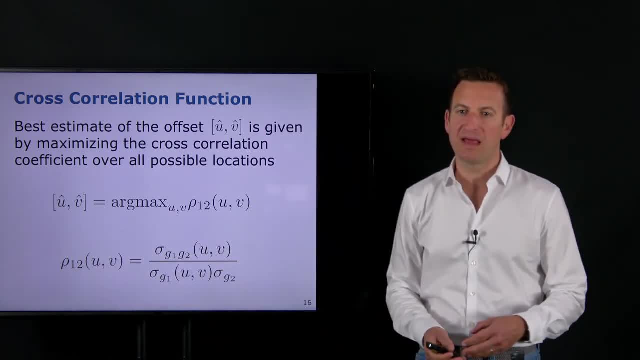 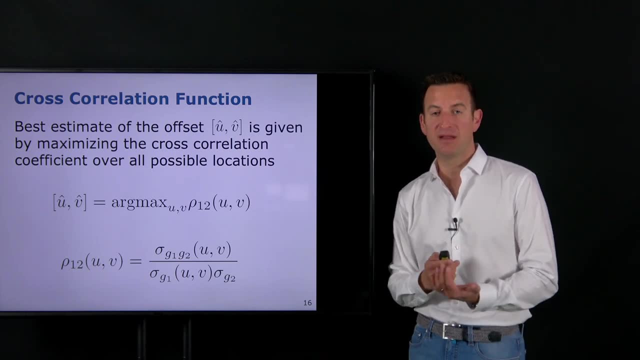 into the details in the next slide and explain what that normalized cross-correlation actually does and what the individual values here are. And, as you see, the advantage of this technique is of using this measure is that it's invariant under this radiometric transformation. 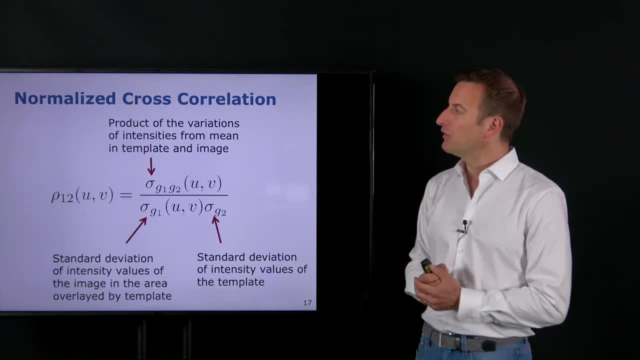 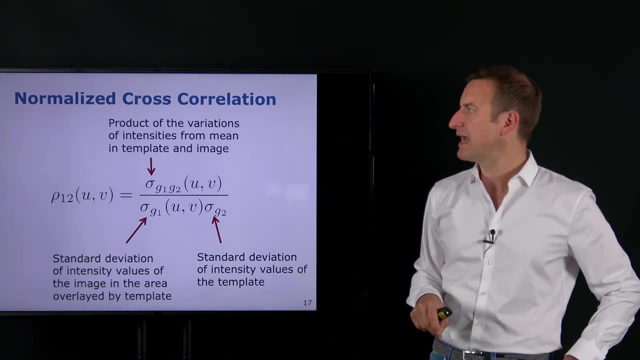 that I was describing before. Okay, so let's dive a little bit into the details and see what actually happens here. So the first part is the product of the variations of intensity values from the mean in the template image as well as in my original image. 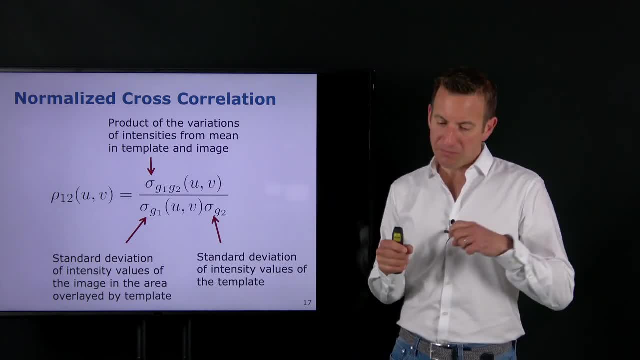 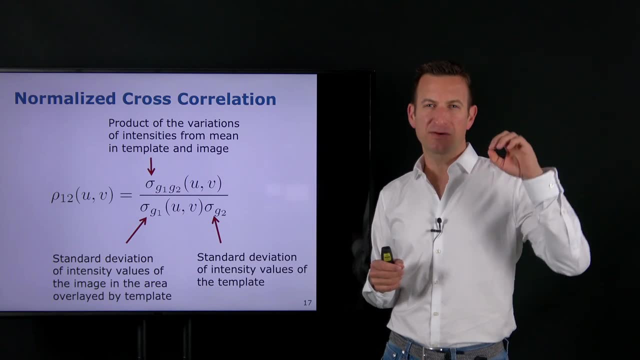 So I'm basically looking in kind of how far do the individual intensity values actually differ from its mean intensity value? So this means, for example, if I shift the mean in one of those images, but I'm only looking to the variations of the intensity values. 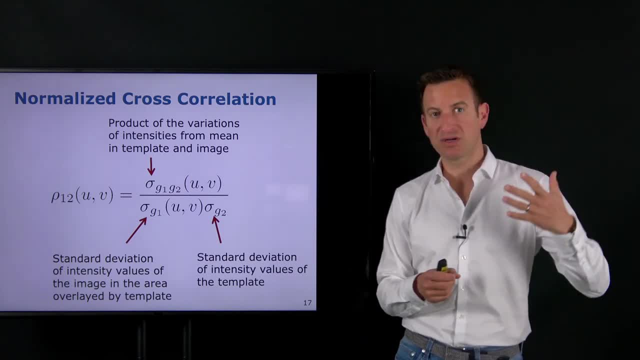 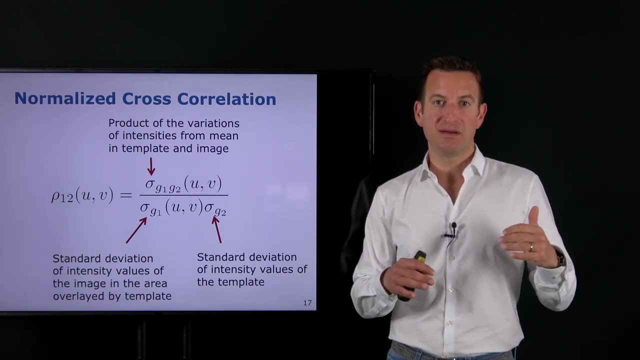 this will actually give me the same result. All right, if I take one image and take my intensity values and I add, let's say, 10 to all intensity values, then the mean is higher by an absolute value of 10, but if I'm just looking into the variations, 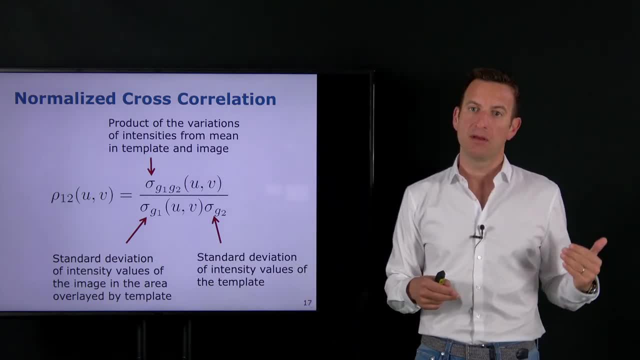 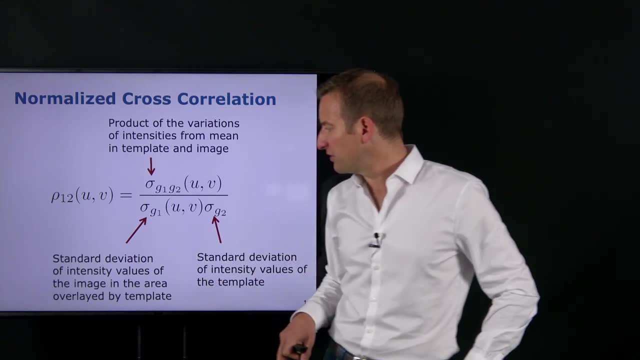 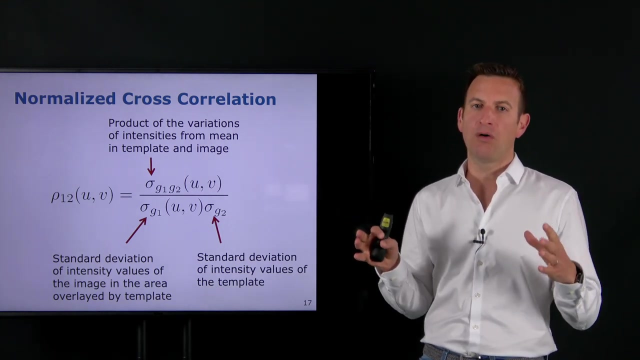 of intensity values from that mean in both images, then I'm actually invariant under that. Then I have down here the standard deviation of the intensity values in my image, in the original image but not computed of the whole image, only taking those into account. 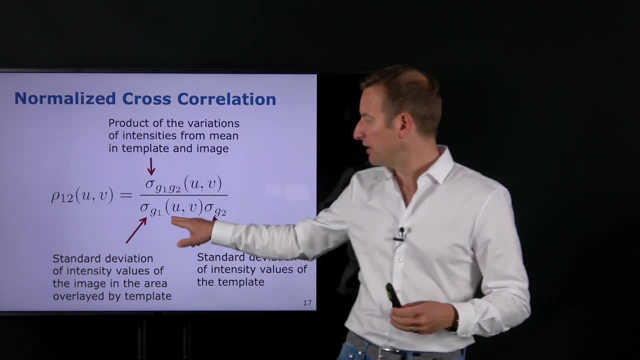 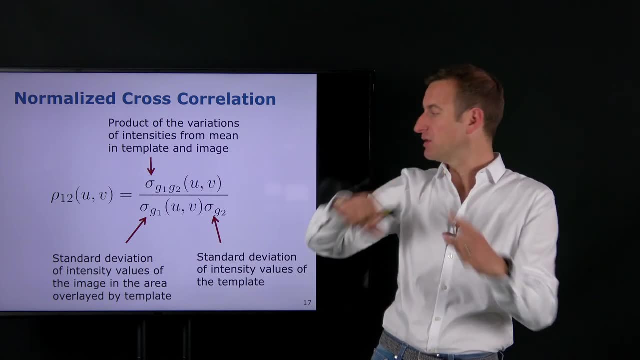 which are in the overlapping area of the template in my image, And therefore here the shift parameters matter, because I'm basically taking the size of the small image, overlying it with a large image, where 0, 0 will be at that location. 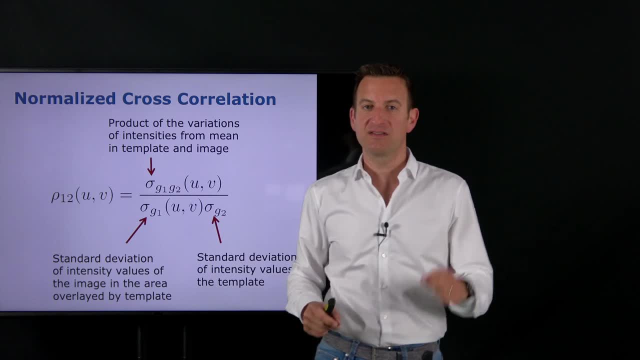 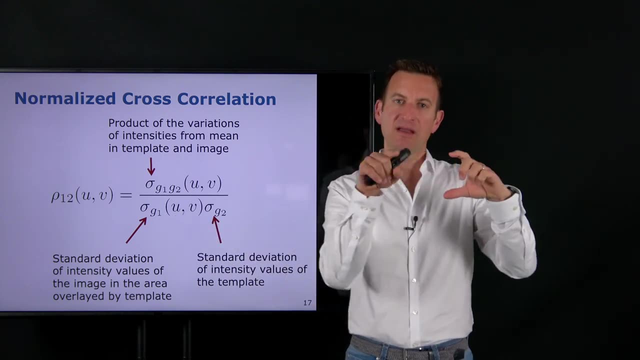 and then only computing the standard deviation of intensity values in that local area. So I'm taking the size of the template, overlying it with my image at my position where I want to evaluate it and then only compute the standard deviation in that local area. 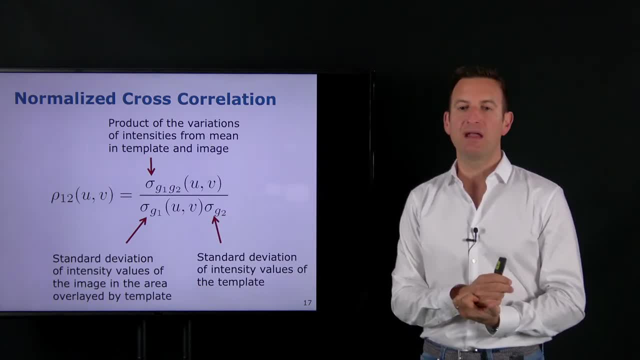 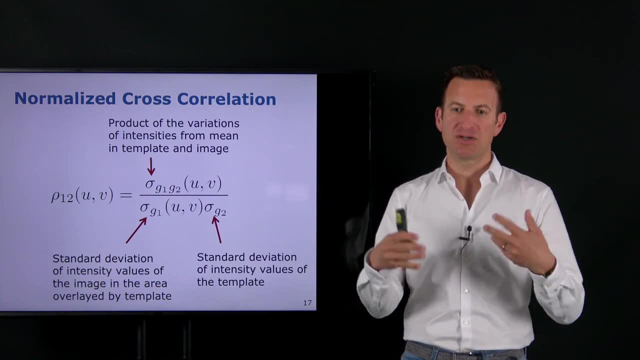 And the second one here is free of the parameter u and v because this is just the standard deviation in my template and no matter whether where it is located in the overall image, these are the same intensity values. Therefore, I only need to compute that once. 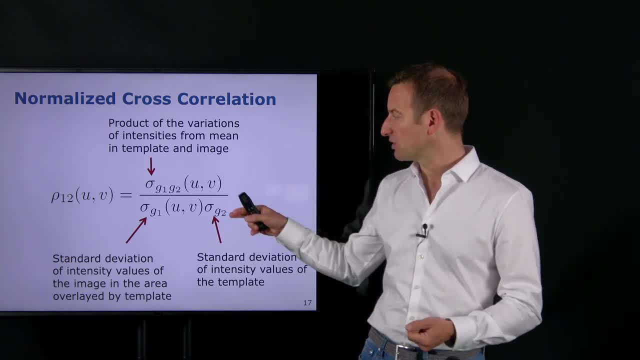 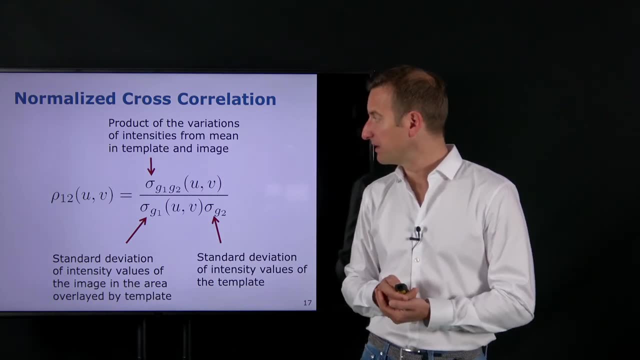 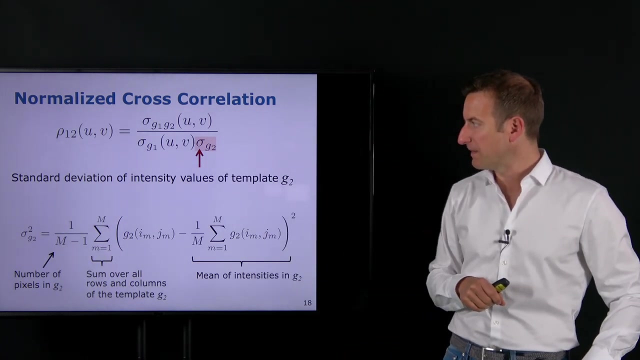 and this parameter is independent of the actual location which I'm looking into, because it only depends on my template. Okay, so how do I compute those individual terms? So this one is the standard deviation of intensity values of my template G2.. So how do I compute this? 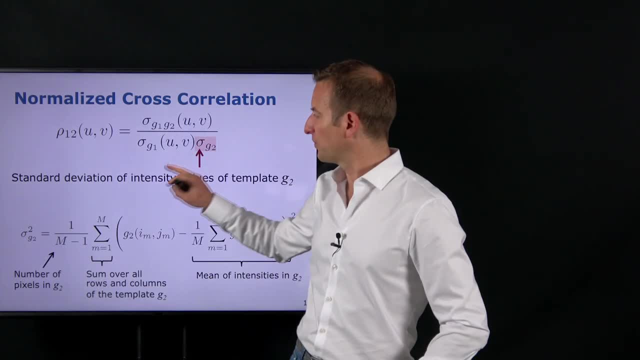 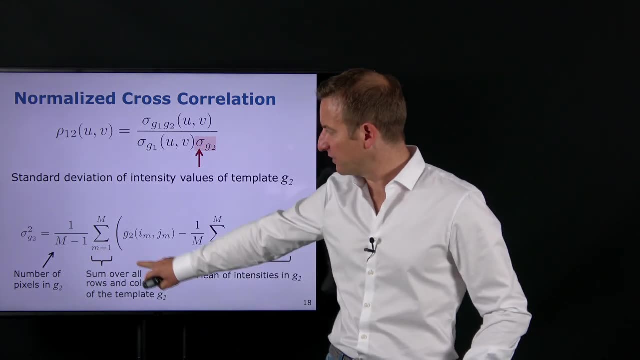 So the variance, this is kind of the square root of this. so the standard deviation is the square root of the variance. I'm having a formula for the variance in here. So this is my normalizing term by the number of elements I'm taking into account, minus 1.. 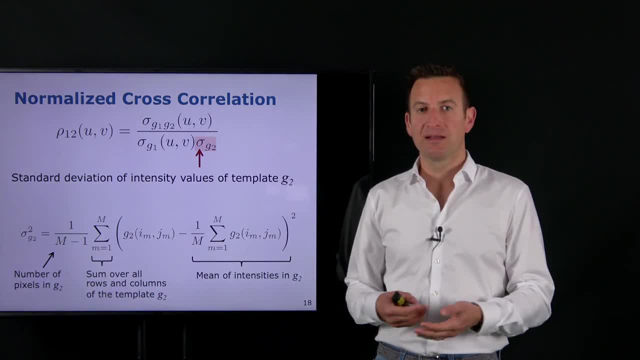 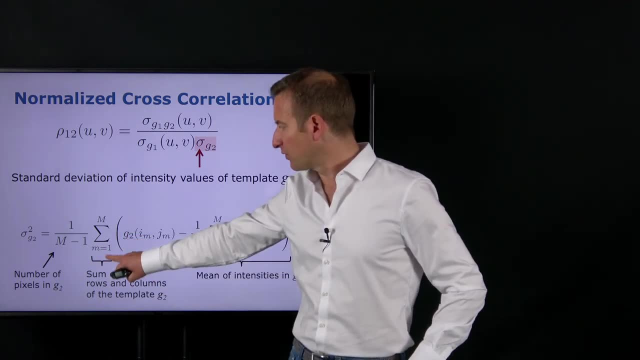 So these are the number of pixels in G2.. So lower-upper case m tells me how many pixels do I have in my template? What's the size of my template? Then I'm summing over all elements of all pixels in that template. 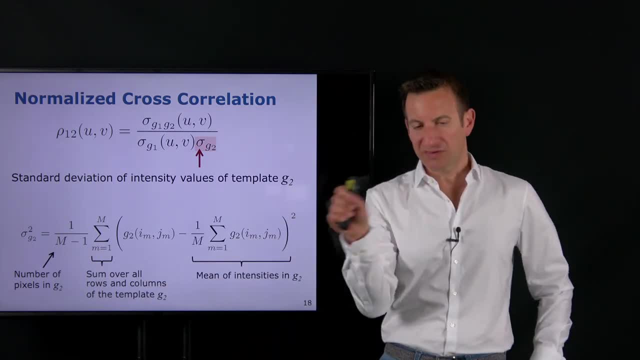 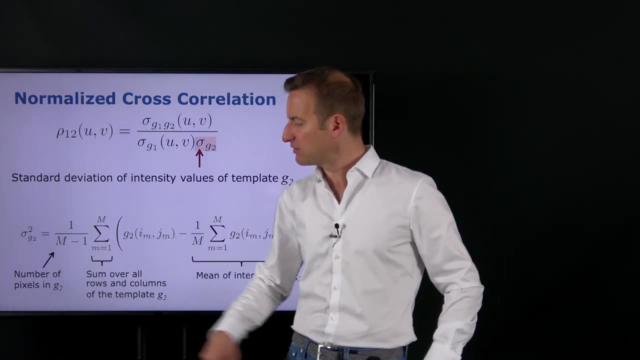 and summing over all rows and columns, so assuming that I can just have one sum going over them, not splitting it up into two different sums just to make the notation more convenient. So this basically means I'm iterating over all pixels in my template. 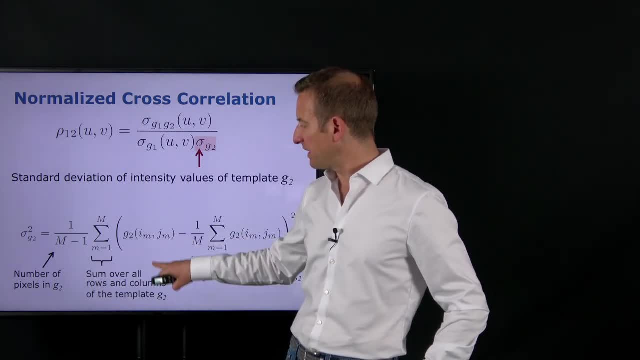 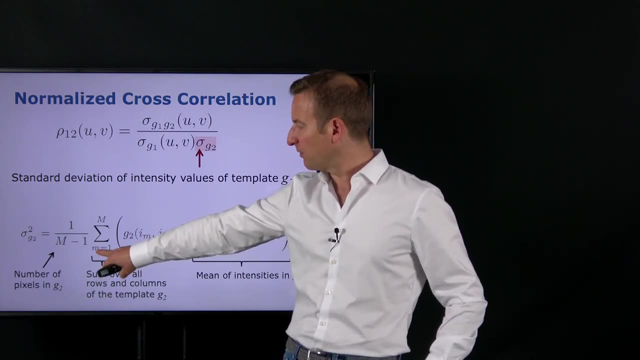 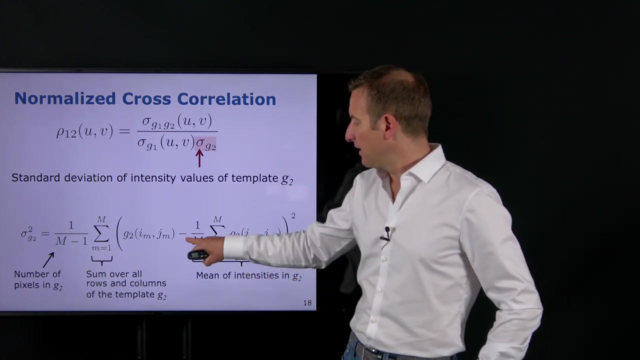 And then I'm taking the actual intensity value of the template and so this: i subscript m and j. subscript m means I'm basically mapping this index from 1 to m, basically to the corresponding x and y. So this is my values in that template. 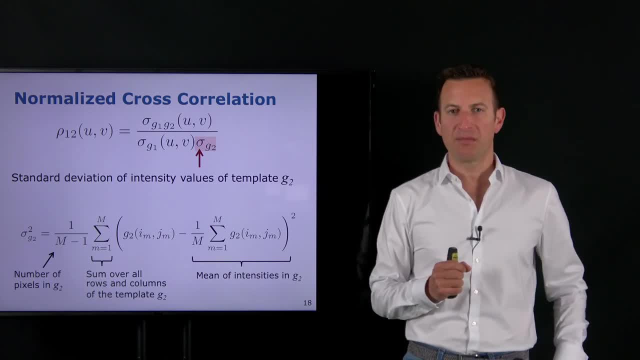 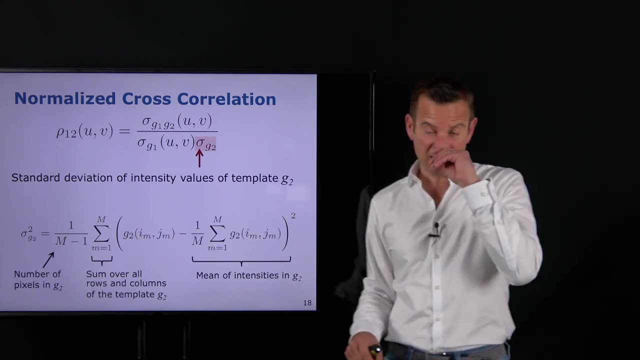 And what I'm subtracting from this is the mean intensity value over my template. So I'm computing the mean intensity value of my template, Then I'm subtracting that one from the actual intensity value. So this tells me here the deviations of the intensity values. 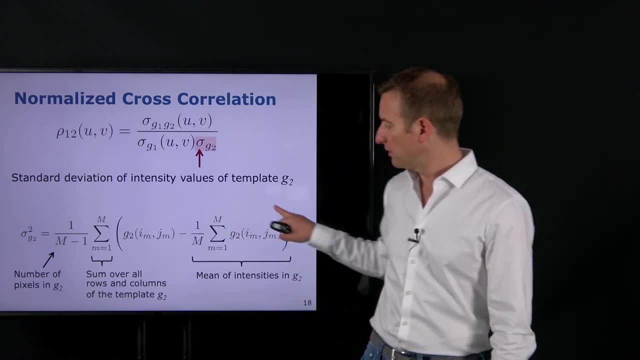 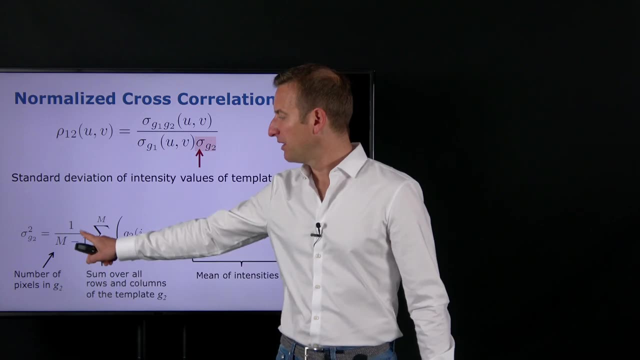 in the template from the mean. I'm squaring that. So I'm basically computing the squared difference for every single pixel, how far it is away from the mean, And then I sum them up and divide by the number of pixels minus 1.. 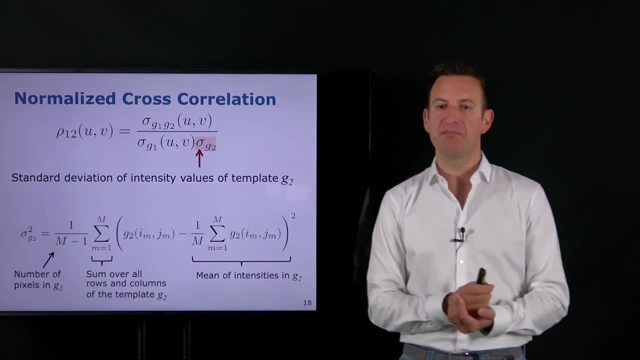 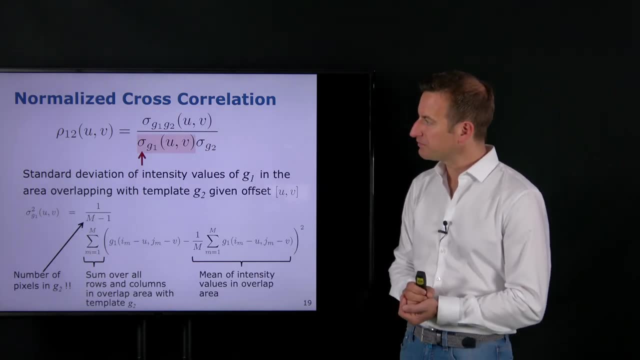 So I'm computing the variance and then I take the square root of that and this gives me my value over here. Okay, so that was the first term. Now let's go to this second term. down here. It's basically the same. 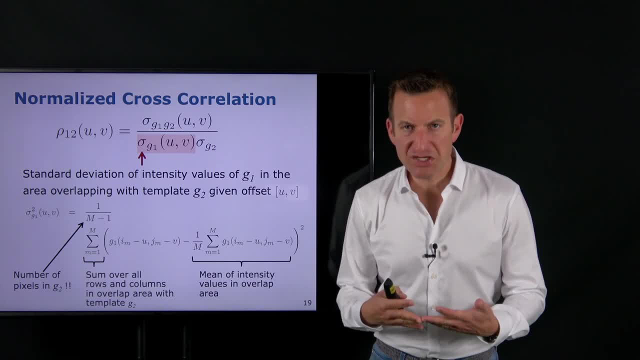 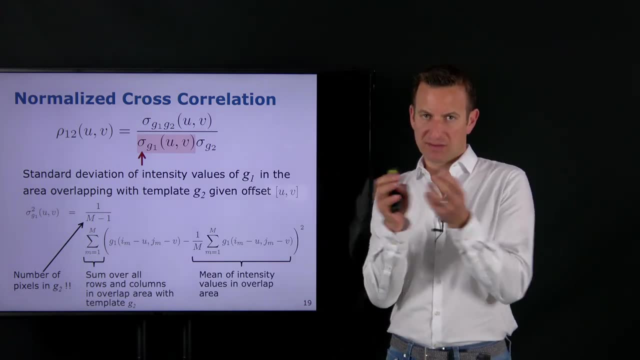 except that I'm performing the operation now in my original image, in my image of G1, and only in the area that overlaps with G2, because this is a comparison that I want to do. I'm overlapping two templates or two local regions. 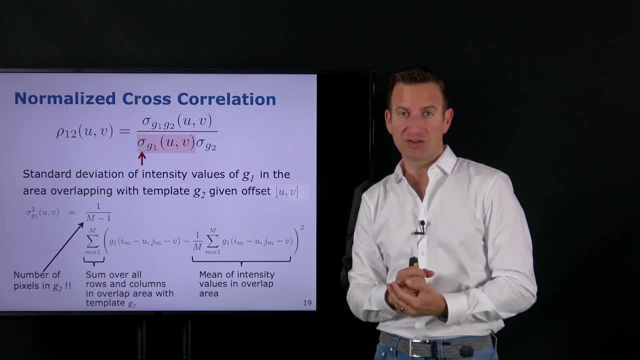 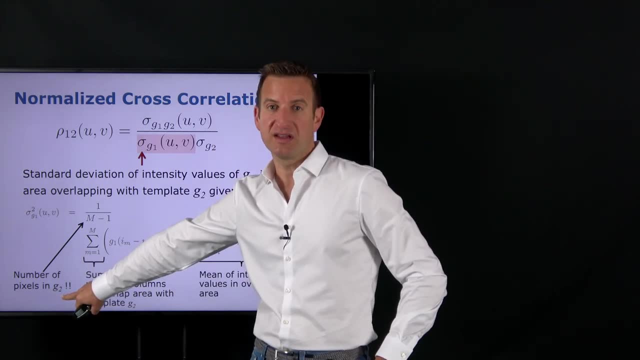 and we'll say how similar are those local regions. What happens outside is not interesting to me at that moment, So I'm again summing over all pixels in G2, so not G1,. G2 is important. It's not a mistake in here, G2.. 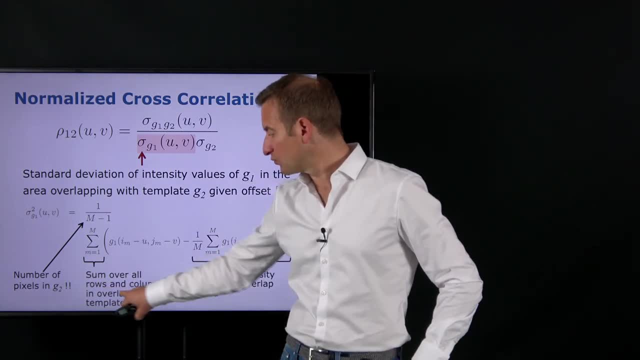 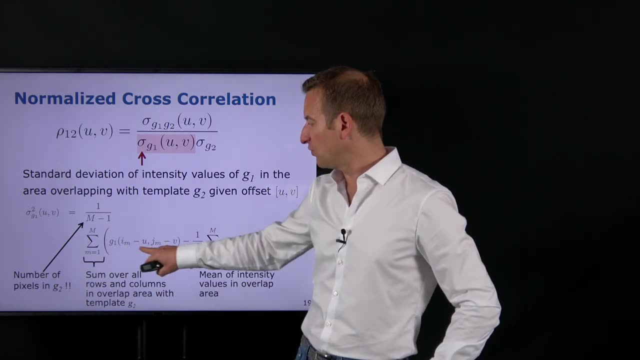 It's just the size of the template. And then I'm iterating over all rows and columns in that template and saying, okay, what is this value? using the same index that I used before and now subtracting from here the offset. So I'm basically saying: 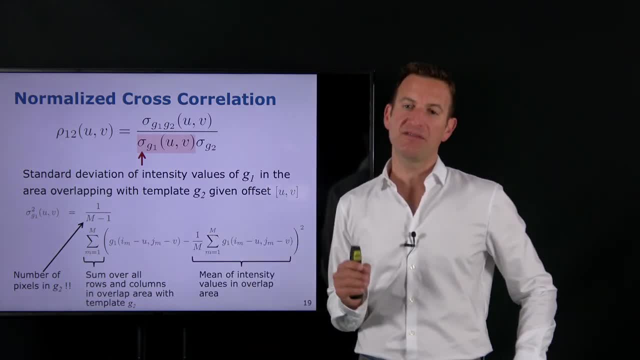 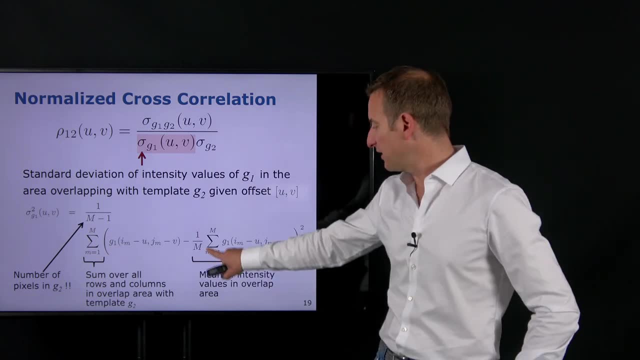 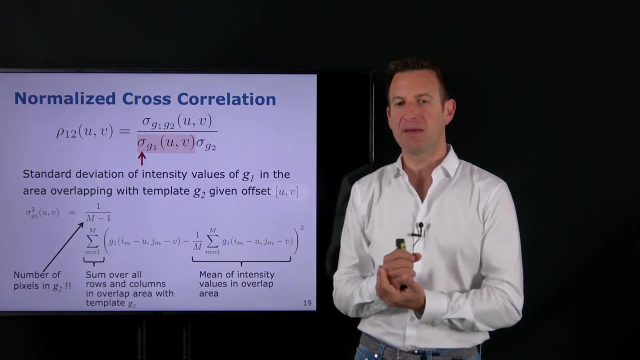 so what I'm doing here? I'm taking the intensity values in my in one image and taking the offset appropriately into account And then subtracting the mean intensity value of the image, but only located in this overlapping area of my template. 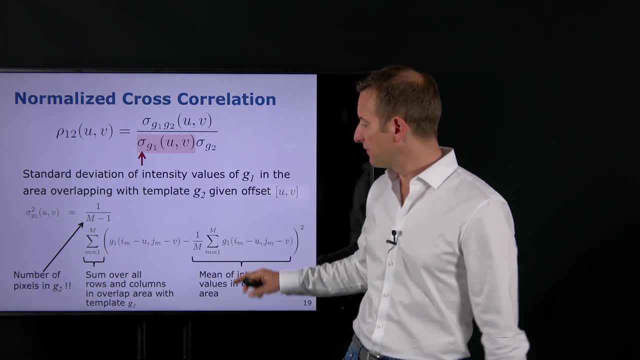 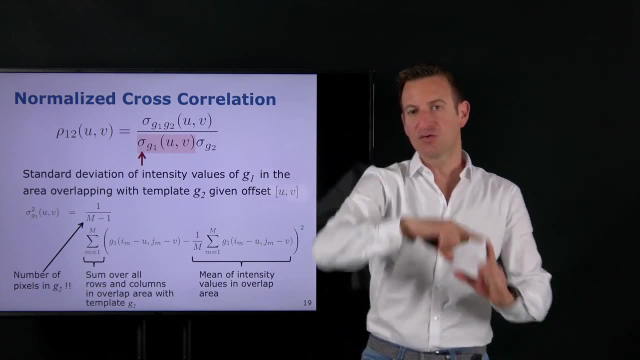 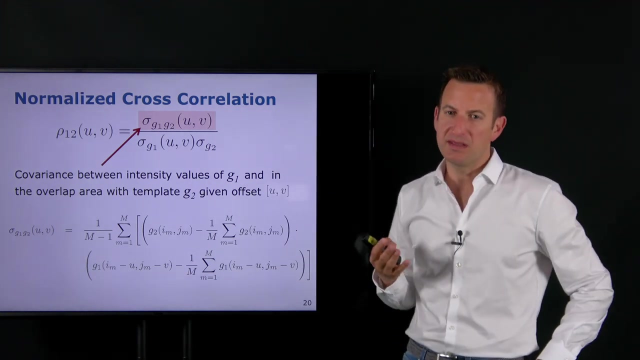 And the rest is the same. The only difference is here: this computation depends on the index UV, because I'm basically only doing this computation in that small region. And then this part of the equation is the covariance between the intensity values that I have in my image G1. 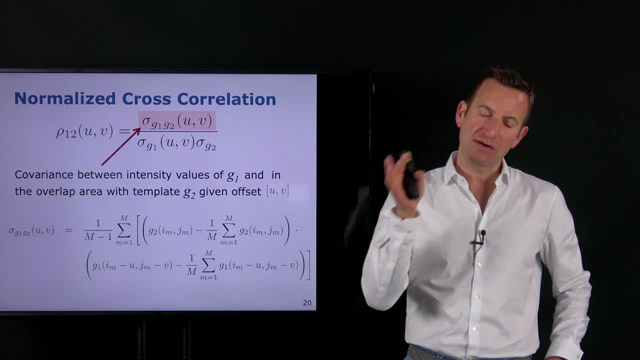 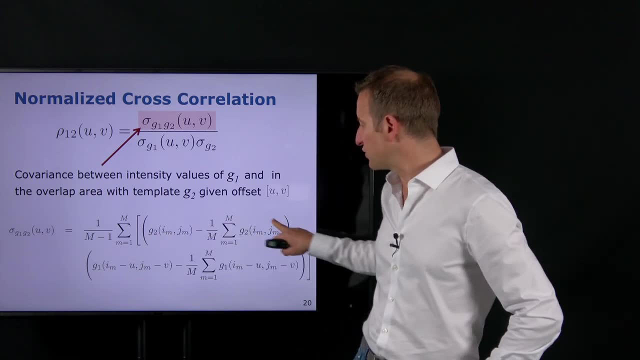 and my in the overlapping area, so in the area that overlaps with my template in G2.. And so I do the computation here, one for the parts of the image that happens in G2 and this the intensity values that happen in G1.. 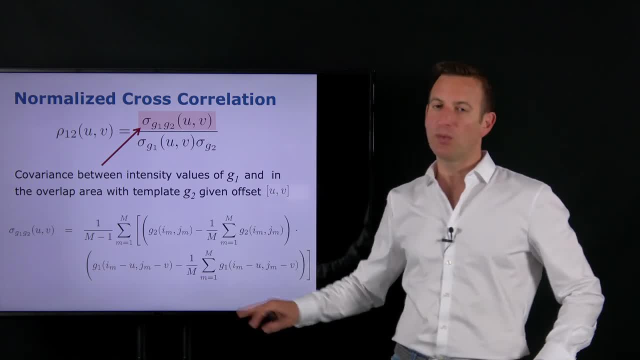 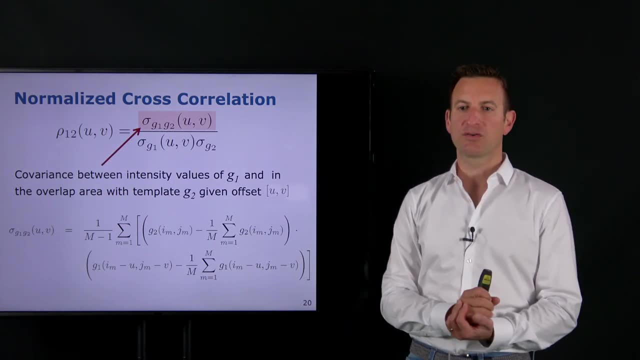 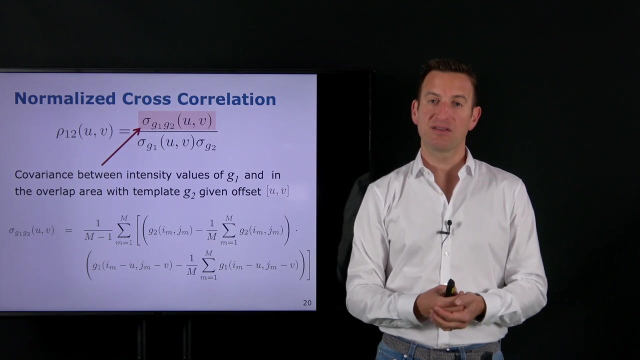 Taking always the mean of G1 and the mean of G2 into account, always in the area of the template. And if I compute this normalized cross-correlation value, that means large values, will tell me: yes, the two images are identical under this measure. 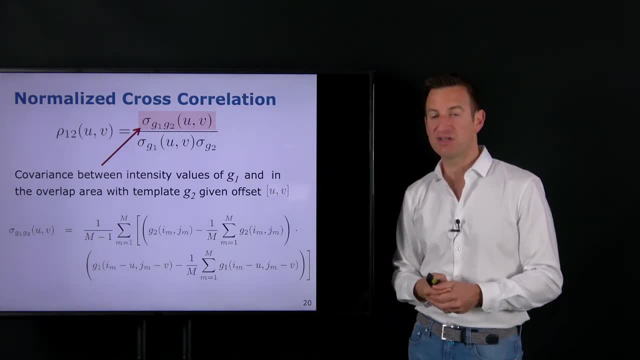 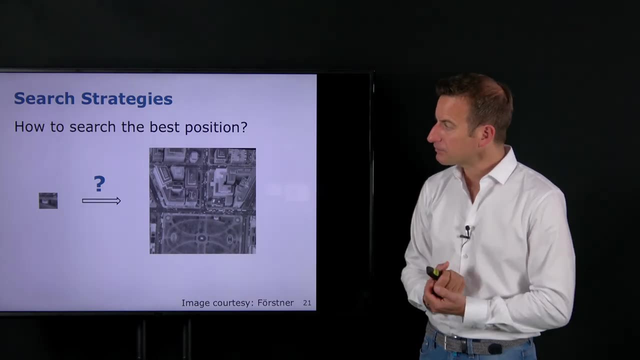 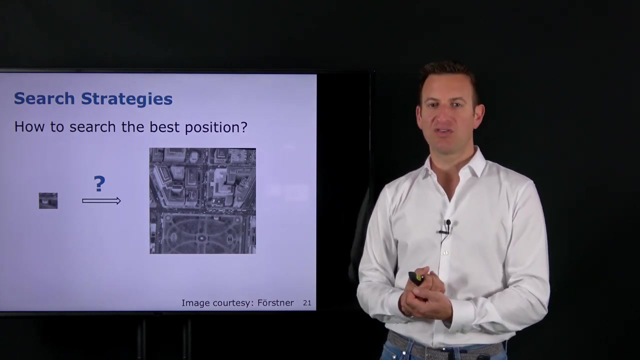 being invariant with respect to translation and shift, And if this is a low value, then this is not the case. Okay, So I now defined what transformation I'm allowing and I told you how I measure similarity now. Now the question is: 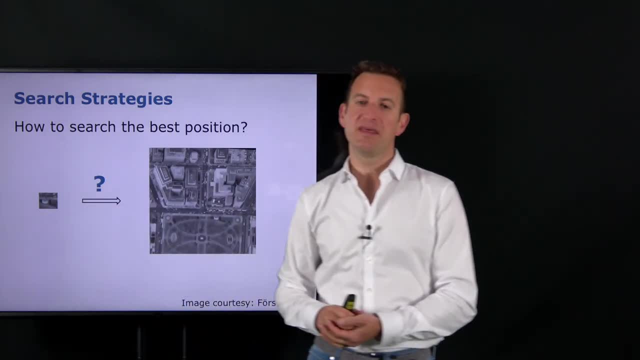 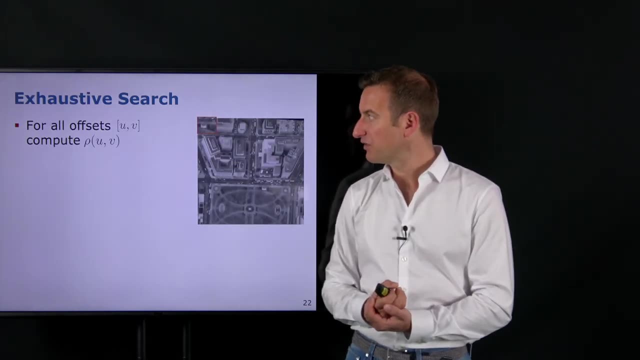 how do I actually find the best position? So how do I determine where that local small template sits in my large image And what I need to do for this? I simply need to compute this measure, this similarity, for all possible offsets. So I say okay. 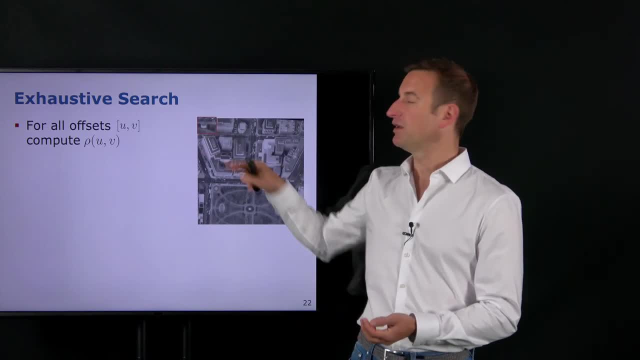 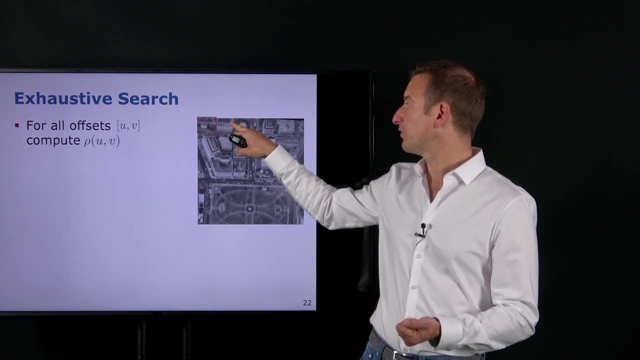 what about offset 0, 0?? That means I'm sitting over here. What about the offset 1, 0? Or 0, 1? Moving 1 here? Or 0, 2? Or 0, 3?? 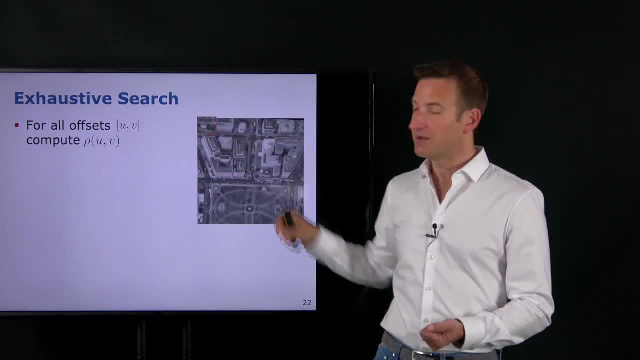 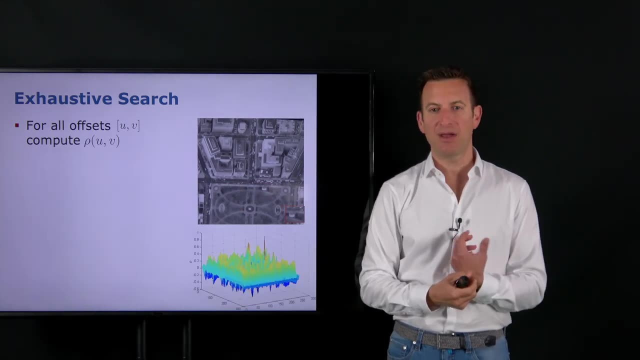 Or 0, 4? And so on and so forth, And then through the individual rows and columns, And I'm basically taking this template and I'm basically sliding it over my image and evaluating that image at all locations. So, as a result of this, 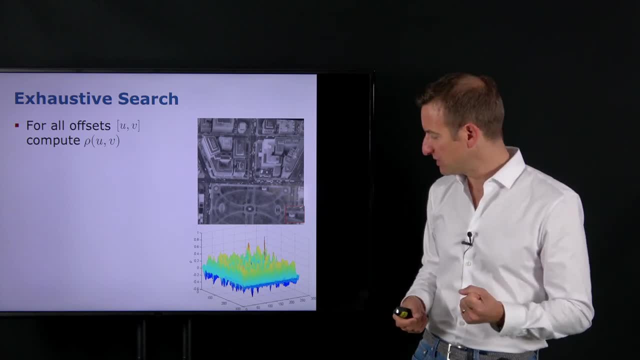 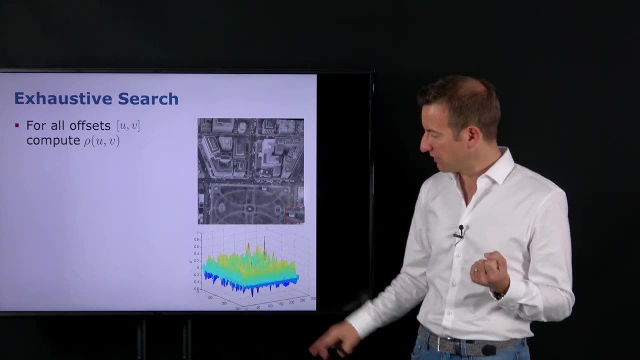 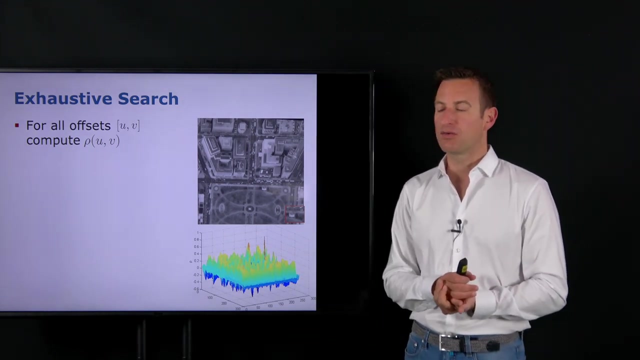 for every possible shift. so which is a u and v coordinate? over here I get one of those normalized cross-correlation values And these I can represent here at kind of this hilly landscape, not very smooth, of cross-correlation values. 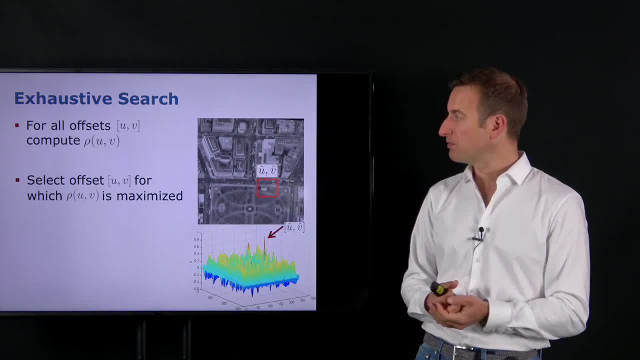 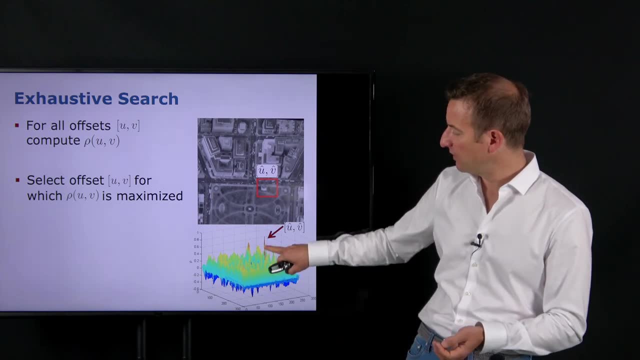 And then I said, okay, I want to take the one which shows the best performance, So where the row value, the normalized cross-correlation value, is maximized. And this is here, at that location where I kind of have this red peak over here. 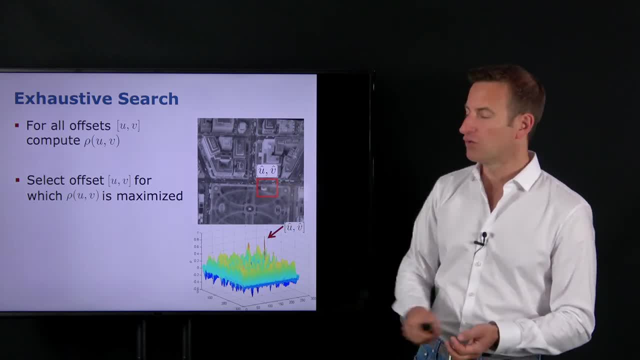 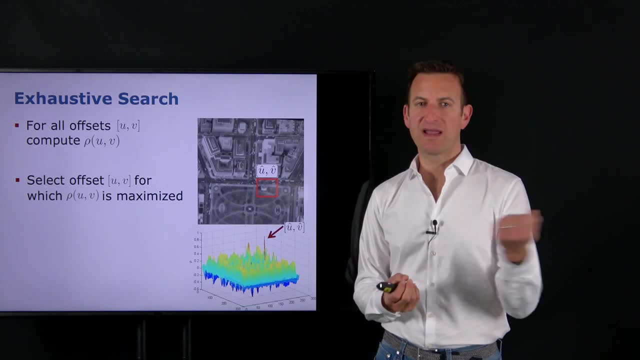 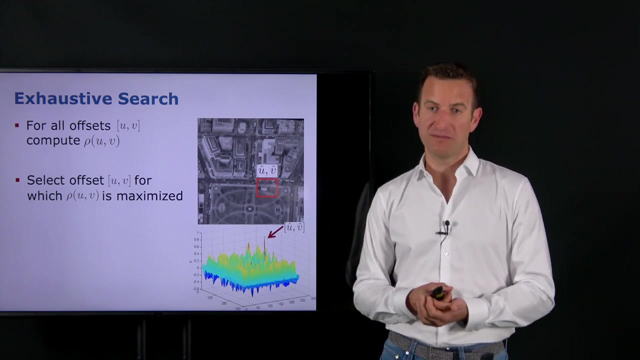 And this exactly corresponds in this example here to the true location where that point actually is. So it's basically an exhaustive search that I'm computing, trying all possible intensity values and see if they would actually fit. What you can see in here is that 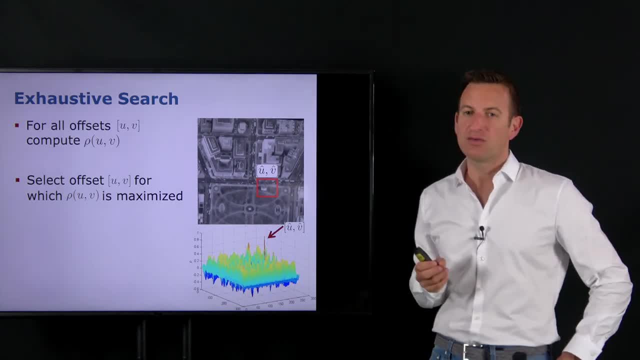 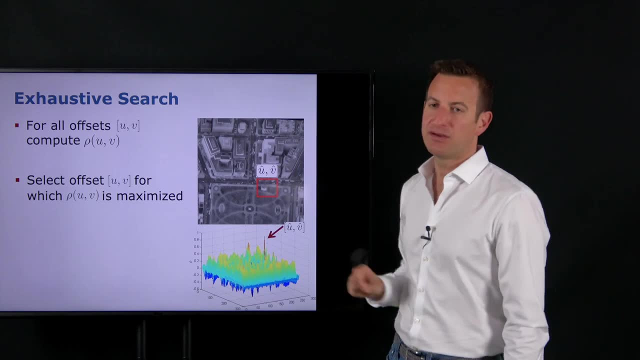 there's also one way how I can increase this approach to taking into account rotations, for example. So the naive approach now to take into account rotations. I'm not just sliding this template over the original image. I may also rotate that template and try all possible rotations. 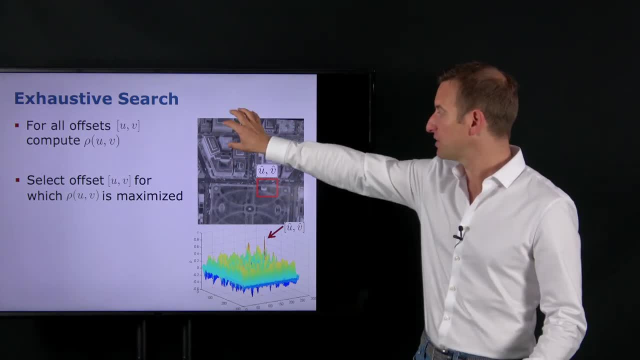 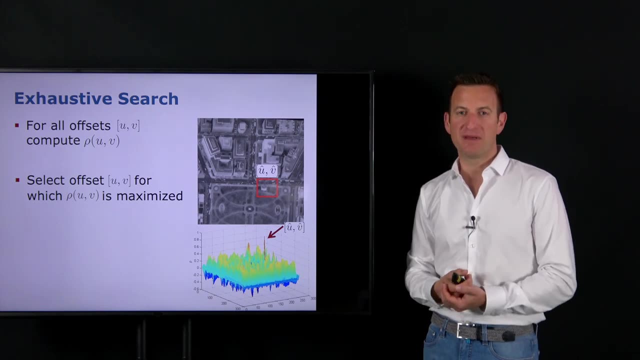 sliding them over the image. And then, of course, for every possible rotation I need to slide over that image, So it gets computationally much more demanding. the more possible parameters for that geometric transformation I'm going to add to that. Therefore, we are sticking here. 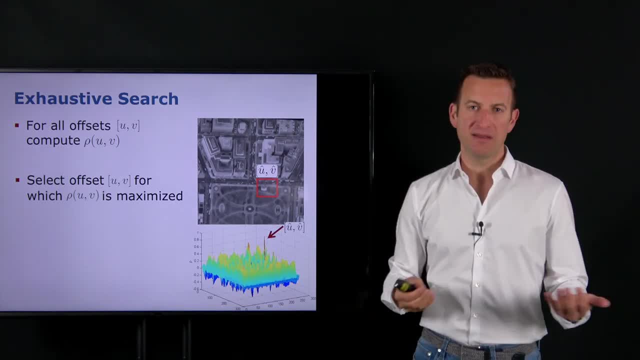 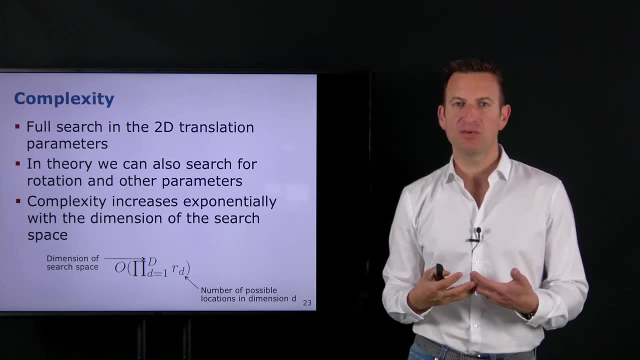 just to translations, so shifts in the delta x, delta y pixel coordinate. So in terms of the complexity of this approach, so we're basically doing an exhaustive search or a full search in the space of 2D translation parameters. So I'm basically trying out. 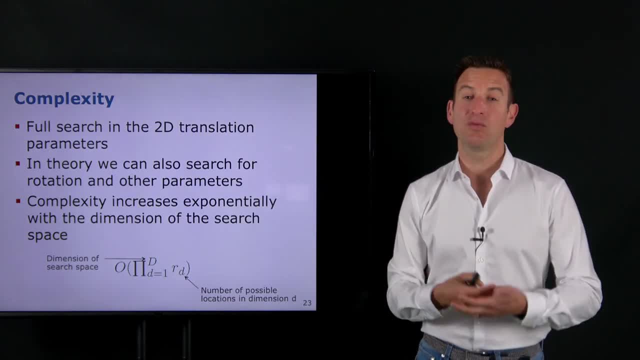 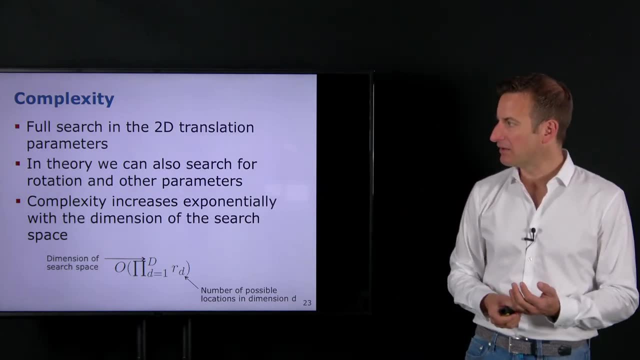 every possible location. Of course, I need to do not do all possible locations, all possible locations where the template and the images actually do overlap And, as I said, we could also look for rotations or other parameters, but that increases the complexity. 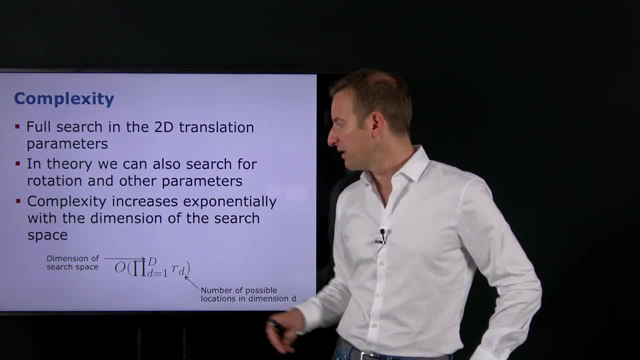 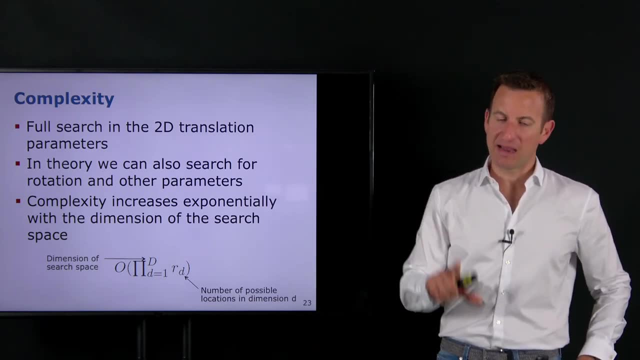 And the complexity actually increases with the dimensionality of that search space. So the number of parameters I need to test for the shift in x times, the shift in y times, the shift in y times, the number of rotations times the number of whatever shear parameters. 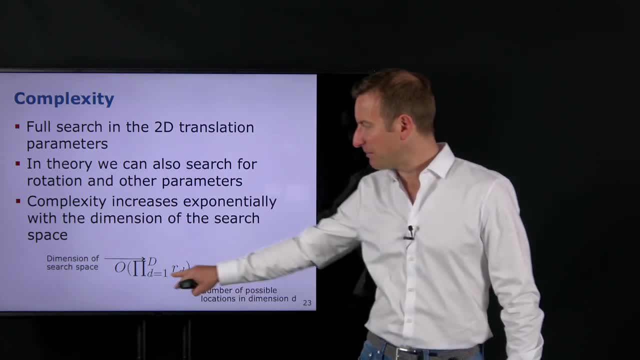 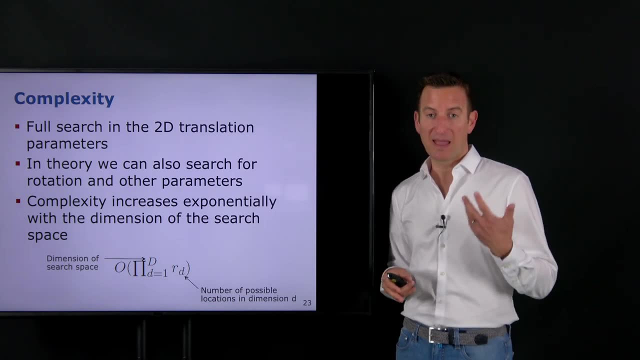 or scale parameters I want to take into account. This all adds up and I need to multiply those values, So the complexity grows very, very quickly And therefore I want to reduce the number of dimensions or keep the number of dimensions I need to take into account. 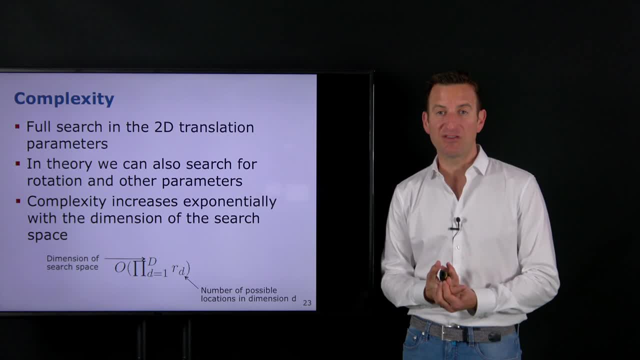 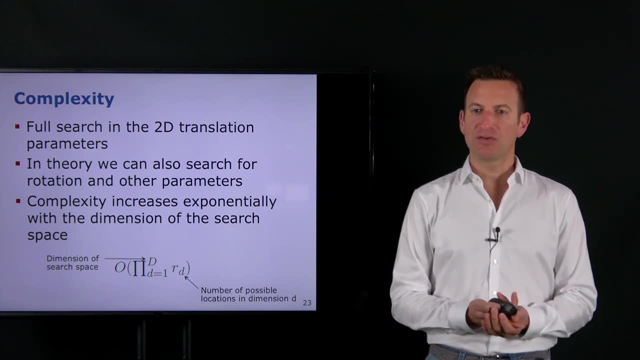 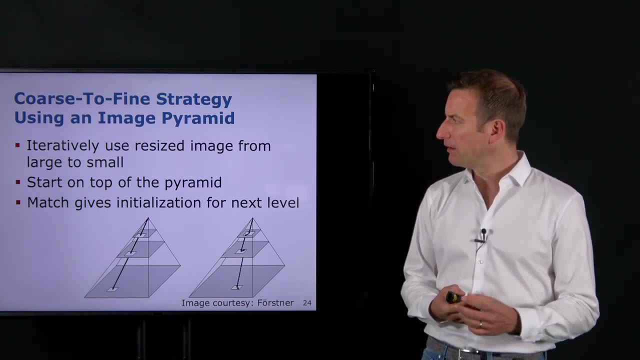 in order to have not a dramatically increasing complexity, being unable to compute the results later on. A few notes about how we do that in practice. One is to be more robust and the other one to also be relatively fast. doing this, We are not using 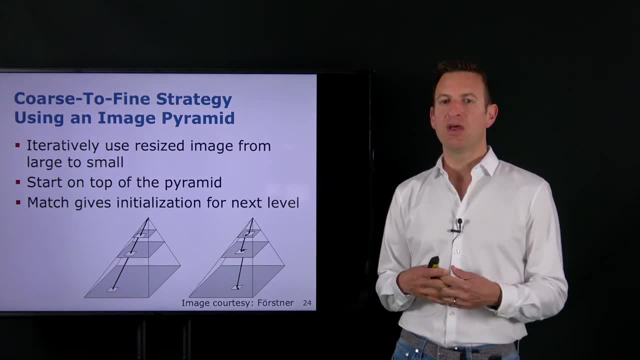 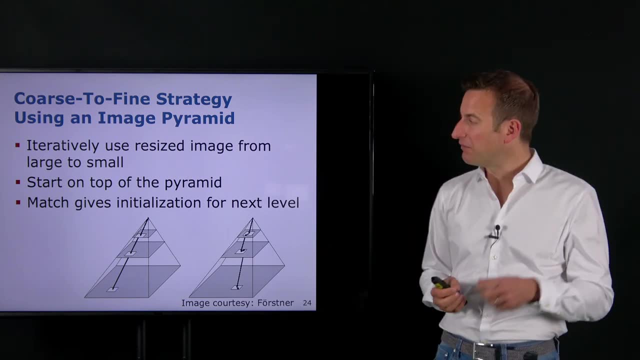 the original image immediately. So what we are typically doing is we are using downscaled versions of the image to first localize the patch roughly and then perform a fine-based analysis, And this we can do using an image parameter. Remember image parameters, something that we discussed. 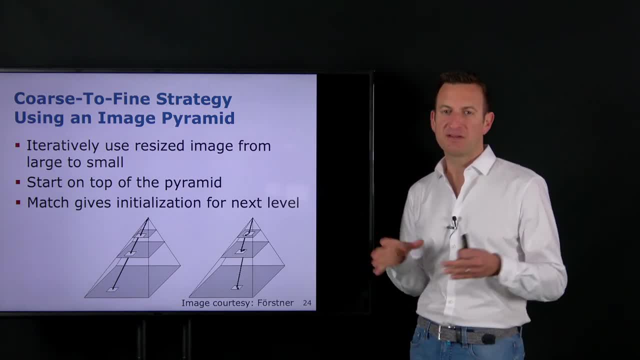 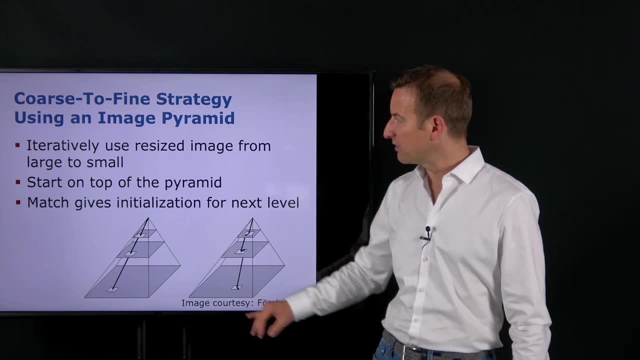 in the chapter of geometric transformations. These are differently scaled versions of the image, For example, halving the size of the image from one level of the pyramid to the next level of the pyramid. And one way I could do this? I could simply. 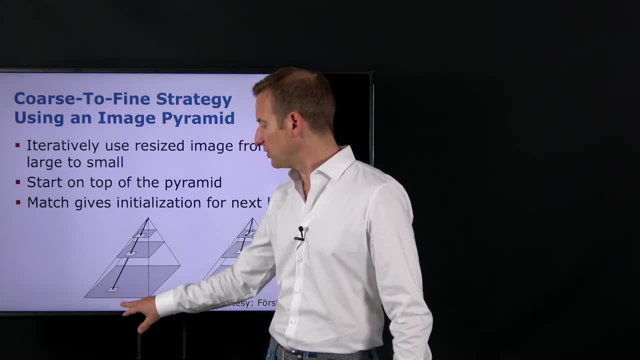 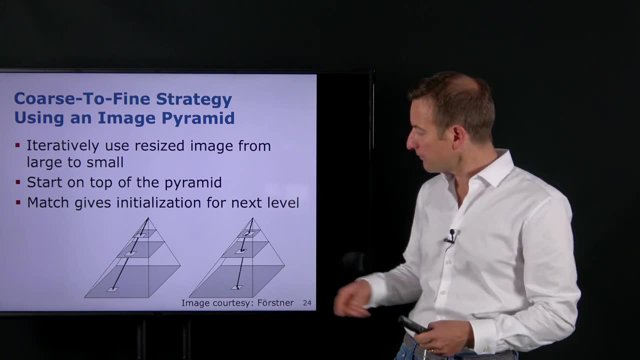 if I use the original image, I would need to slide over the whole image on the lowest level. That would be the naive, exhaustive search approach that we have described before. What I can do as an alternative: I'm first looking for the template only on the highest. 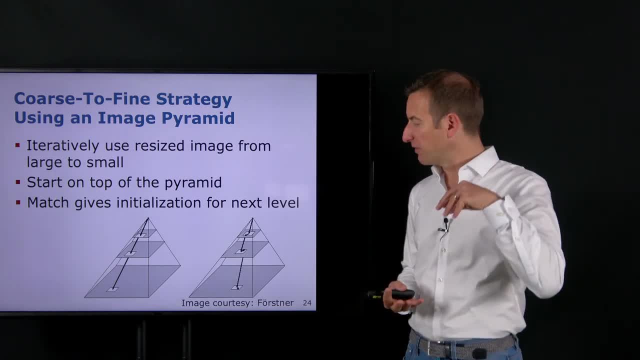 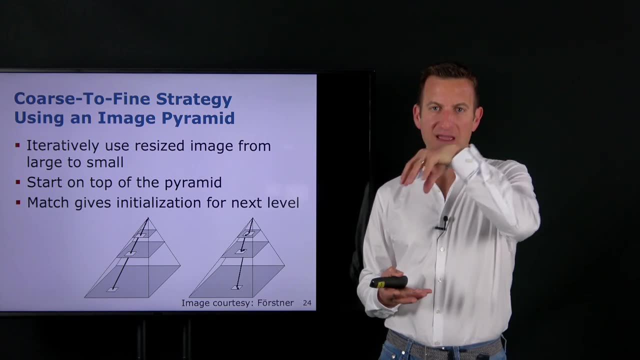 level of the pyramid, And so in this case I can basically actually nail it down where it actually is located. And then I say, okay, now let's say the resolution of this area, here is just whatever is. sixteenths of the resolution. 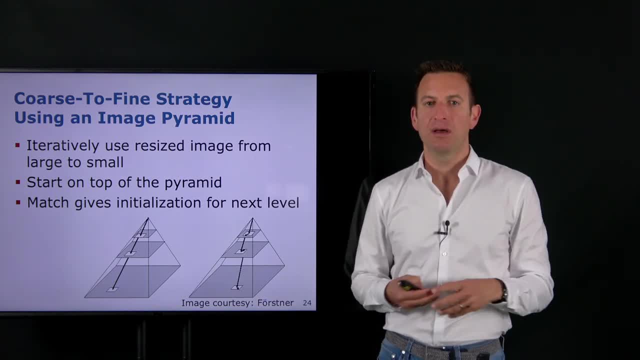 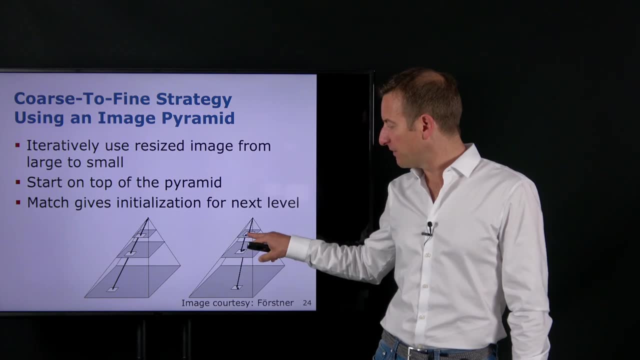 of the area down here. So I have a higher uncertainty where it actually is located, just based on the discretization that I have. But then I can say: okay, I can now go one level down and start from this point and only to look in this local area. 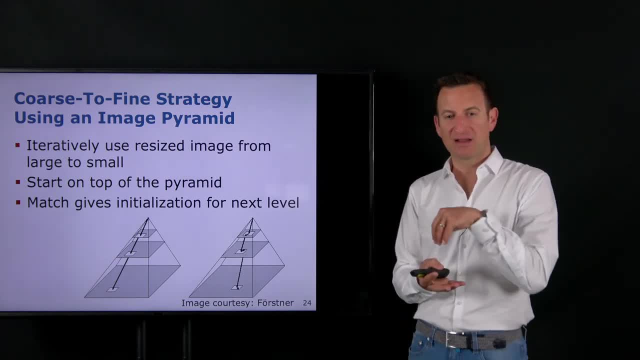 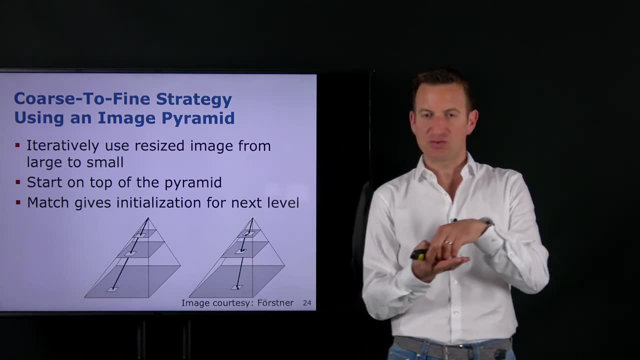 that overlaps with the original template and can kind of pinpoint where the template is at this kind of lower resolution. Then I can go a step down to the highest resolution level and can actually find my template. So this is a way how I can iteratively 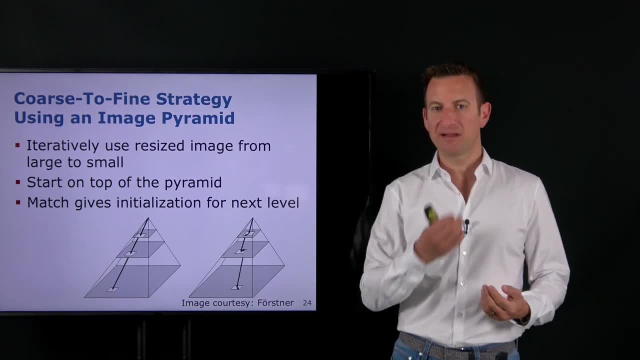 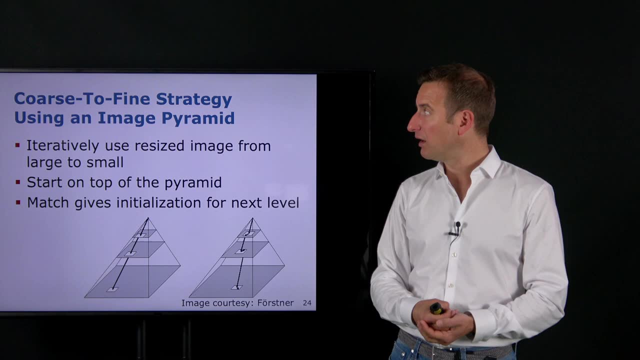 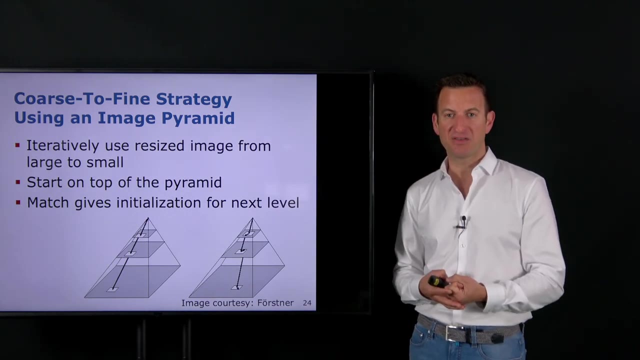 go from one level to the next level until I am at the most high resolution level and find my template over here. I could also use the pyramid if I want to look over scales. So if I don't know if my template has been scaled, 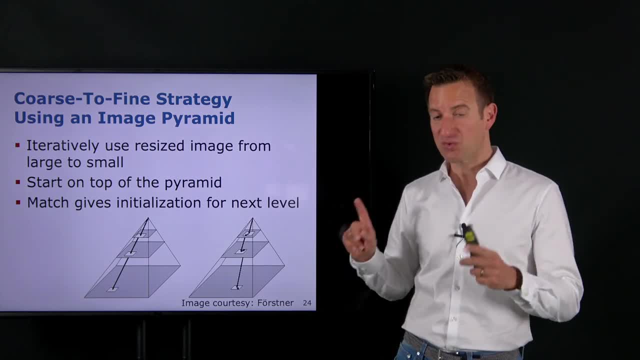 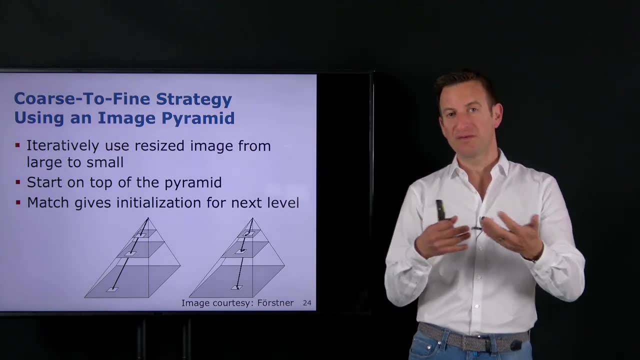 then I can of course use a different approach, and then I simply need to make sure that I don't actually scale the template when I go through the different levels of the pyramid. But these are kind of two different approaches that I can both address using the pyramid over here. 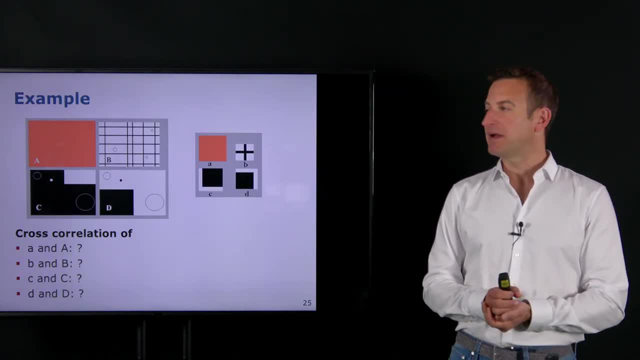 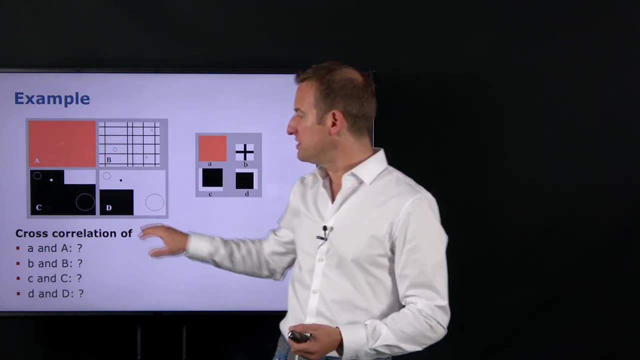 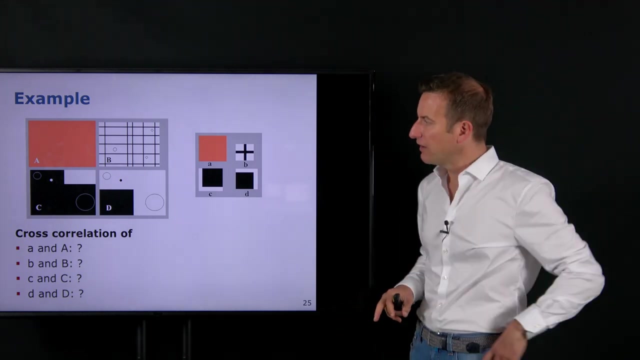 Okay, let's look into a small example to get a slightly better understanding of what actually happens here. So consider: these are four examples- A, B, C, D of images that I want to have, and I have templates which actually look like this. 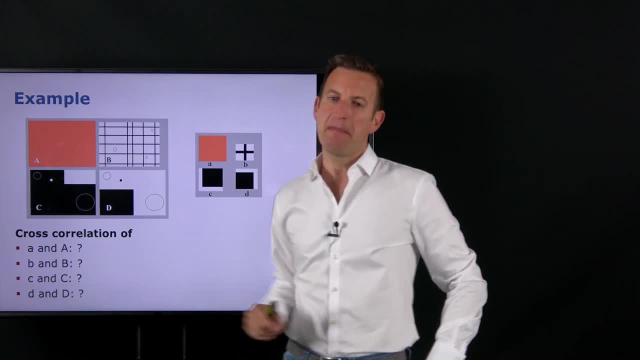 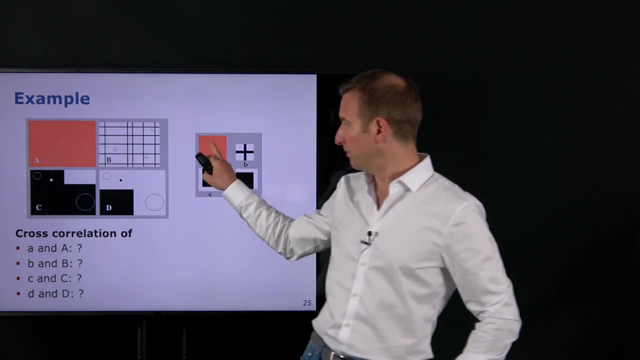 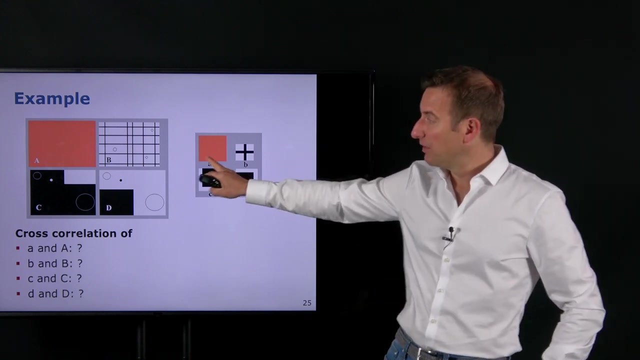 So how well does lowercase a matches uppercase a? So this is one example. So how well does cross-correlation allow us to pinpoint this area in this image? How good is that? So wherever I slide lowercase a and uppercase a, it will always be a perfect match. 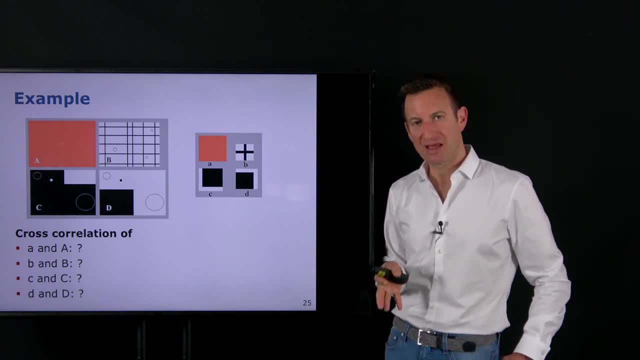 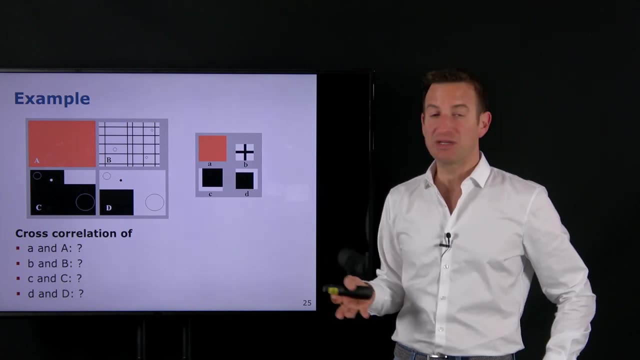 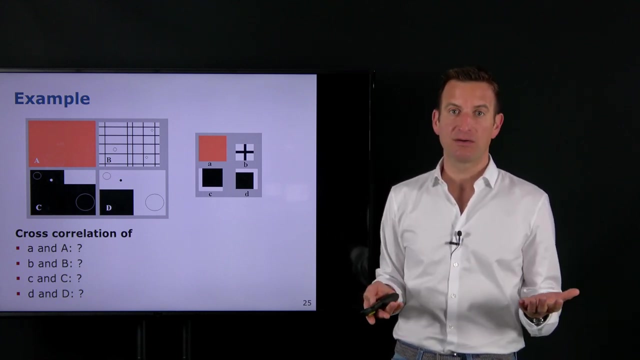 So there's no area which stands out which allows us to localize this point. So the normalized cross-correlation coefficient will actually be very high. The normalized cross-correlation will be high, will return a high value, But none of the values actually stands out. 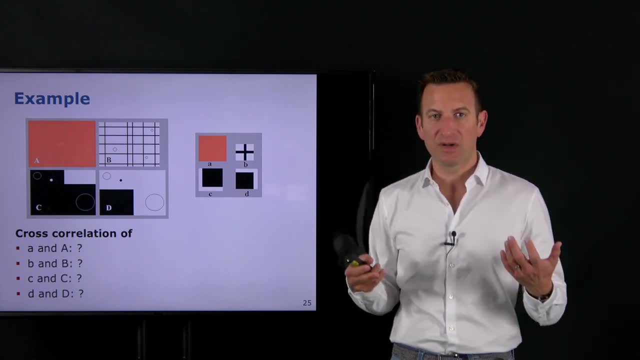 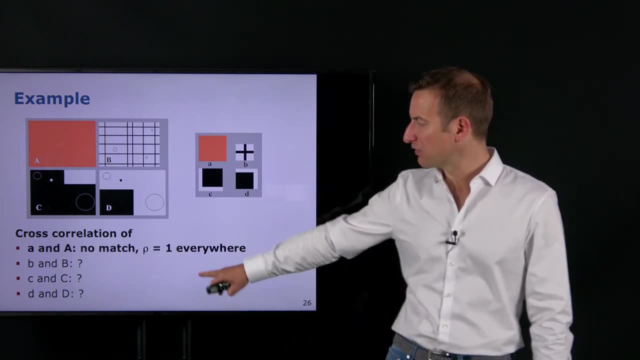 And if none of the values stands out, there's no way that I can say whatever, offset 2, 2 is better than offset 10, 10.. So, as a result of this, I will basically find no match, because the similarity value 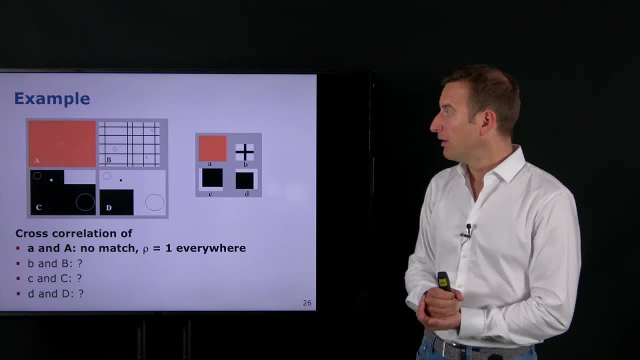 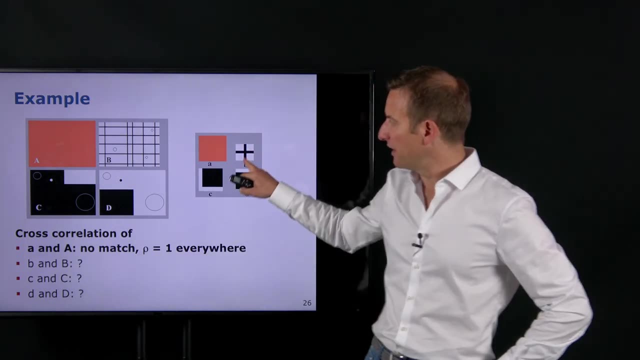 is the same everywhere. Okay, let's look at the second example. How well does lowercase b fits into uppercase b? And it turns out that they are locally distinct areas, So I can slide it and we look at different values, So we won't suffer from the problem. 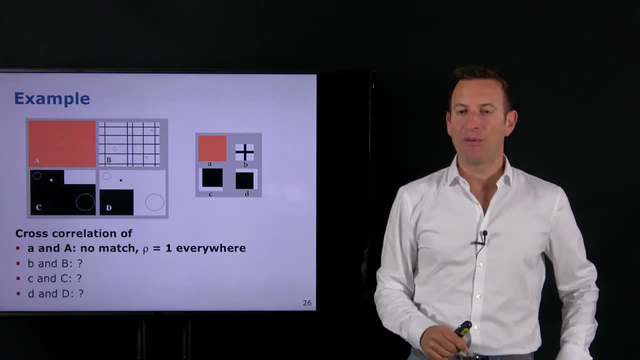 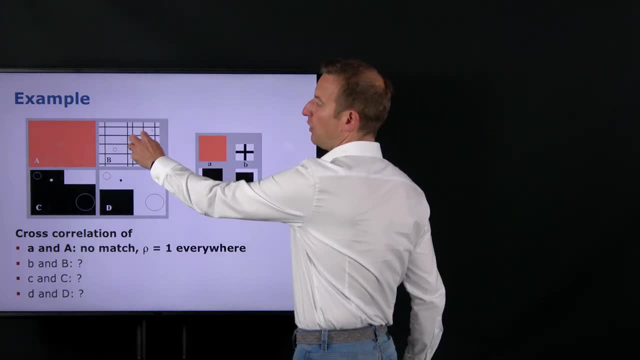 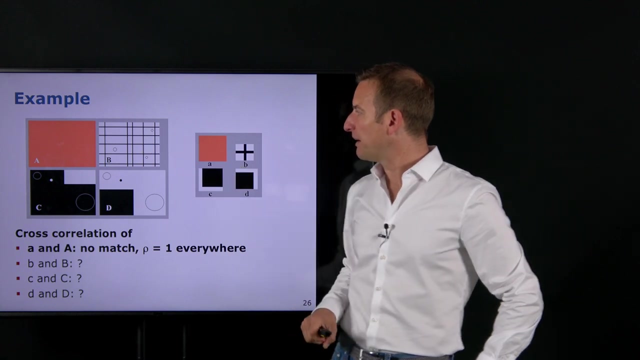 that we have here in our first example. However, there's no unique solution, because this small template basically fits over all intersections of these horizontal and vertical lines. Maybe not this one over here, because maybe the circle would overlap, so it would get a slightly slower value. 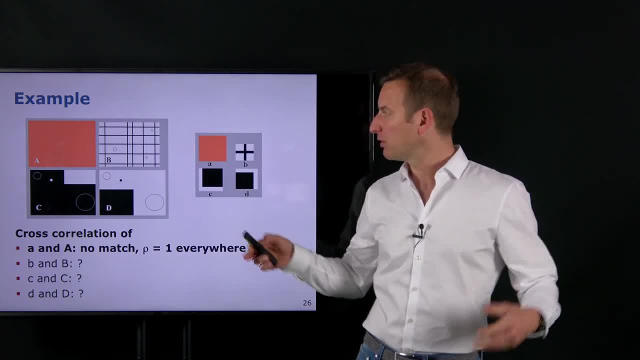 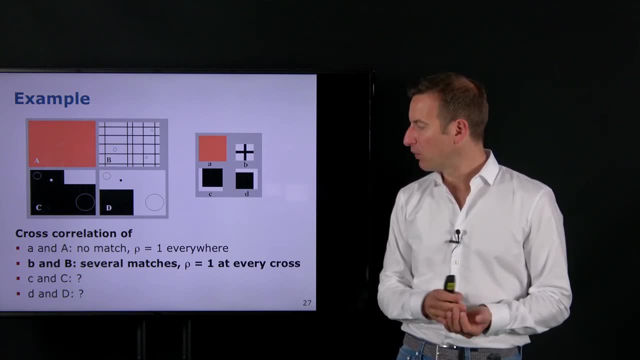 But basically for all crosses or all crosses where there's no other pattern or texture in the local surrounding, we will actually get a high value. So we will have basically a multimodal solution or an ambiguous solution. We say it's either here or here. 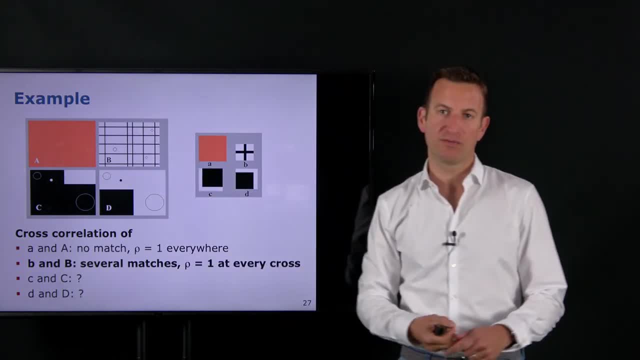 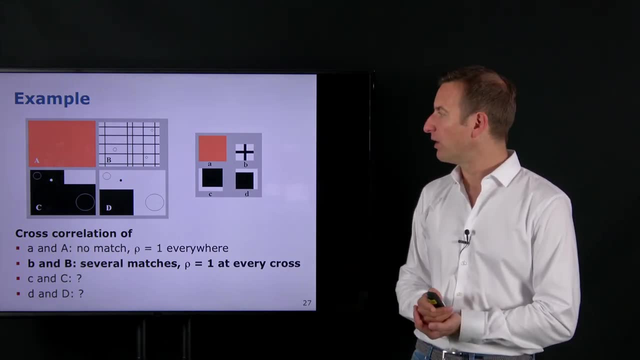 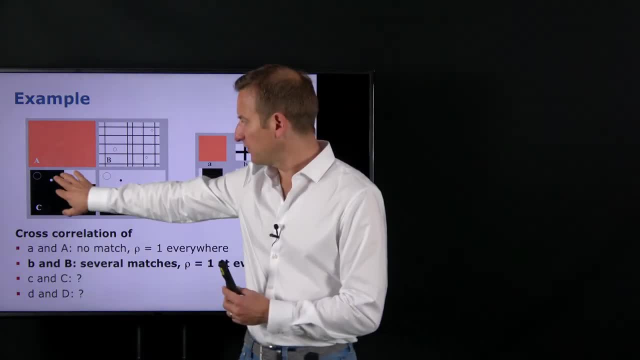 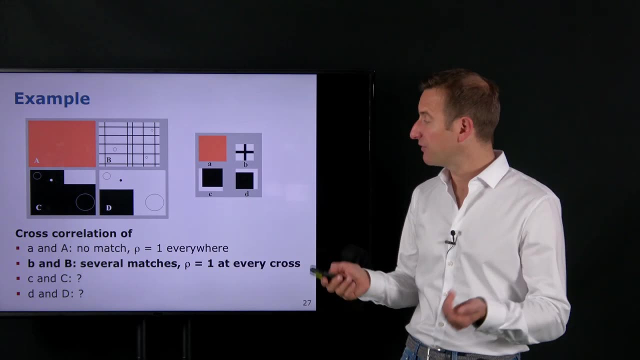 c over here. What you can see is, wherever I slide that, I will actually get no matching results. So there should be no result where I get a value that is high, let's say close to 1 or 80%, something like this. 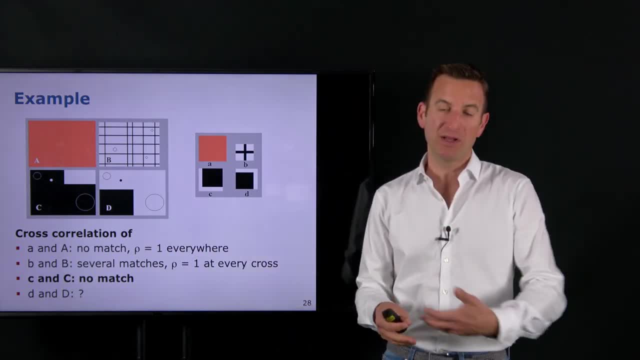 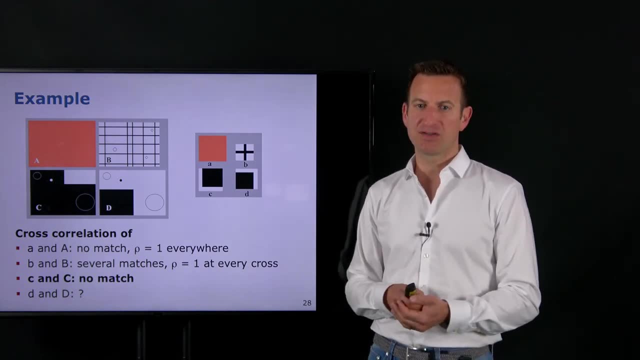 So I should find no match here, or at least there would be one value which may stand out, but this value will be really small and as a result of this, this will not be a match that I'm taking into account, At least if I take for my values. 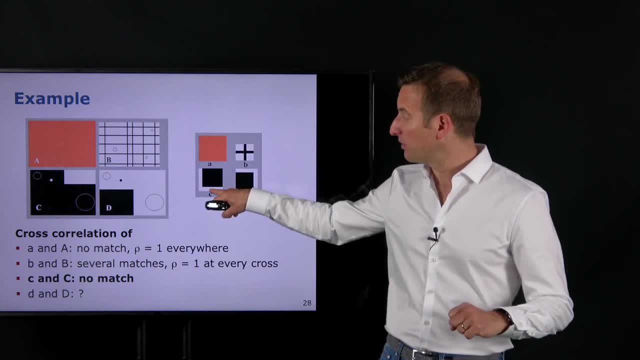 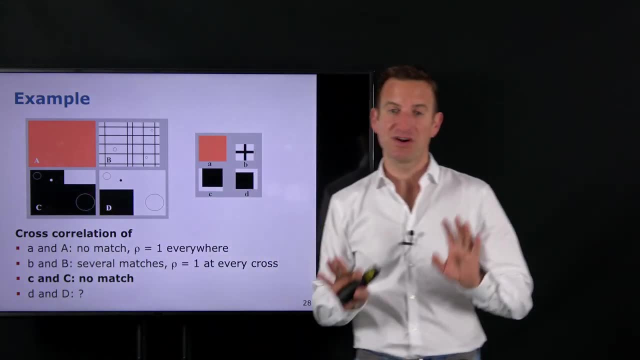 of rho only positive values. if I would go to minus 1, then I probably would find a match over here When black turns into white and white turns into black, then I actually would find a match over here. But assuming I'm not doing this, 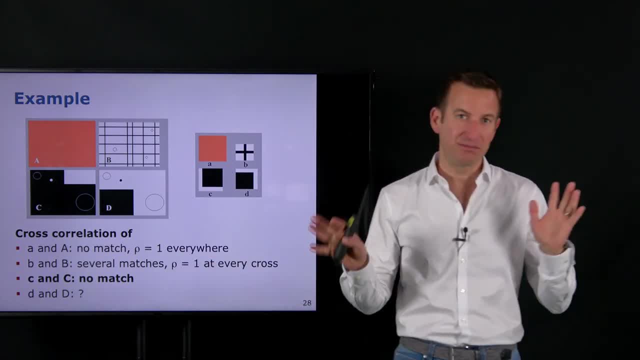 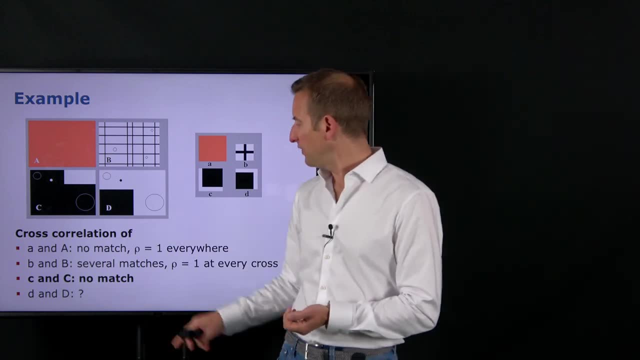 I'm only considering values that say higher than 0.8, or something like this. And then, last but not least, matching lowercase d to uppercase d. If you slide this template over this image, there's exactly one location where I have a good match. 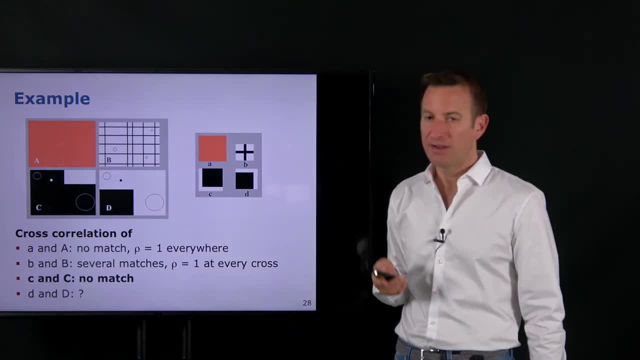 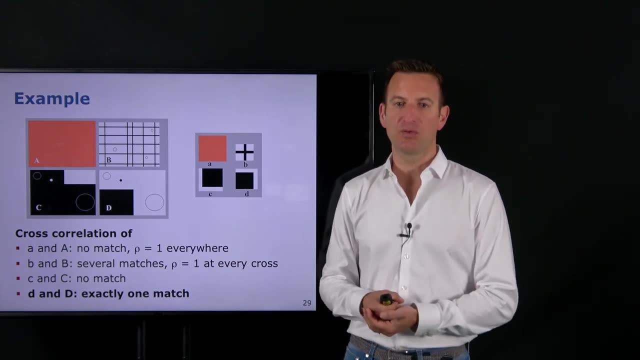 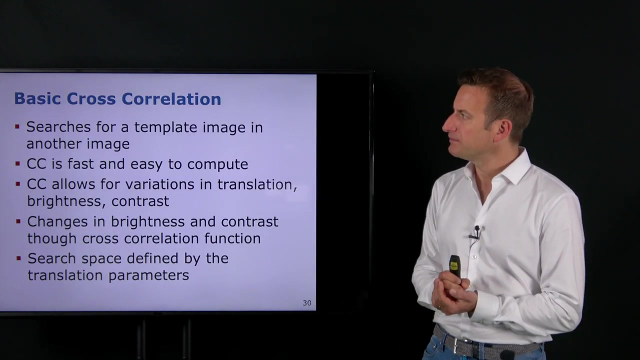 which is exactly this overlapping area over here. So if I match d with d, I will get exactly one match where rho takes a large value, close to 1 in this example, I would find a match over here. Okay, so basic cross-correlation. 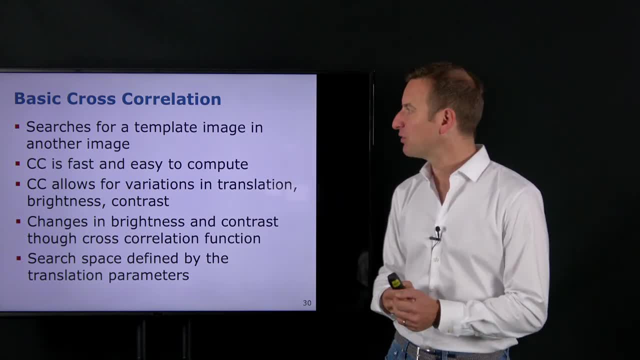 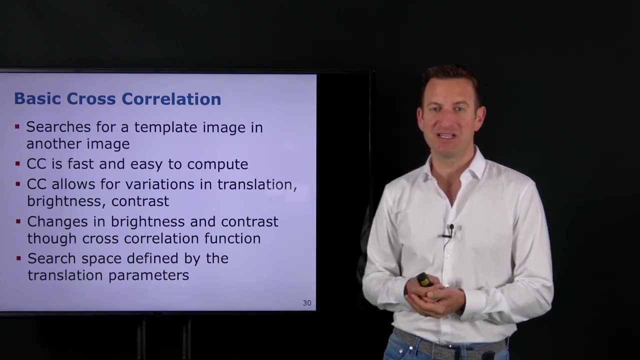 What are the kind of key properties? How do we do this? So it's basically a search for a template image in another potentially large image, And it's fairly easy to compute. The only thing I need to be able to do is computing, basically variances. 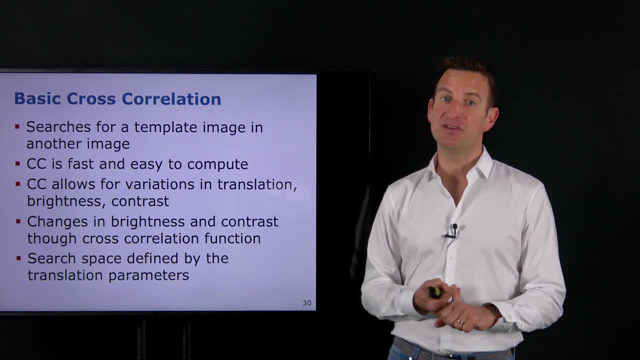 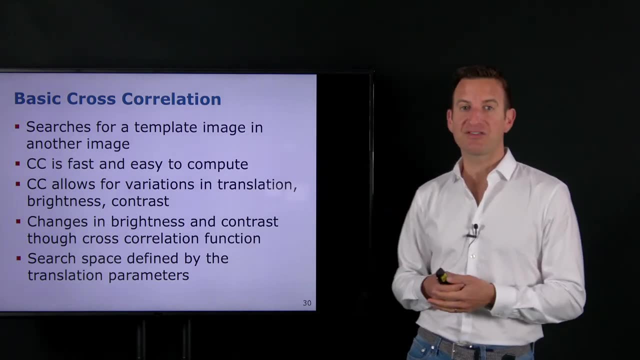 in means of intensity values, And I need to have an approach which basically iterates, slides, a template over an image, So it's relatively fast and easy to compute- at least fast if I understand what I'm doing. I only have translation parameters. 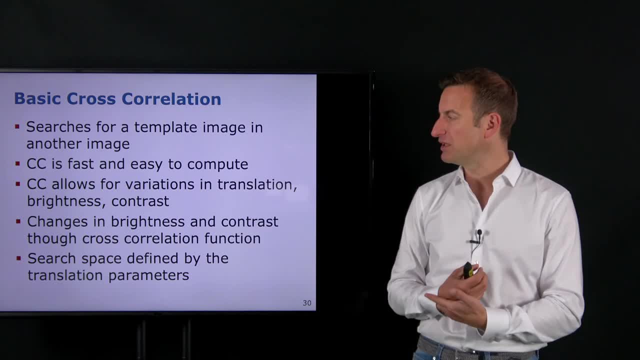 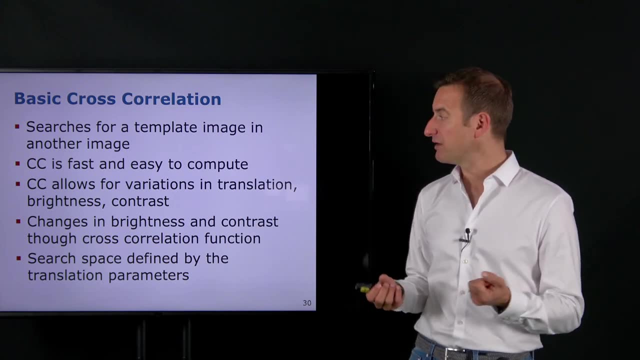 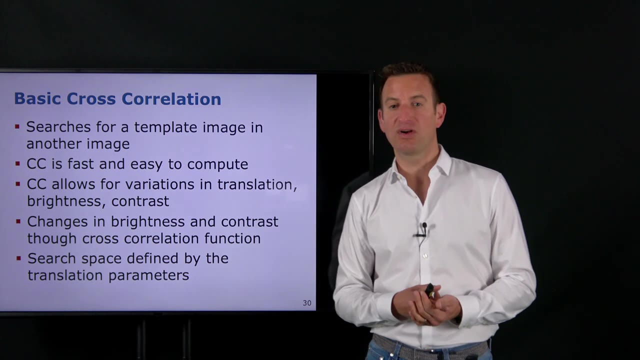 If I take more translation parameters account, this can get computationally costly. Cross-correlation in its basic form allows only for variations in brightness and contrast with respect to the radiometric transformation and the translation. for the geometric transformation There are extensions of the basic cross-correlation. 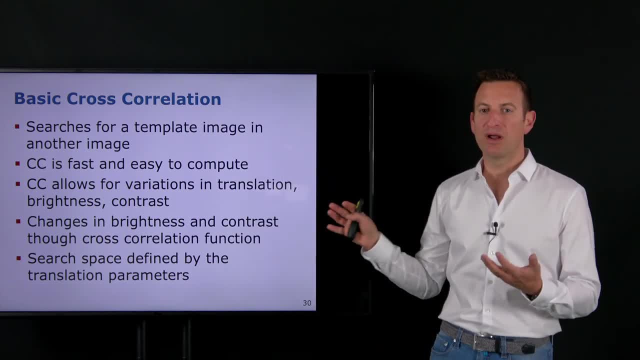 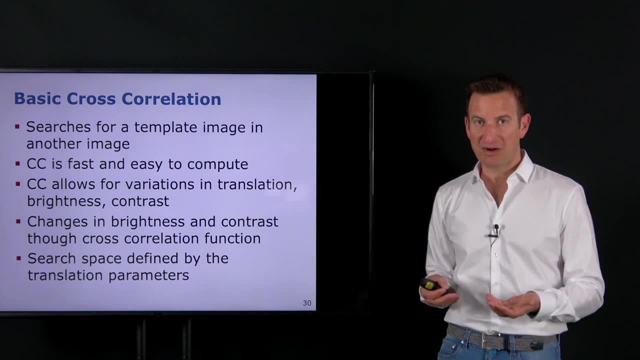 Therefore I call it here basic cross-correlation, which can do more, but this is kind of the standard approach that we use when we are doing and through this, using this normalized cross-correlation function as our similarity function, we actually have a transformation. 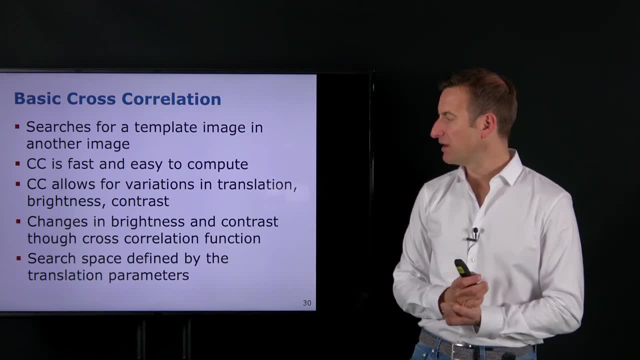 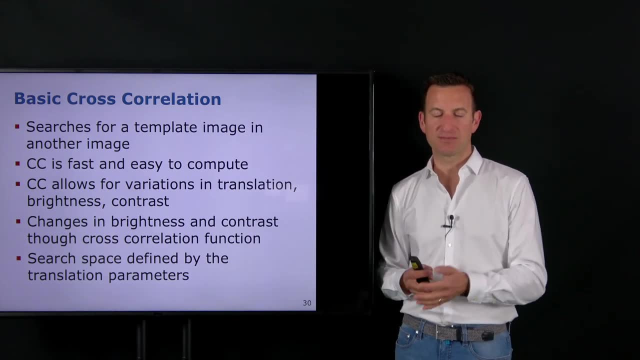 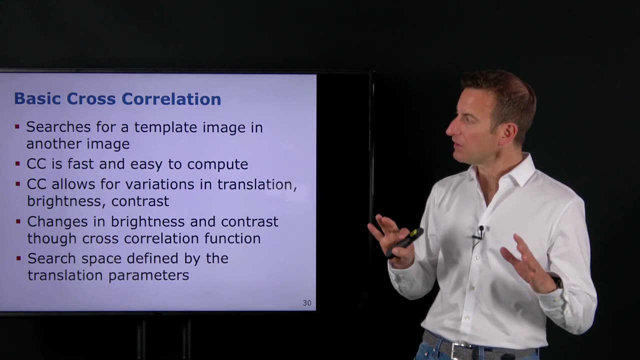 which is invariant to brightness and contrast changes, And thus, with this measure, I can easily just compare the geometric translation parameters, or transformation parameters, which are the translation, in order to, with an exhaustive search, find the best parameters. So this was basic standard cross-correlation. 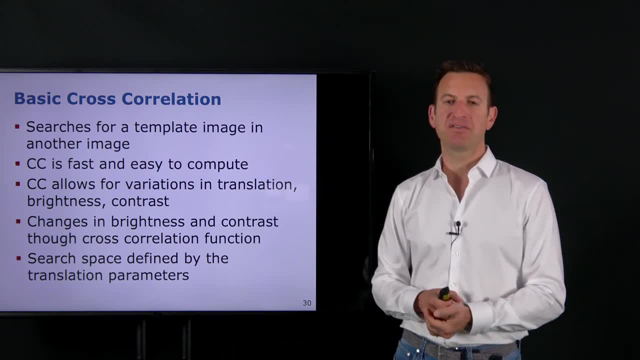 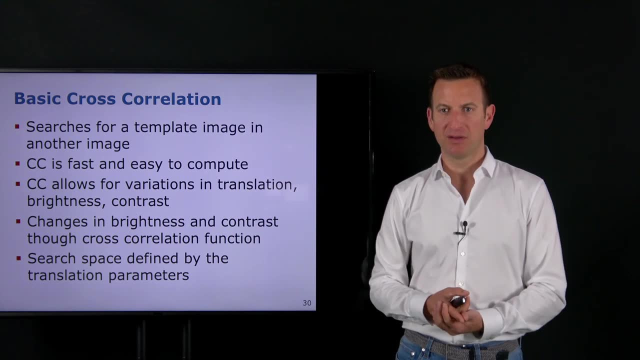 And now I'm going to show you how to perform this matching up to pixel level accuracy. But we may want to have more, We want to may go down to sub-pixel matching, And so the question is: can we actually do? 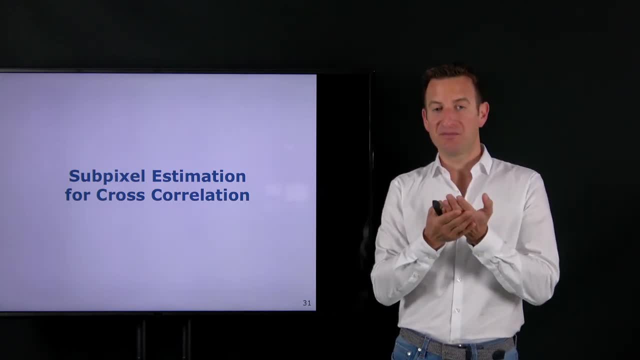 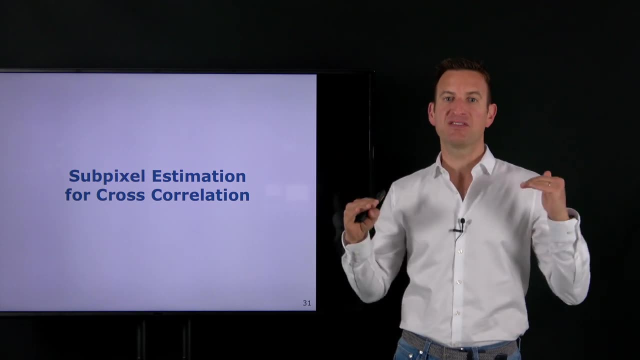 sub-pixel estimation of cross-correlation. So let's say we have this example that the airplane is flying taking two images. There's no guarantee that actually the world is shifted by exactly one pixel or exactly two pixel, And so we may want to get better. 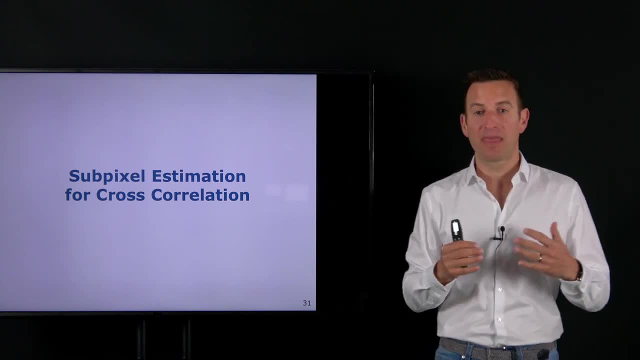 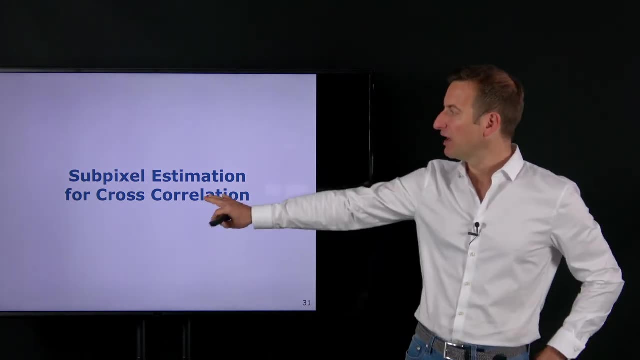 than just pixel precision for our matching, And the question is: can we do sub-pixel estimation for the cross-correlation approach? And that's something which I found surprising when I saw that for the first time as a student, that you can actually do. 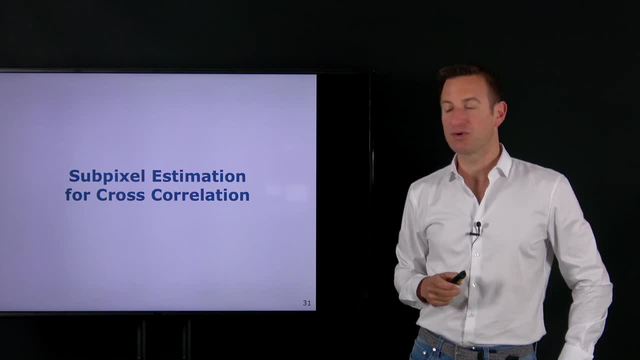 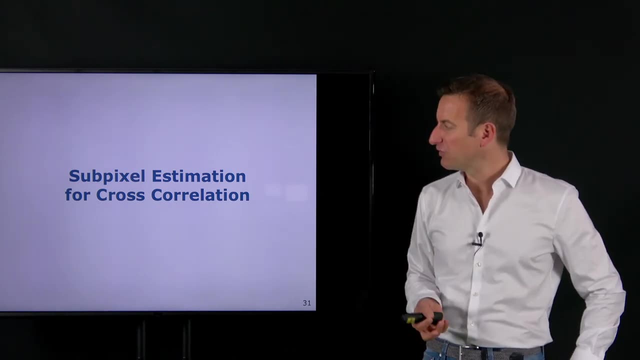 this sub-pixel matching, But I hope I can convince you that it's actually a good idea to do and that it's actually not too complicated And we have all the tools that we need to be able to do this. So I'm going to show you. 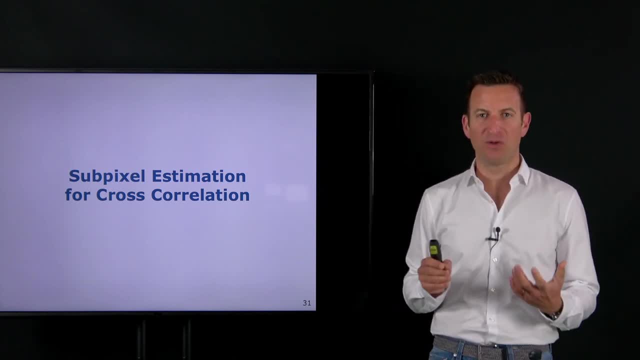 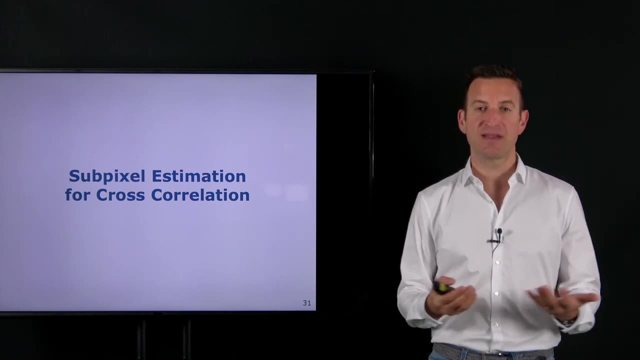 how to do this. So I'm going to show you how to do it, And we have all the tools at hand that you have learned in this lecture and the last two lectures over here looking into geometric transformations as well as local operators and convolutions. 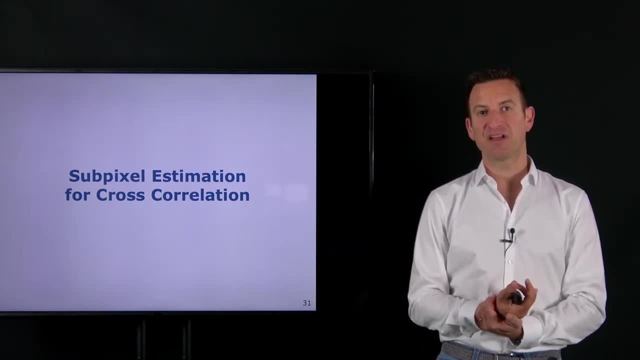 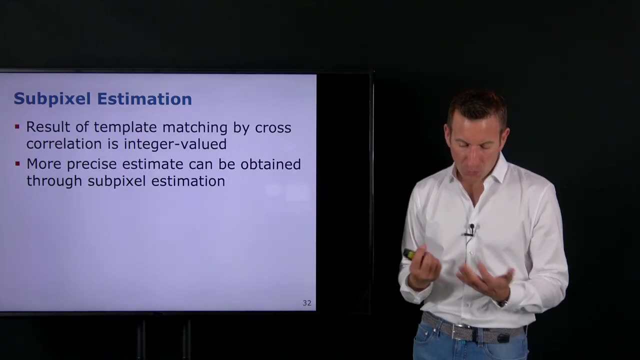 in order to exploit those properties and in order to perform sub-pixel estimation using cross-correlation. Okay, So let's dive into that and see how that looks like. So what we want to avoid is this kind of integer-valued possible shift. 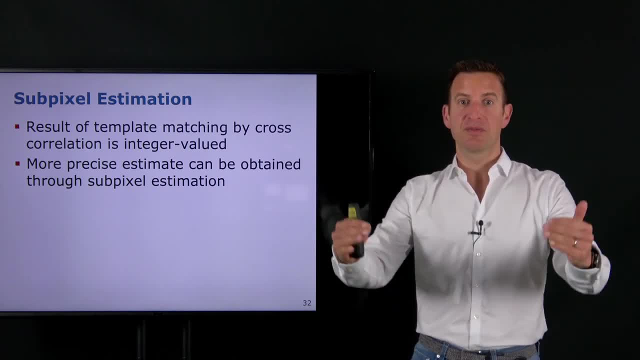 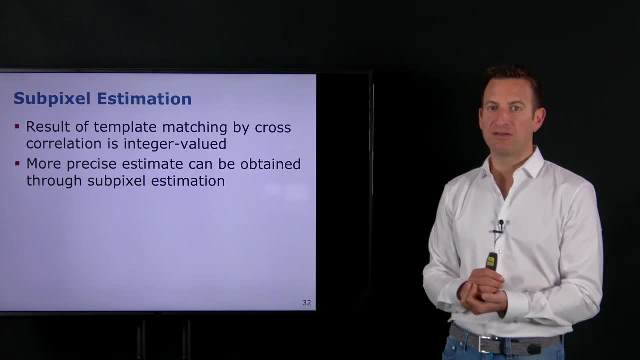 So saying I can only be shifted by one pixel or two or four. I want to be able to say: this template has been shifted by 7.3 pixels, for example, And we can obtain that by not taking into account shifts. that only happen. 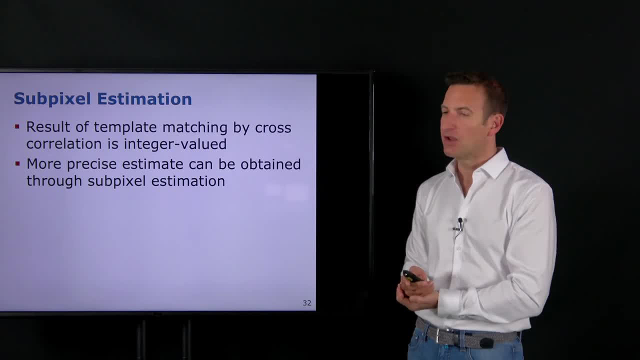 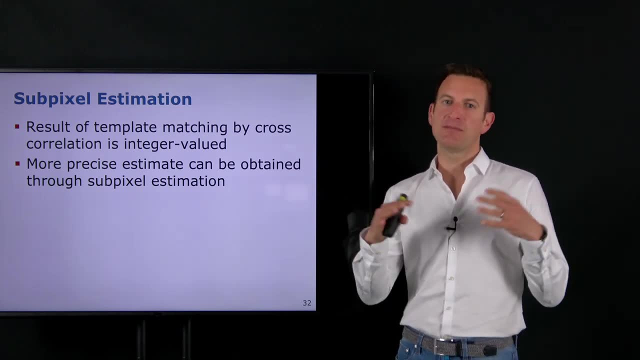 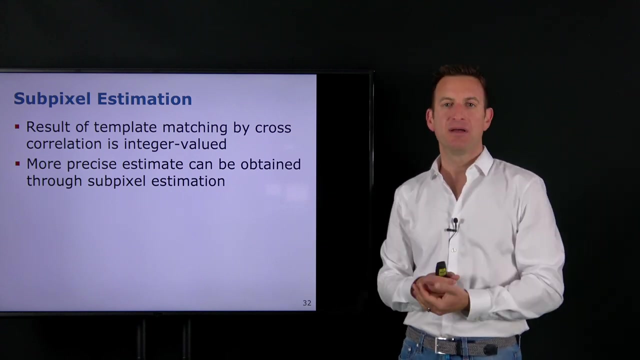 at pixel level but going into sub-pixel estimation, And for that we need to take into account that the templates and the images that we have are actually coming from a continuous function, from a continuous light intensity function, which we just sampled, some distinct locations. So 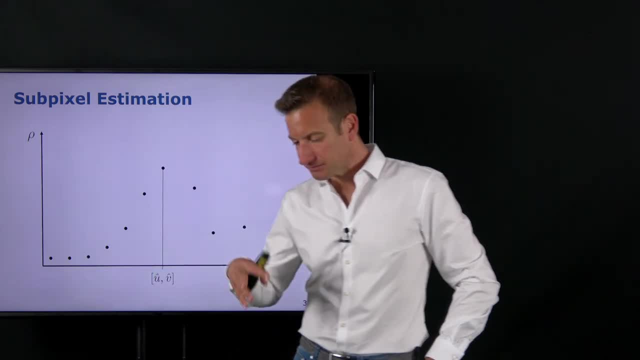 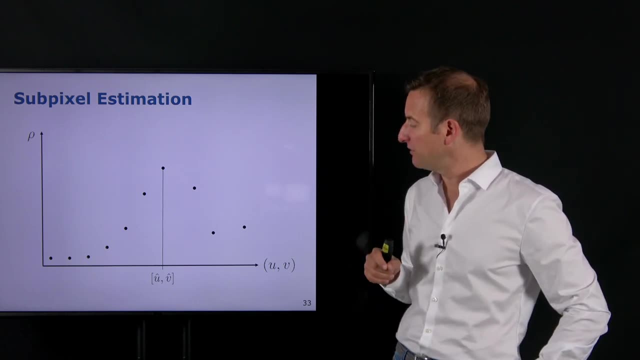 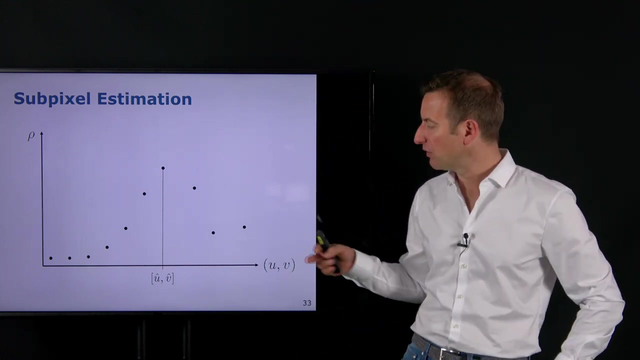 what we have in our image is basically different intensity values like this, and as a result of this, having this discretized intensity values, we have also discretized, normalized cross-correlation function values, Right. So these values over here that we compute are a result. 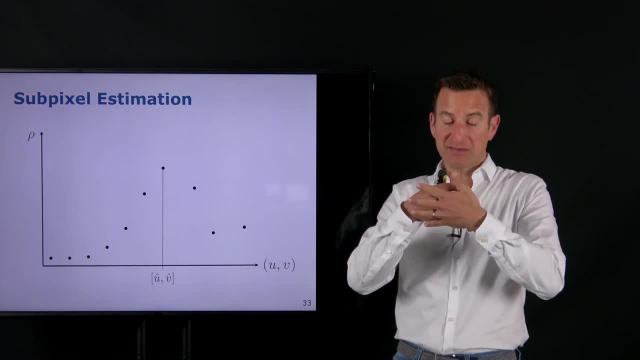 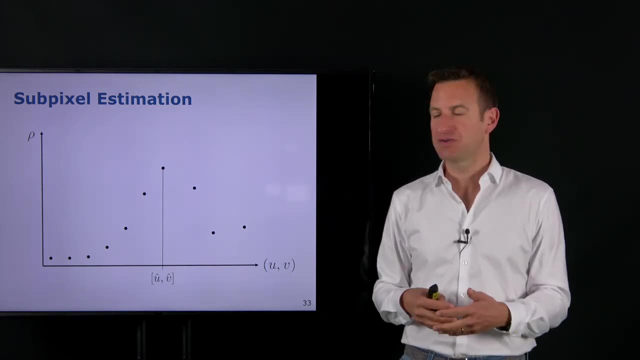 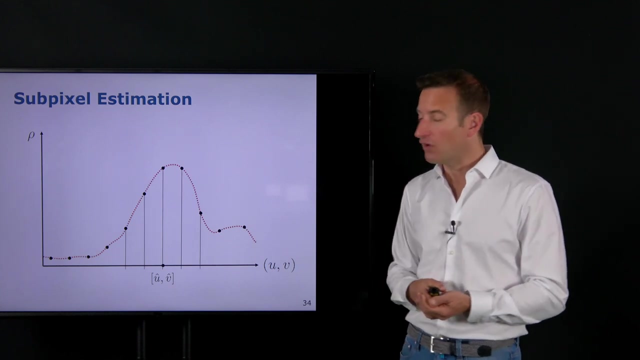 of the fact that we have the pixel discretization in our image, and this actually stems from a continuous function. So if the actual intensity values are a continuous function, then also this normalized cross-correlation should be a continuous function. So let's draw in a continuous. 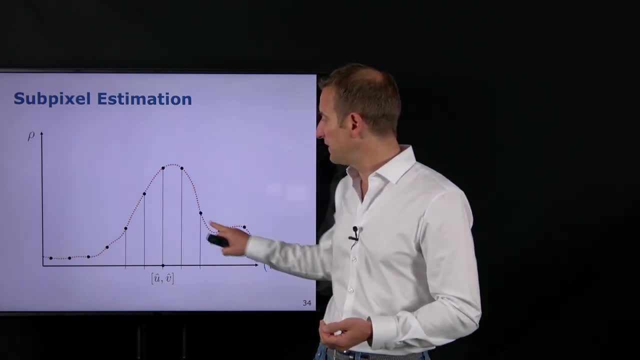 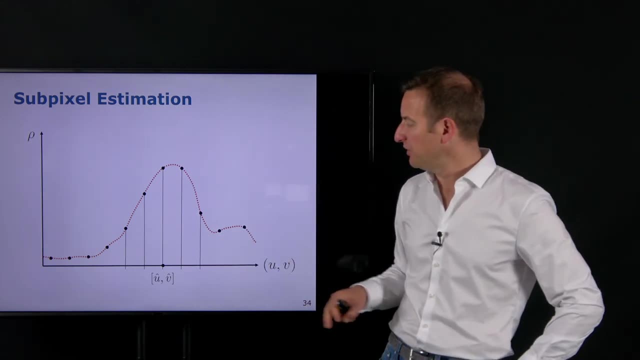 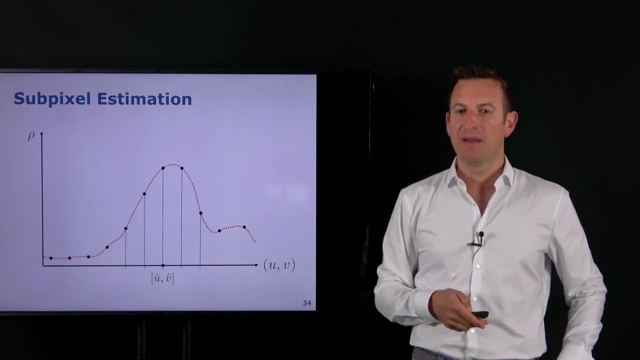 function over here, So a function which actually fits to my intensity values, and then I have, for example, two values over here which have similarly high value, then the maximum value is not this point or this point, but actually sits between. So this value over here. 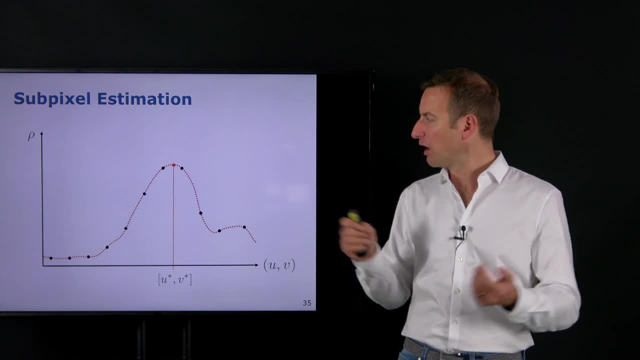 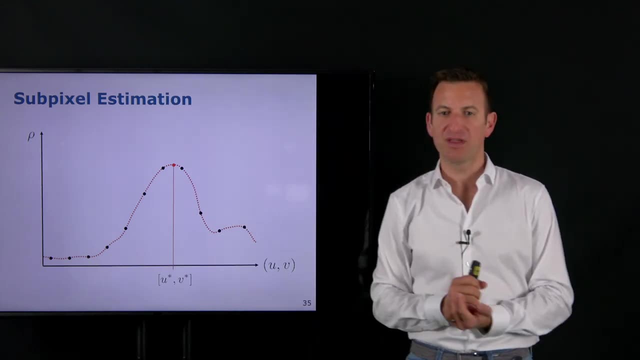 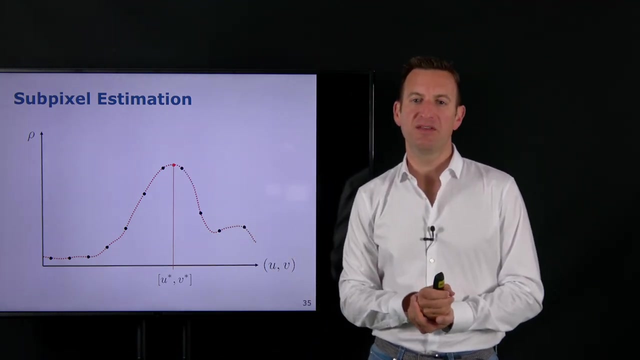 will actually be the optimal, or better it's called optimal matching value, assuming here a continuous function which doesn't do some whatever super crazy movements over here. so it's optimal solution under some assumption that there sits a continuous function between this. discretized measurements at discretized 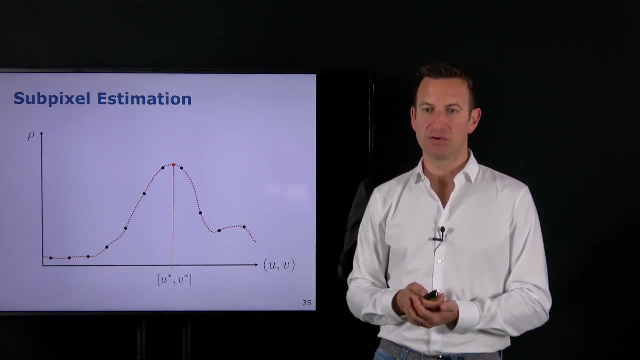 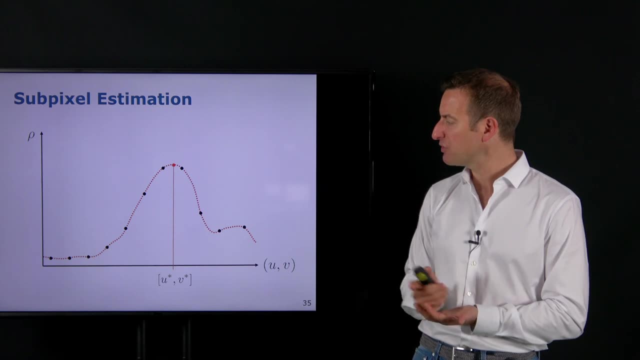 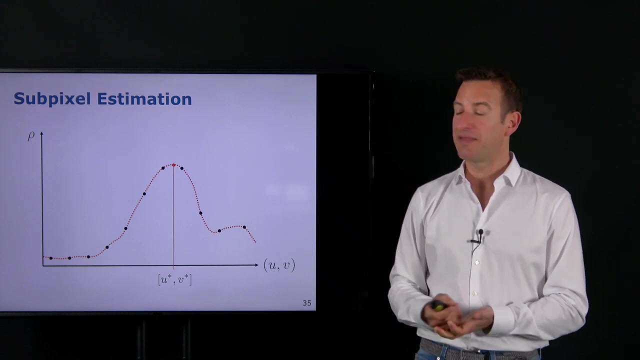 locations that I have measuring the continuous function row. So the question is: how can we do better? How can we actually obtain the actual maximum? We try to do this by using the nearby values, estimating how that ret function actually looks like and then trying to maximize. 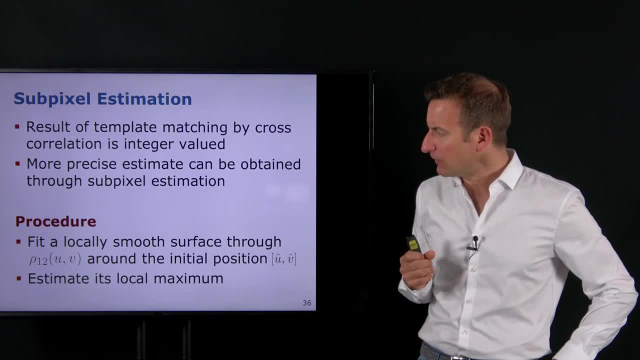 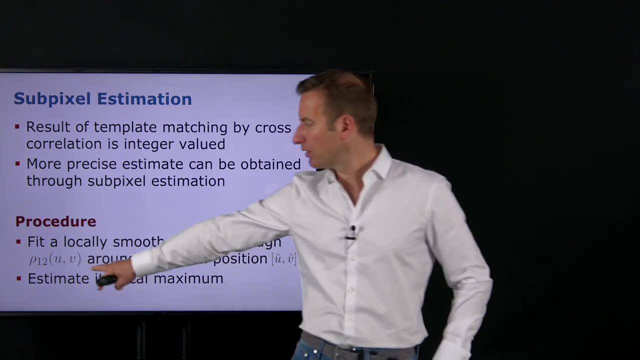 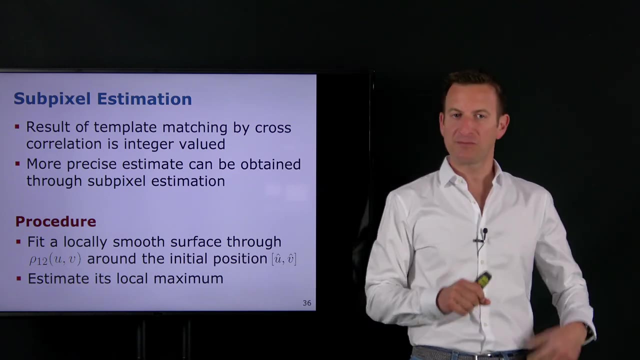 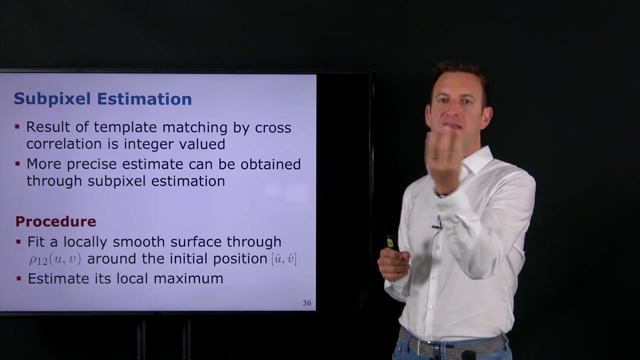 that ret continuous function, Okay. So what we can, what we do, is we basically fit a smooth function into this row or similarity function and start with the position that we have found from our standard cross correlation, saying, okay, here's the maximum, the best possible. 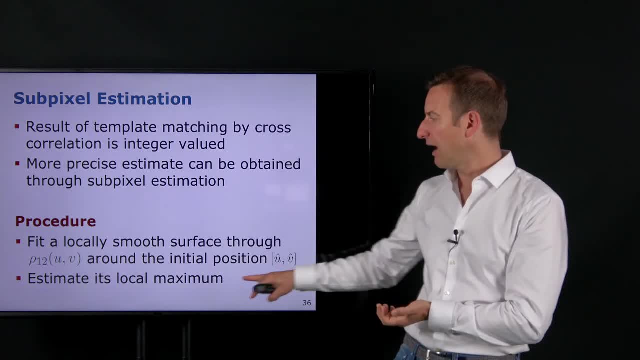 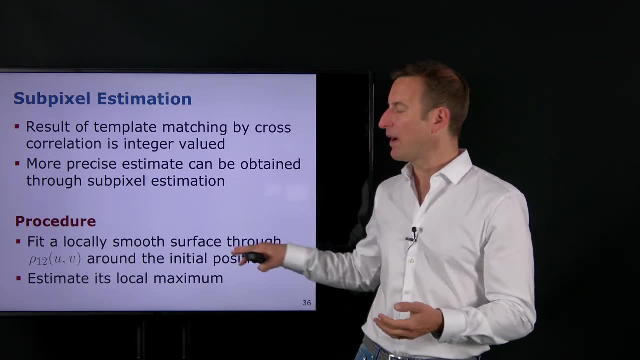 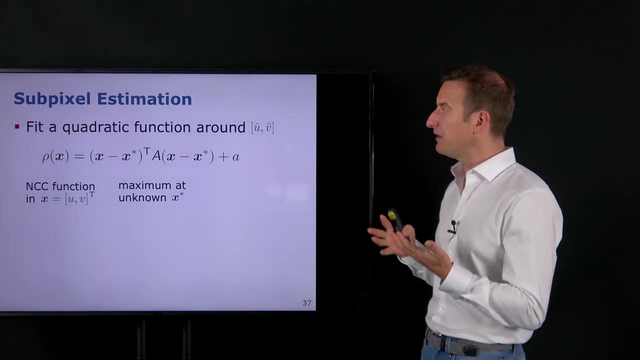 match. Let's look in this local surrounding by taking neighboring values into account, estimating how that smooth function potentially looks like and then estimating what we're doing. Okay, and what we're doing is we are. again, this is an assumption, but we are fitting. 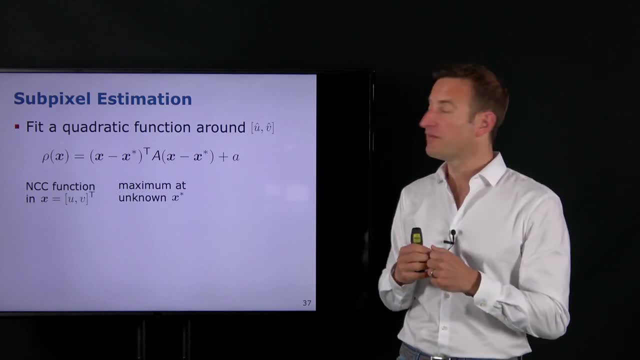 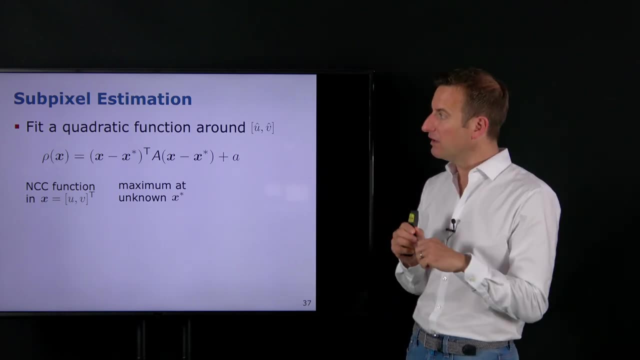 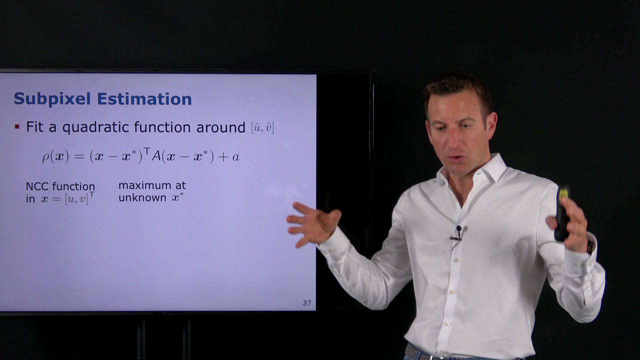 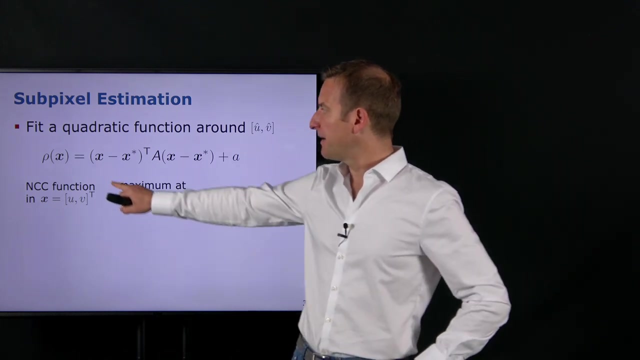 a quadratic function around our measurement values. So we're saying this intensity of this normalized cross correlation function is a quadratic function where we only have kind of sampled locations from in this local area. We don't need to do the refinement in that local area. 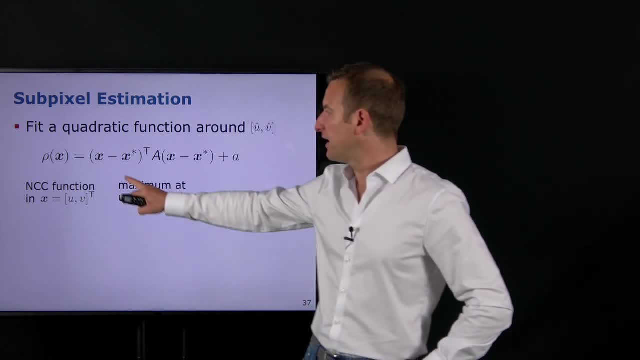 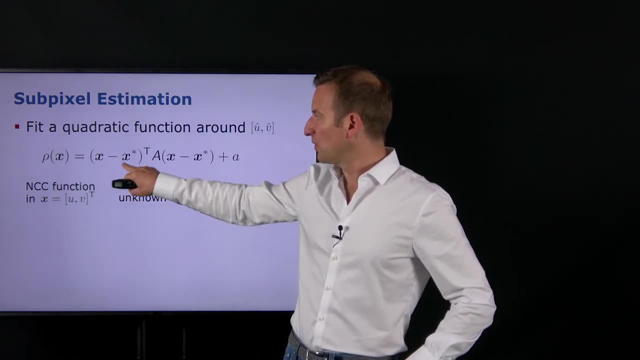 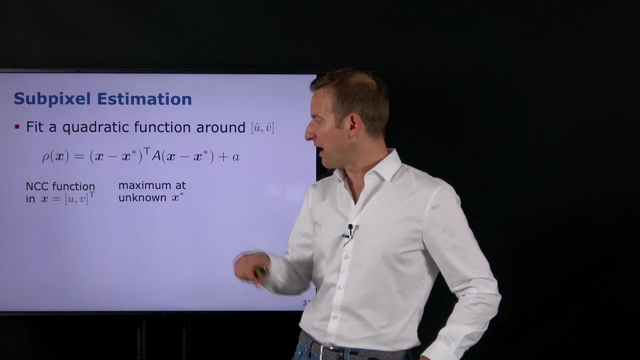 And if you have a quadratic function, you say, okay, x is our function, our offset, and x, star is this unknown thing, this unknown maximum that I want to determine. And so this function, so we want to actually find x star. 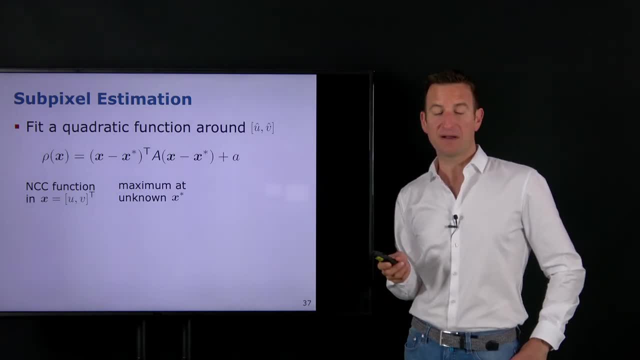 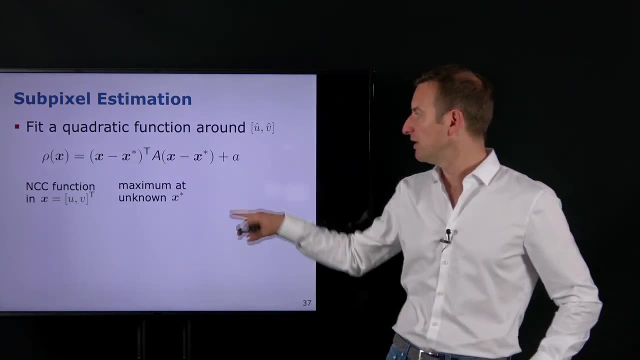 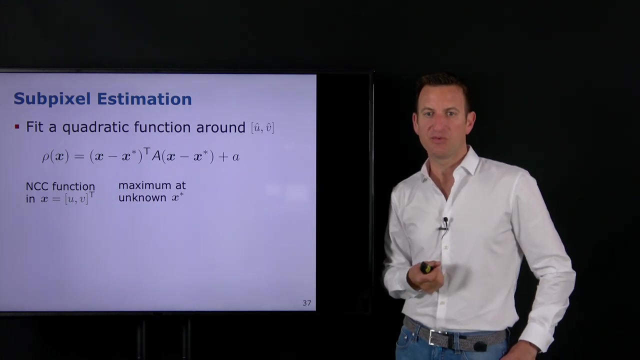 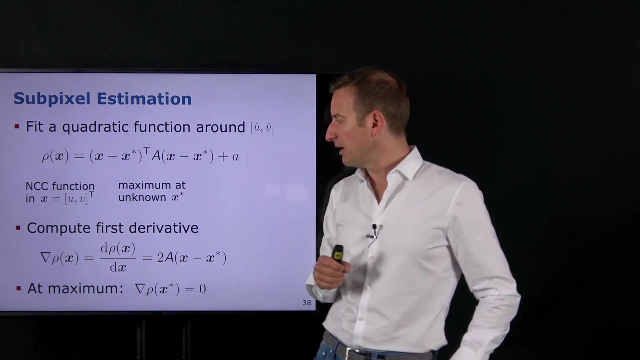 That's what we want to have. So we have this: x and x star are 2D values, and a is then a 2x2 matrix, and this is here a 1D additive value that comes in. Okay, so let's start. 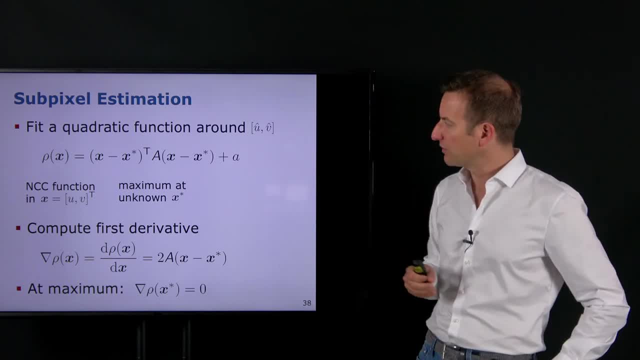 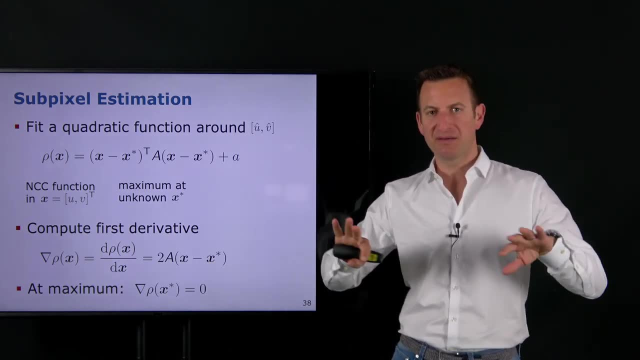 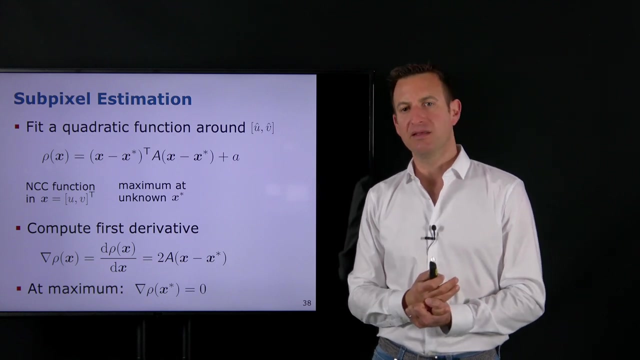 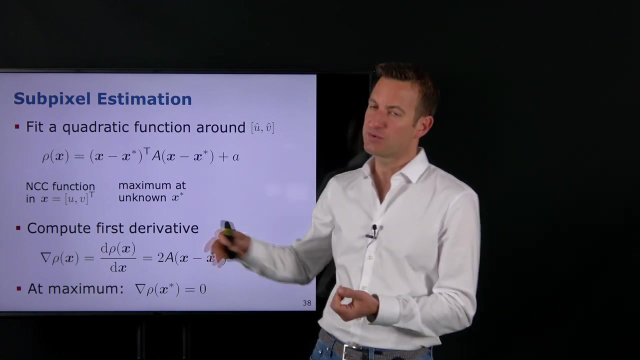 with this, and what do we need to do in order to compute the maximum or the minimum, depending if the parabola opens to the top or to the bottom? We need to look into derivatives, right, because at the minimum or maximum, we have the first. 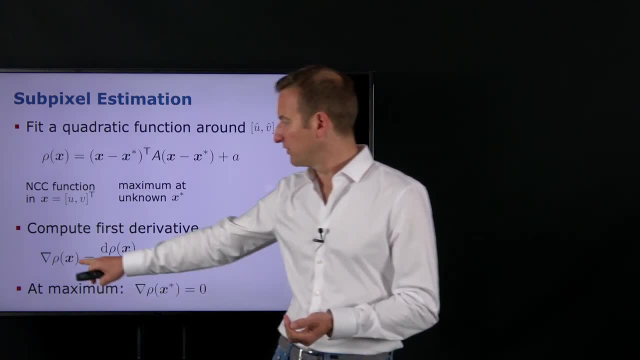 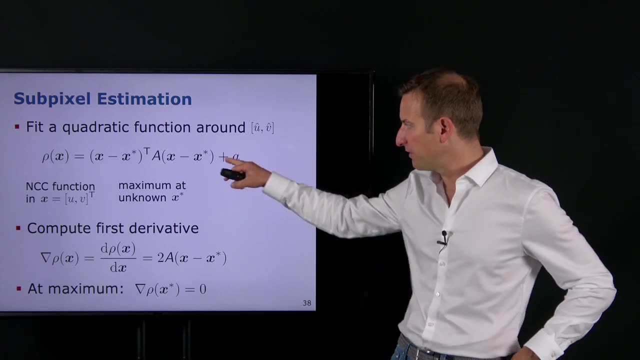 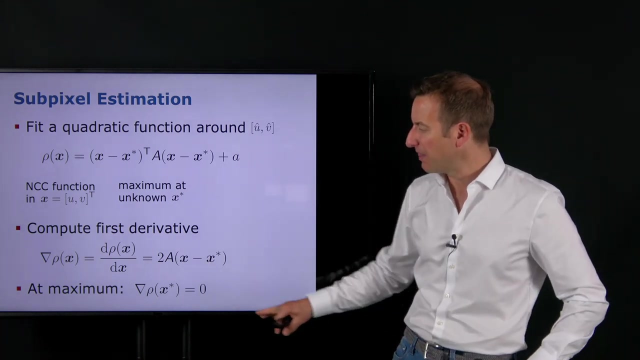 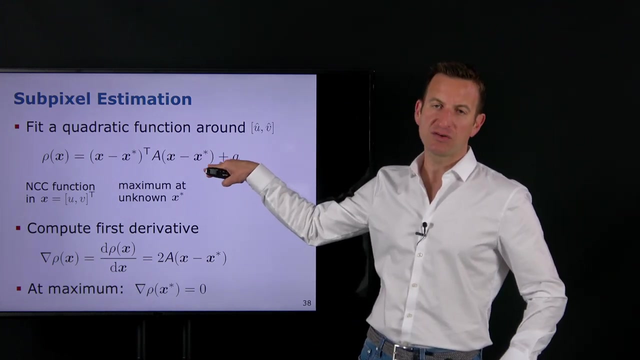 derivative being zero. So what we need to do is we need to take that function, this quadratic form, and need to take that quadratic form. This will be 2a times x minus x star, and we know that at the maximum, this first. 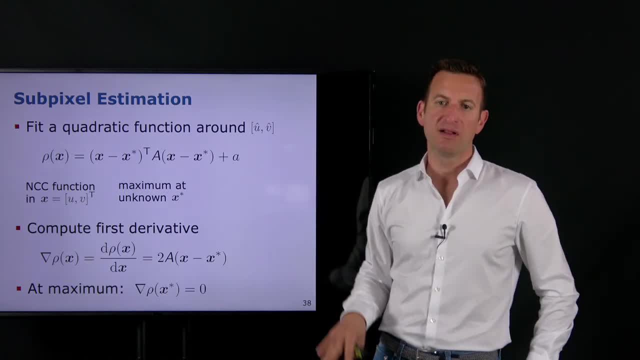 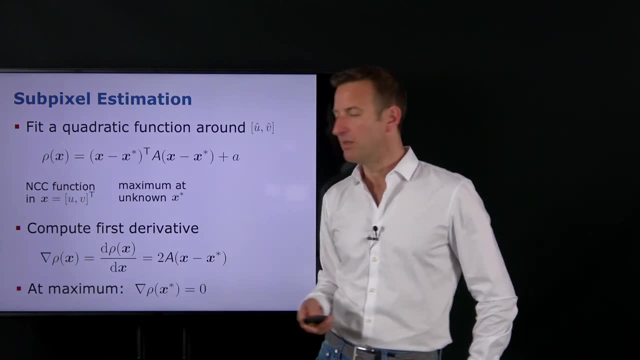 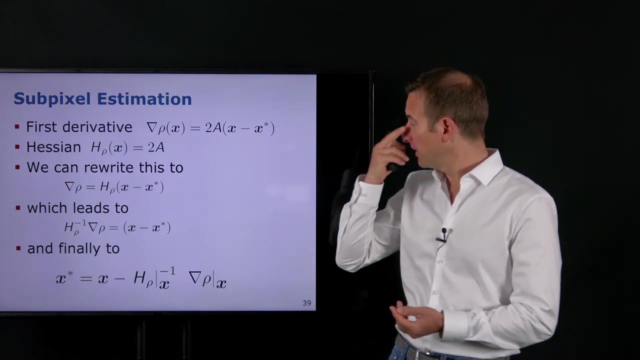 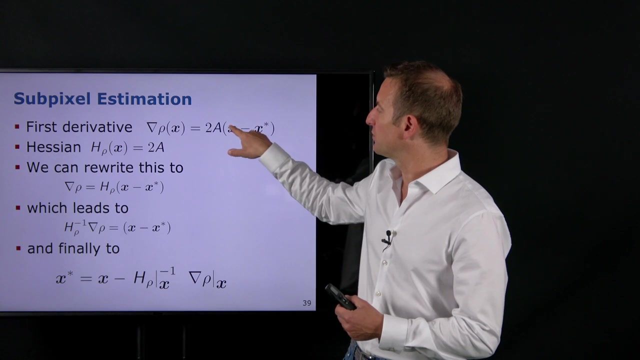 derivative must be zero. And the only thing we did is we said, okay, we assume the function looks like this: Again, there's an assumption. okay, this is our first derivative and if I compute the second derivative of that, so my 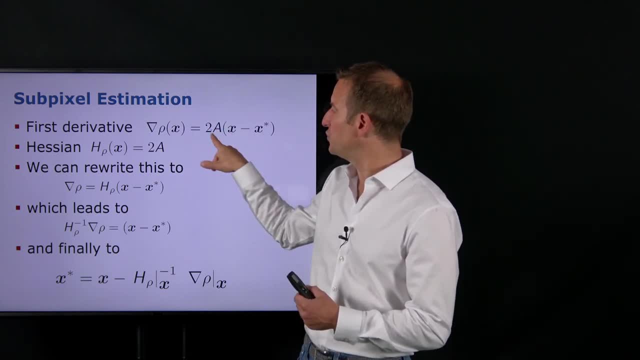 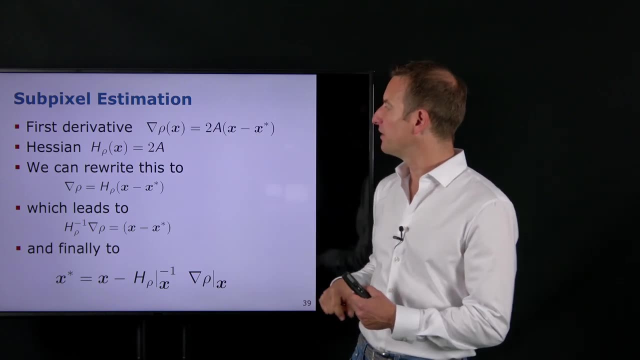 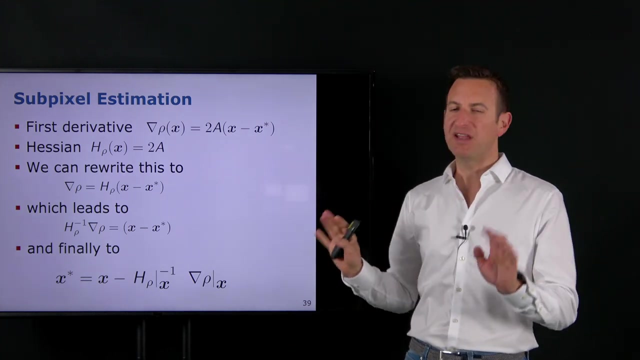 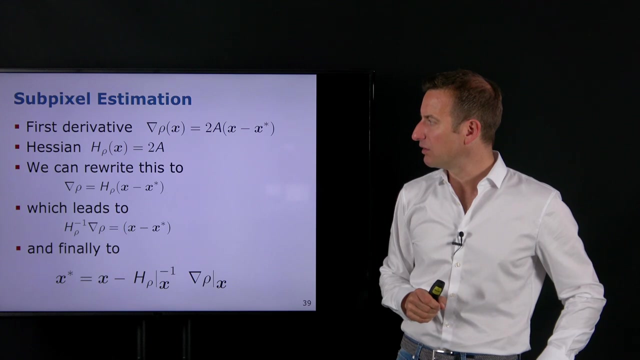 Hessian function, my Hessian, then it actually turns out that the Hessian must be 2a. So if you would compute the next derivative with respect to x of this term, this is the Hessian of my normalized cross-correlation. 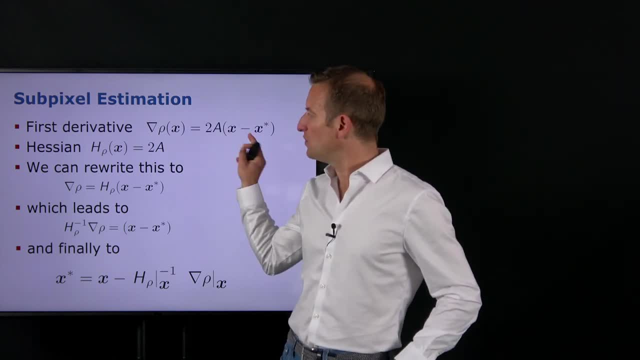 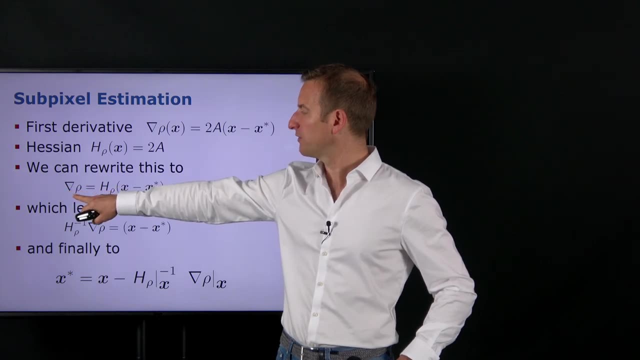 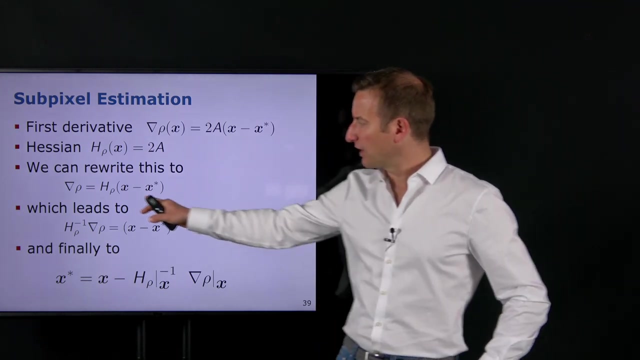 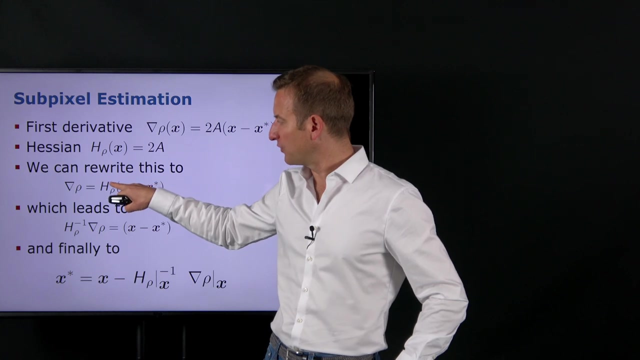 function rho. So if we just replace the 2a by my Hessian, then this function turns into the gradient. the first derivative of my function, rho, equals to the Hessian times x minus x star. So if I move the gradient, 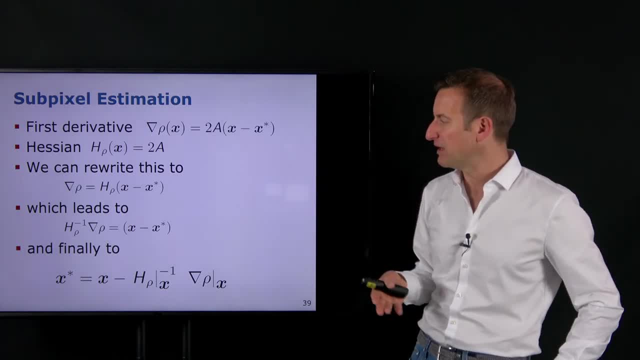 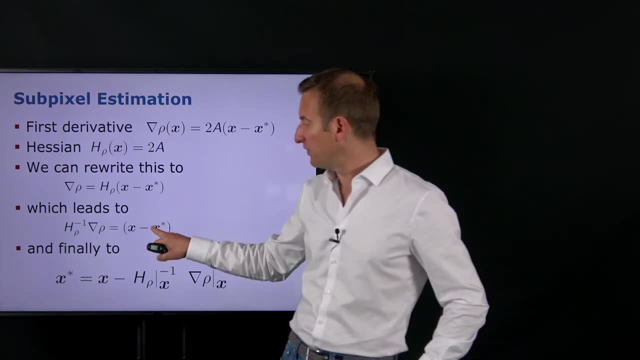 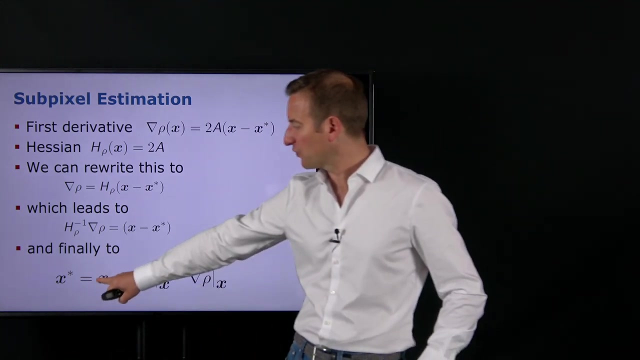 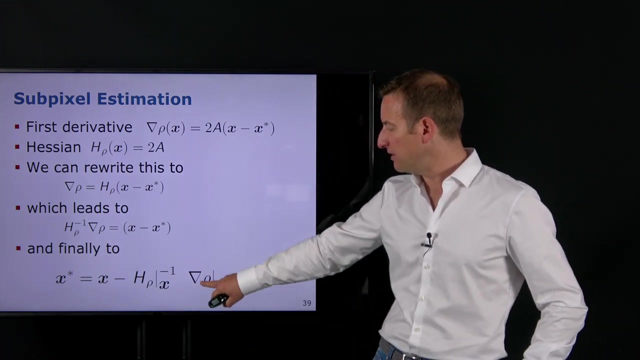 to minus 1, moves over here, this becomes the identity, so I have this term, which remains h. inverse times, the gradient equals x minus x star and x star is the thing that I want to determine, And if I said okay, 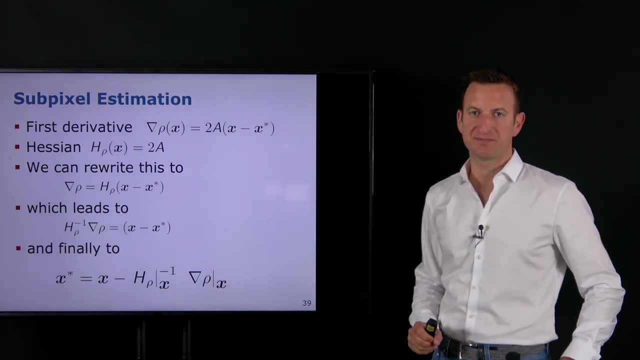 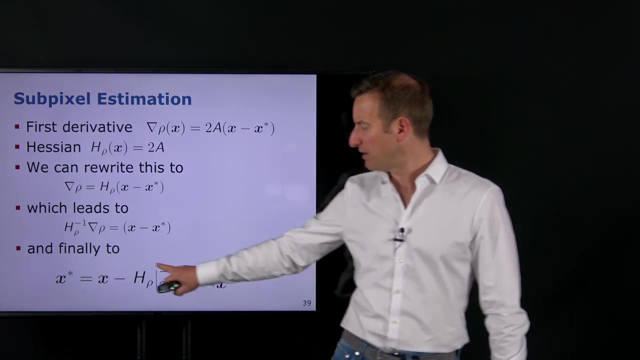 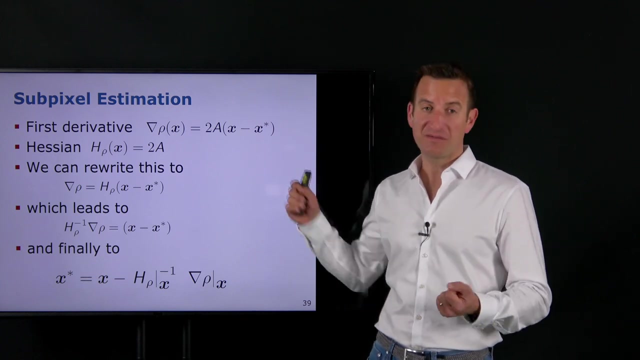 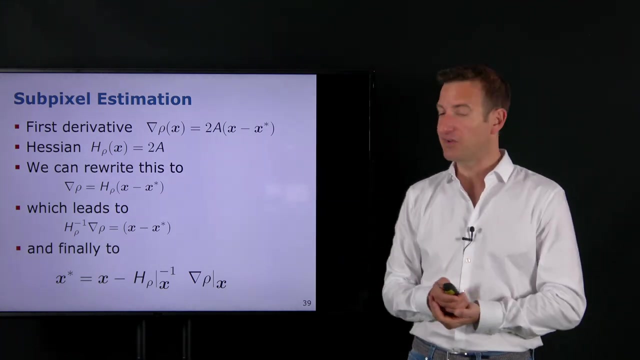 this is the gradient evaluated at that location: x. Okay, So I'm just kind of. this is just a result of setting the first derivative to 0 and doing some replacement. Why did I put the Hessian in here and not leaving? 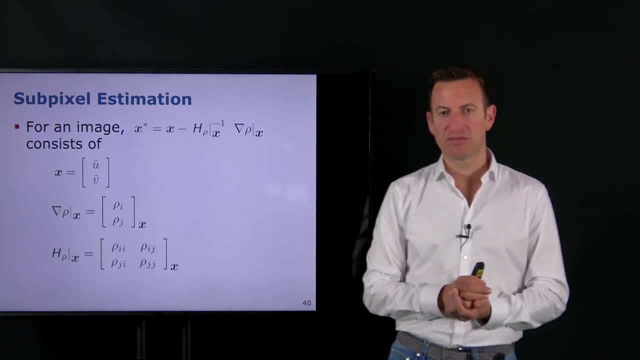 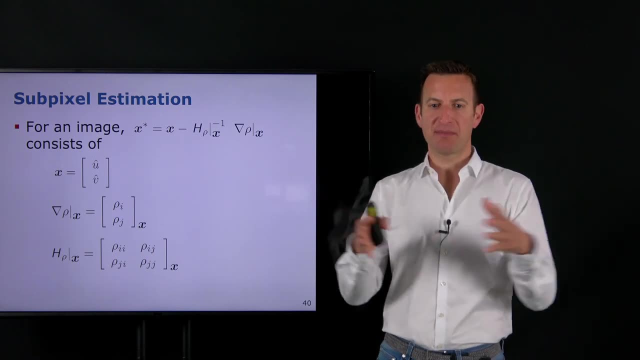 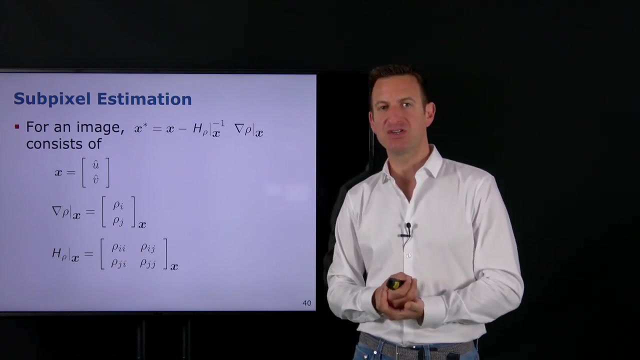 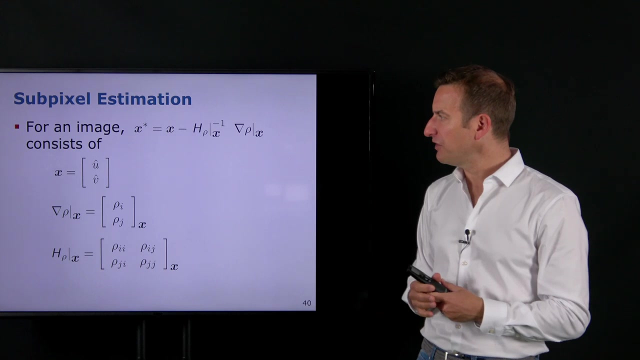 2a in here. We'll do that later. So this is an image and I can see this cross correlation function basically as an image. So we evaluated at every location. so we basically have a 2d grid with some. 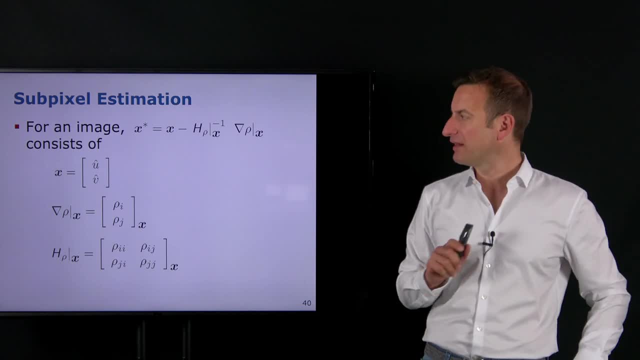 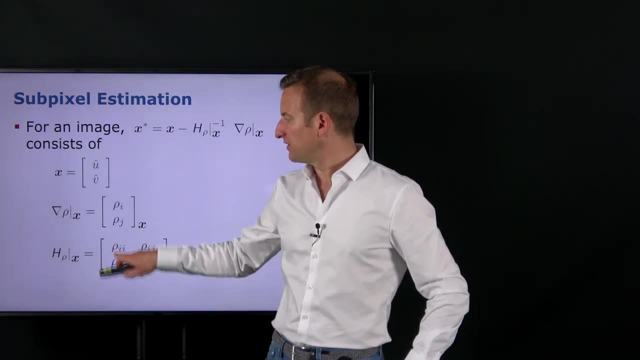 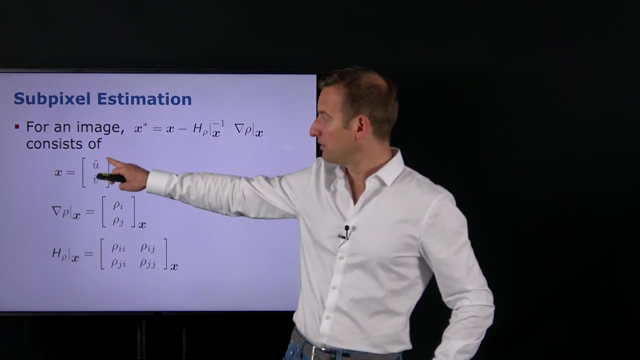 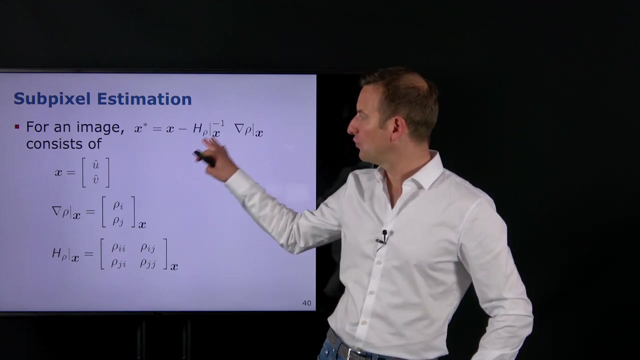 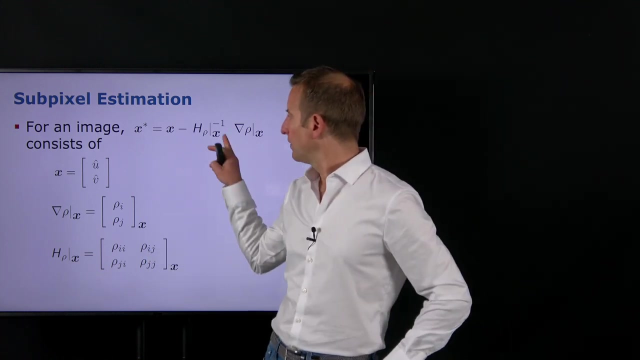 discretized value. You can see this is very similar to an image. So this is my two-dimensional shift vector. This function here is actually the gradient, the first derivative with respect to i and the first derivative with respect to j. so it's. 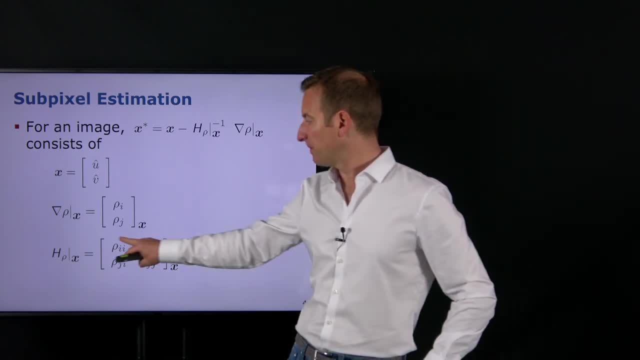 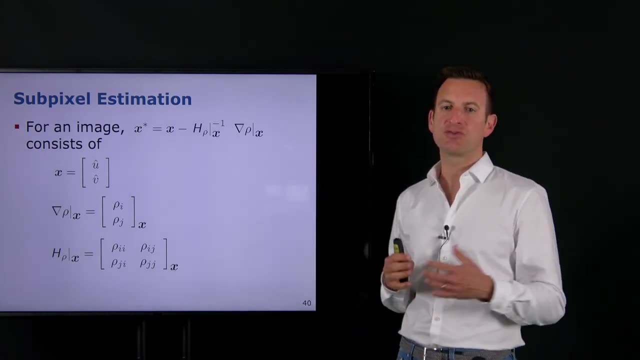 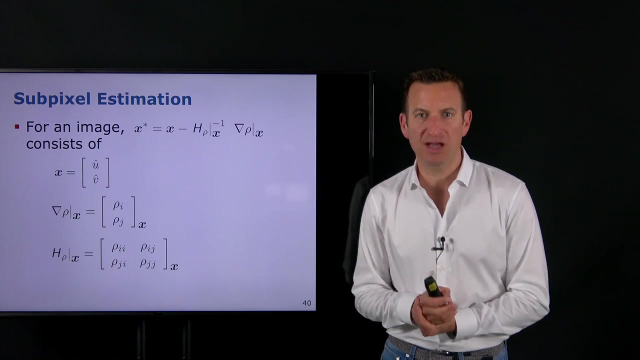 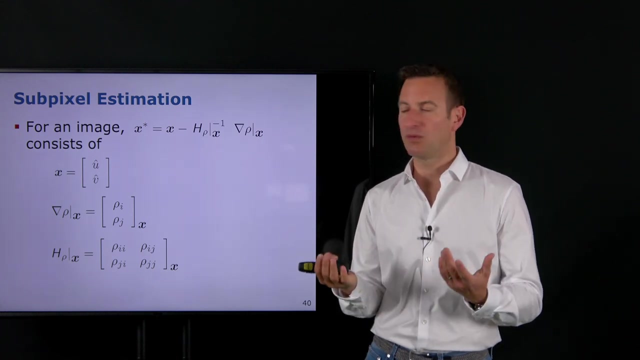 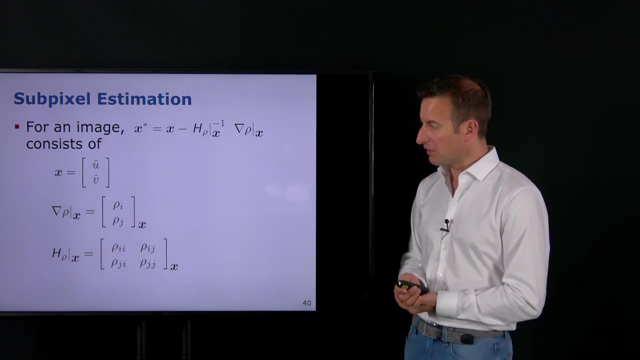 consisting of the partial second derivatives, arranged here in this matrix form, computed at the location x, Also this NCC function, which I can interpret as an image. And now, if you take the gradient and the Hessian matrix, and this is something, 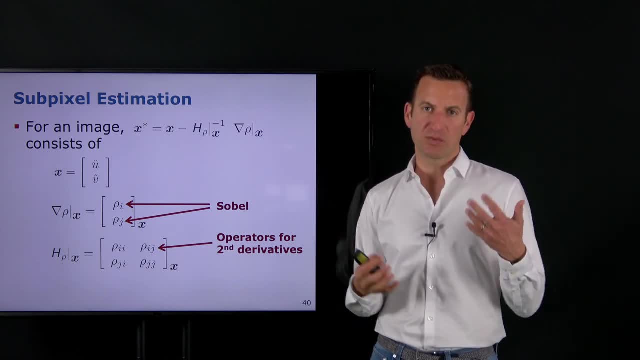 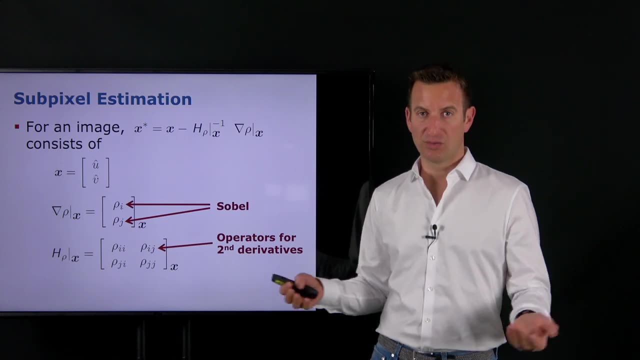 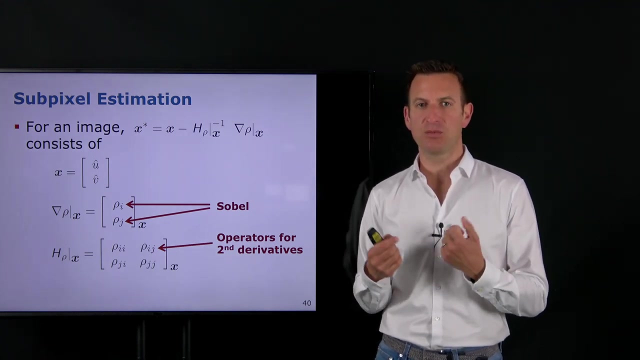 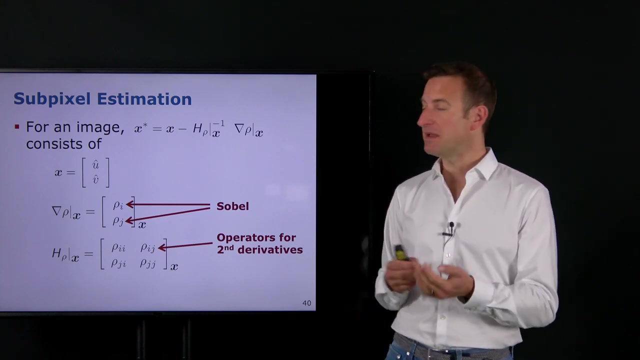 that we can do, for example, with our Sobel operator, as well as with our other operators for the second derivatives that we have defined based on the convolutions. So basically, we haven't exploited when computing the first derivatives of images. 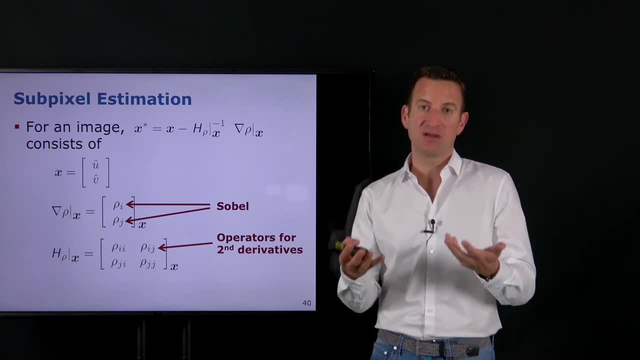 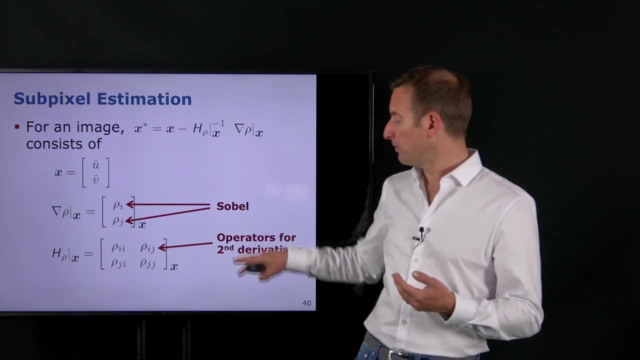 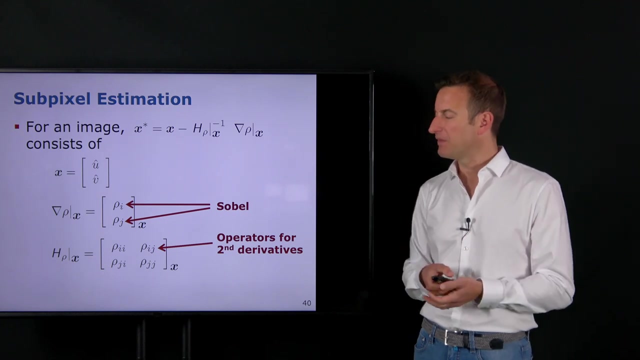 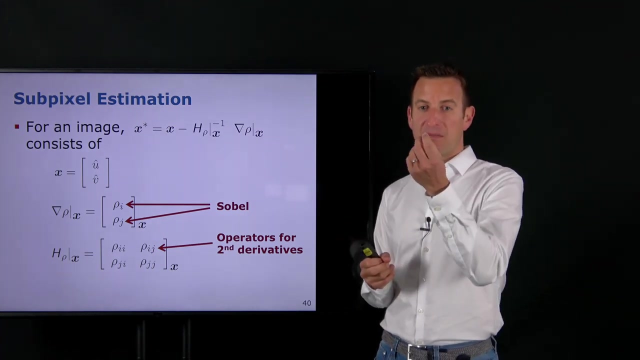 Just as basically, it's a discretized 2D to 1D function which we have only discretized locations, and that's what the NCC perfectly is. So what we basically do, what we actually do, is we: 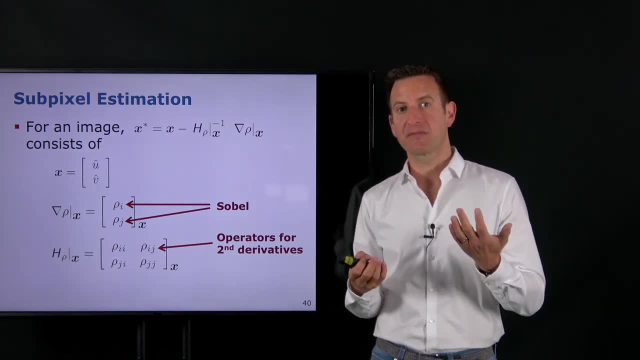 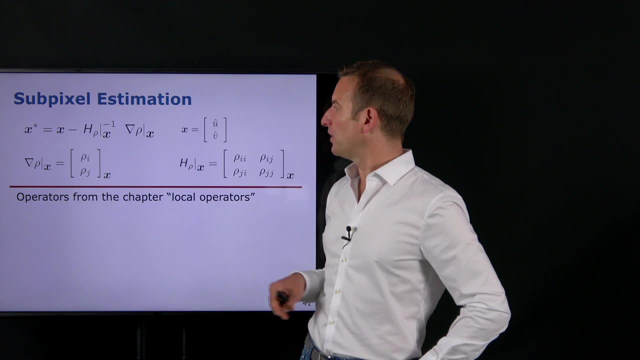 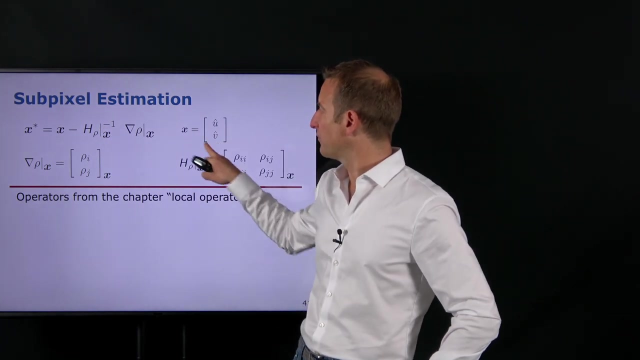 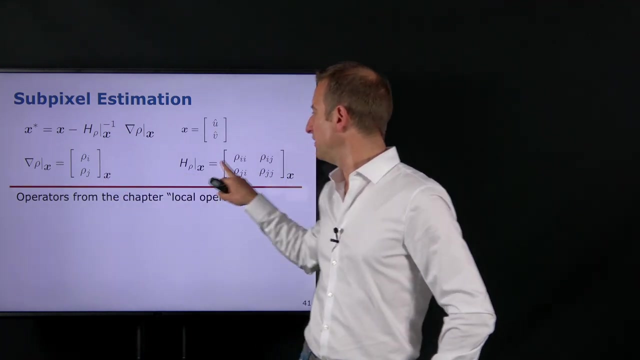 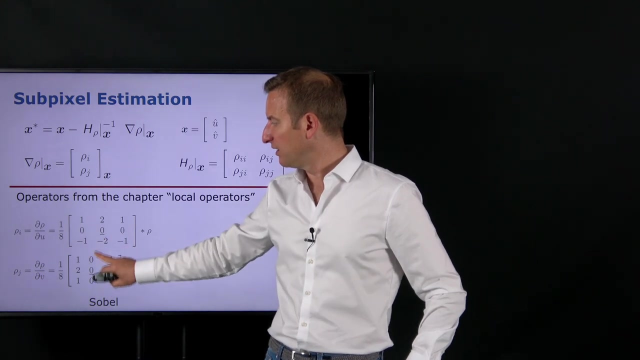 have a function where we run our exhaustive search for, but doing this only in the local neighborhood where the function, where I actually found the maximum value. Okay, so we compute the first and second derivatives and if you go back to the chapter on, 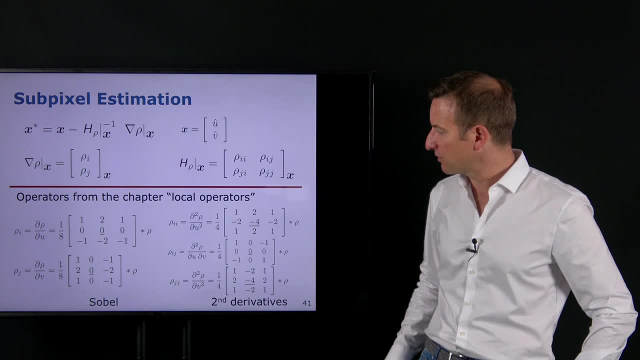 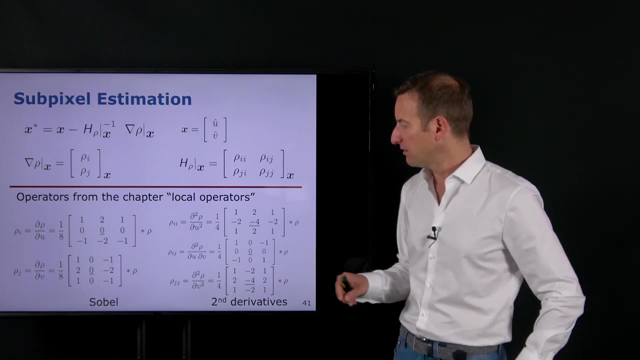 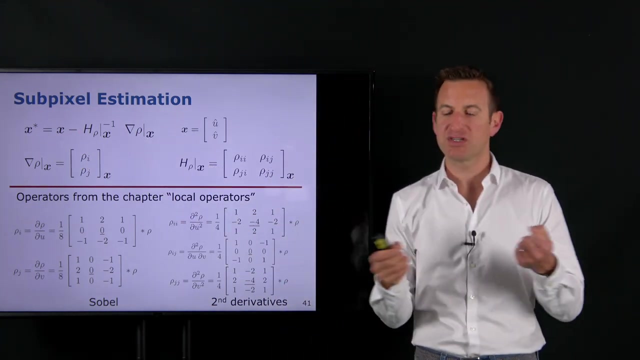 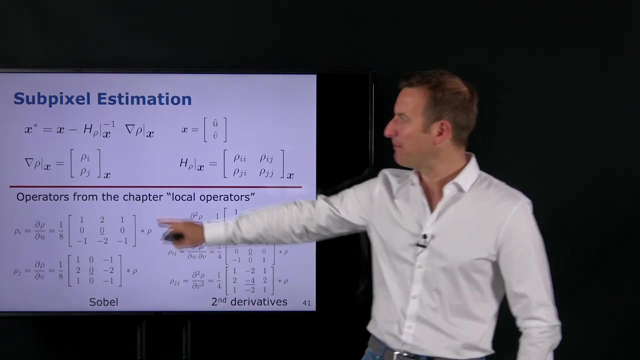 the local operators. this was my, have been my, my operators and I have the operators for the second derivatives and I only need to convolve them with my function row. so I only need to convolve them with my function row. 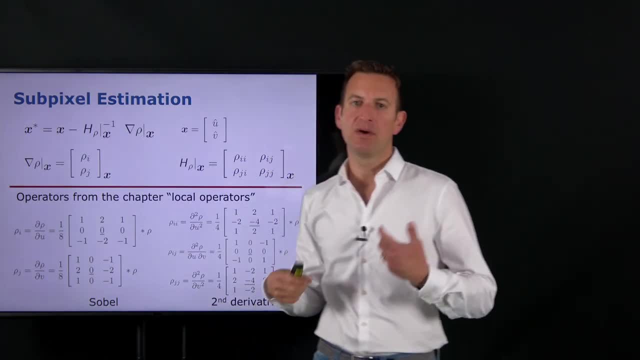 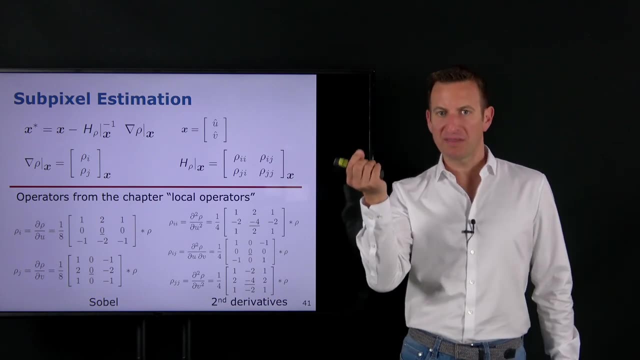 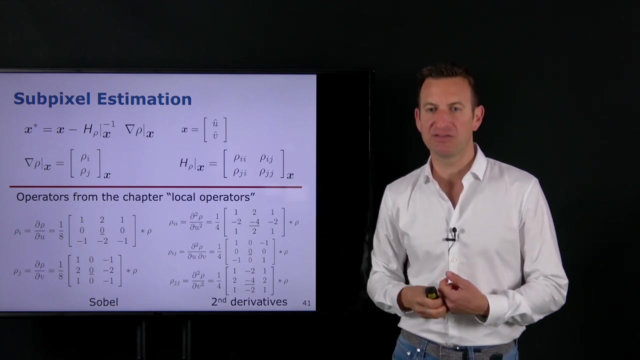 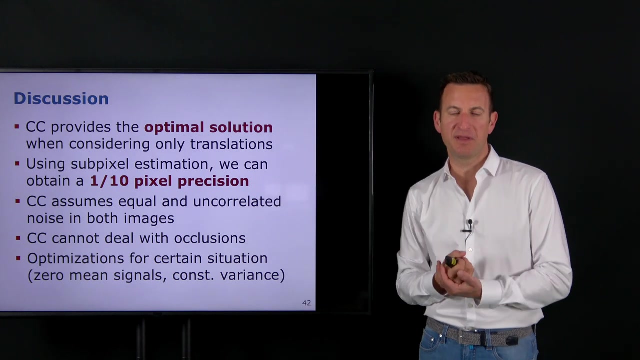 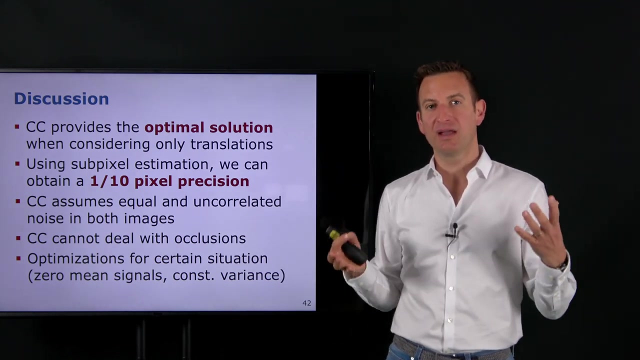 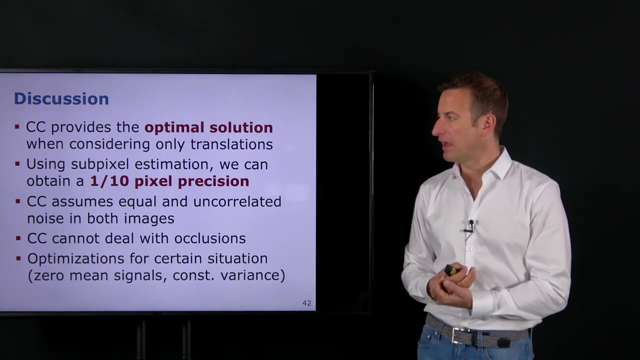 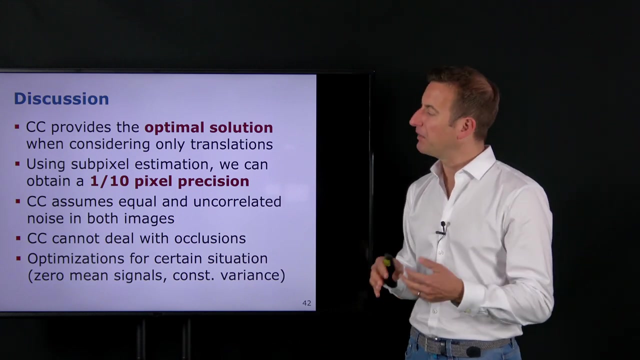 and I only need to convolve them with my function row. and I only need to convolve them with my function row. So here's the value for the number of derivatives that fit on the column matrix. Here's the number of derivatives that. 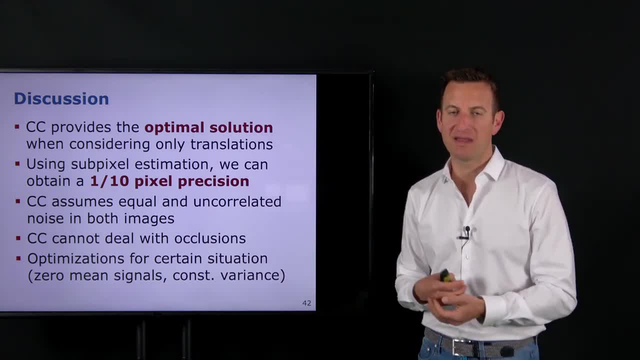 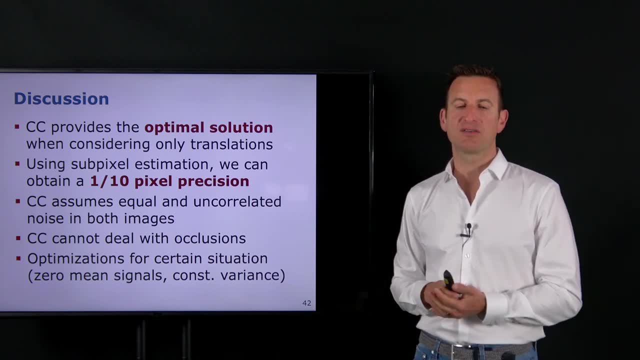 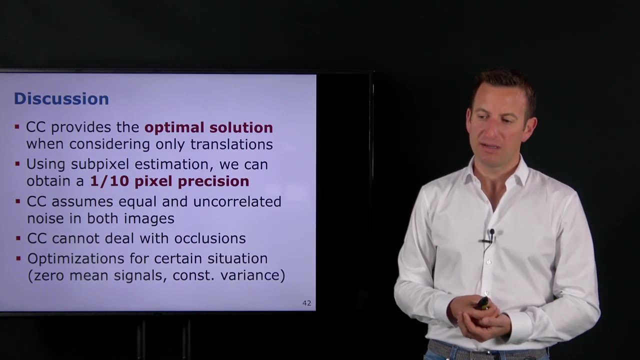 I need to having a locally quadratic form and then estimating this maximally quadratic form And the cross correlation actually provides us with an optimal solution if we only take translations into account and only the radiometric transformations, or having this measure, which is invariant under the brightness and contrast changes of our 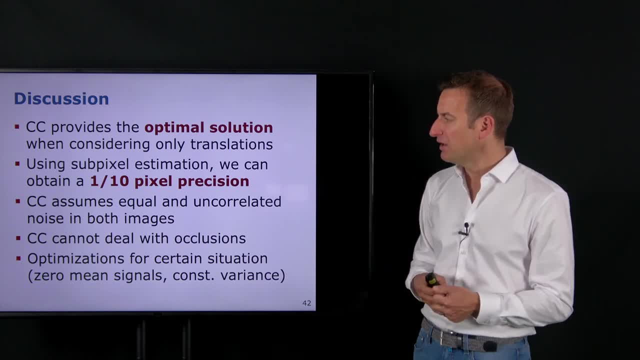 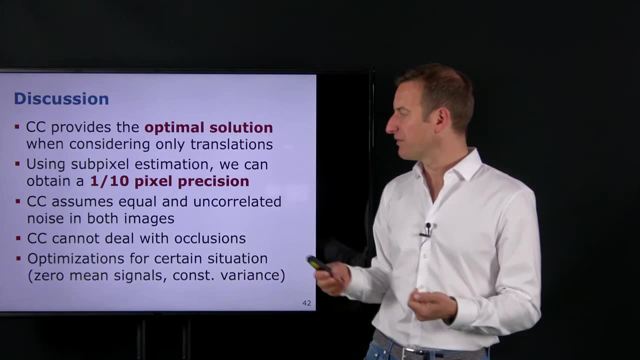 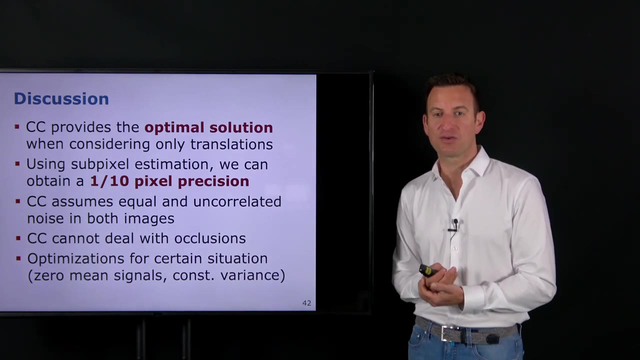 image. There are also some assumptions which are involved in here, so that we have equal and uncorrelated noise between those images and, of course, if we get rid of those assumptions, then things can be will get more tricky. and also what we should take into account, something that cross correlation. 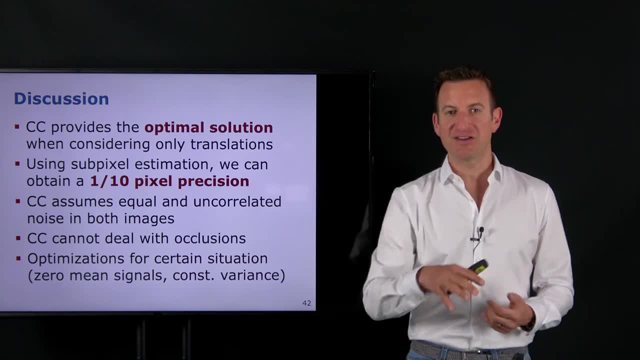 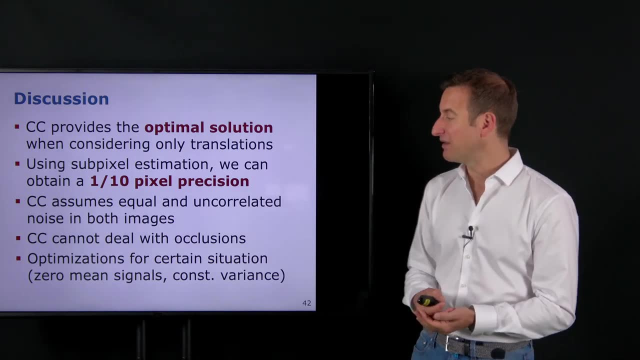 can't deal with are things like occlusions. So if you have a bird flying underneath your airplane while you're taking the image and the bird overlaps, that local region you actually will not find will not be able to find the matching position, at least if the bird is close enough to the airplane to cover a. 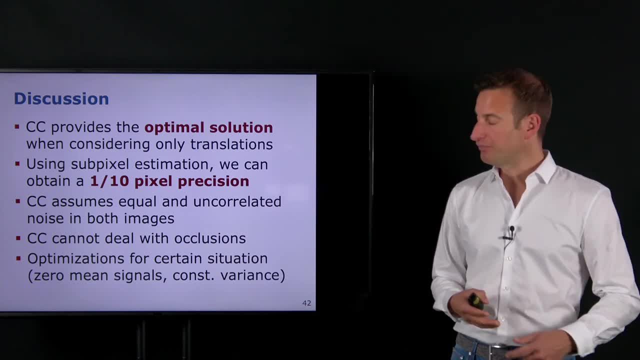 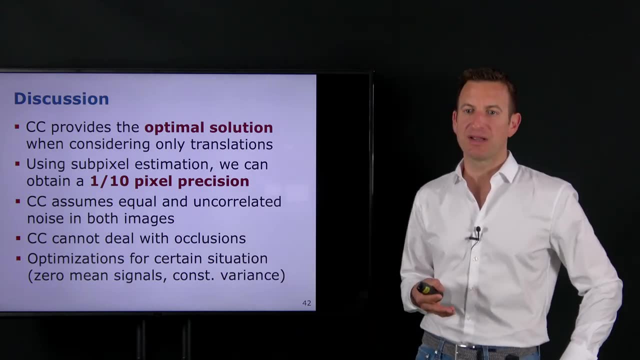 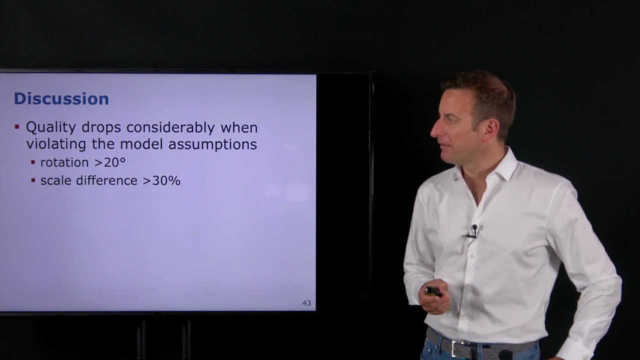 substantial part of your local patch. And again, just to set that there are optimizations for certain situations, extensions of cross correlations and how you actually can do better or adapt to certain local setups that you may have. Also, if you change or violate the assumptions that we had before, 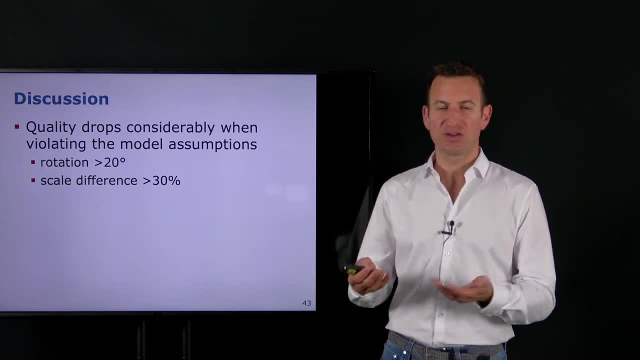 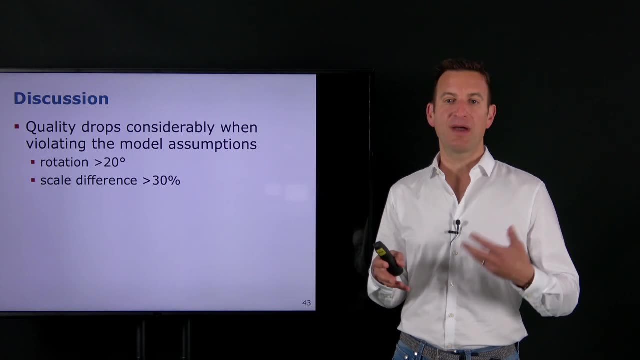 especially with respect, that it's only a shift, that's something that's not always realistic. and if you violate those assumptions, still, cross correlation works not too bad. if you have a cross correlation, Let's say a rotation of five degrees, for example, if you're going to something, 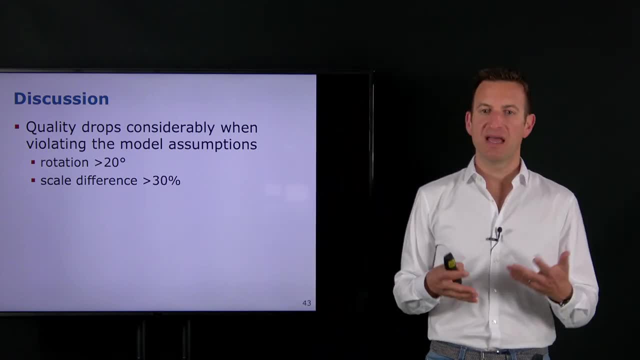 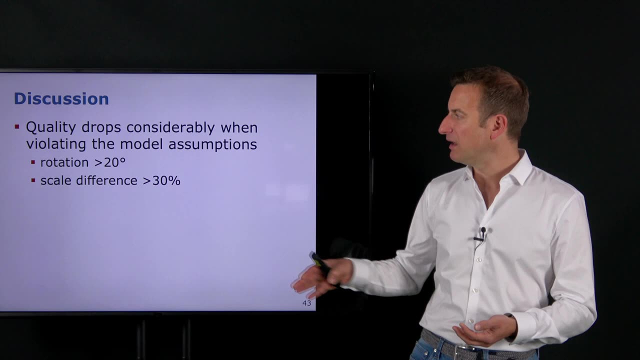 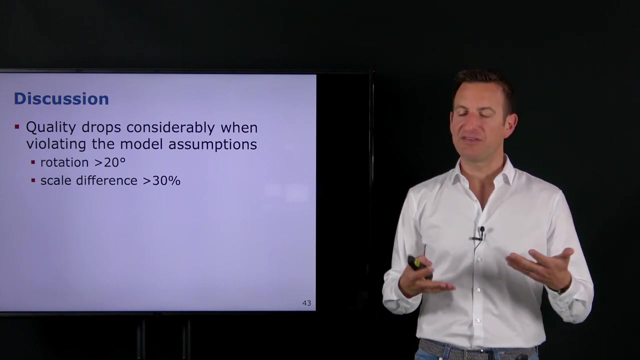 larger than 20 degrees or scale differences larger than 30 degrees, then you're violating your model assumptions substantially and typically don't get good results out of that anymore. If you stay substantially below those values, you can still apply cross correlation and get reasonable results on this, unless 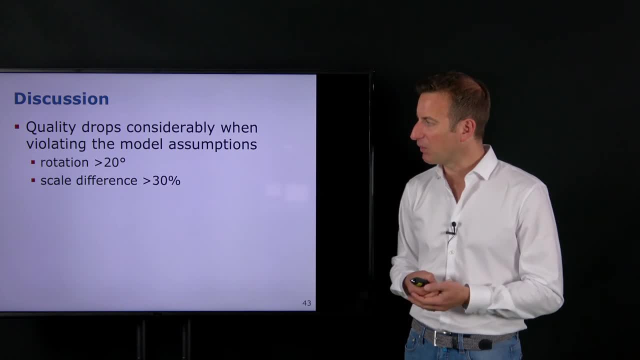 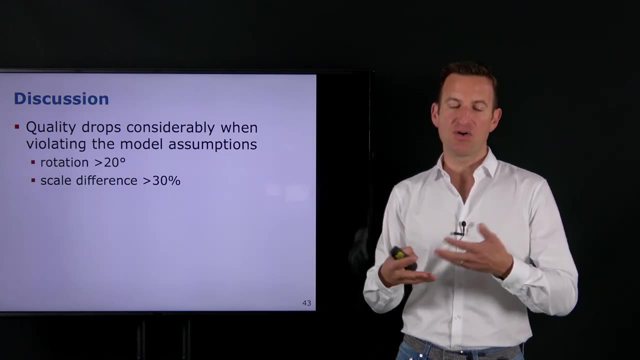 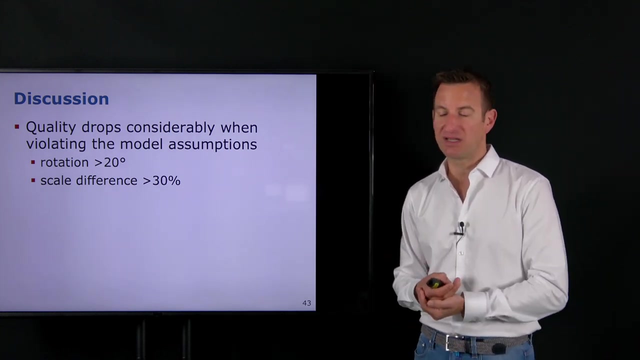 your environment's very ambiguous, for example, then the question is how well that actually would work, or if the violation of those assumptions doesn't create artifacts or noise which is larger than those of the then the variations that you have in your original image. So be careful if you are above those values that are indicated over here. 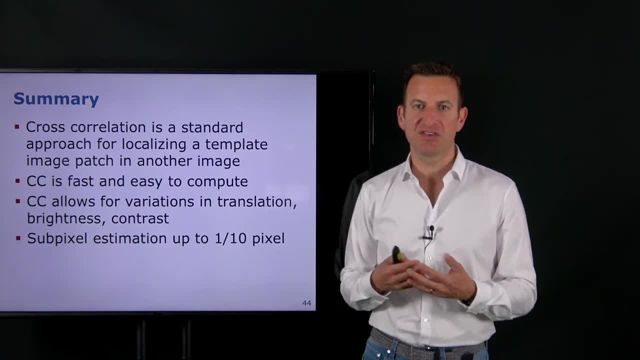 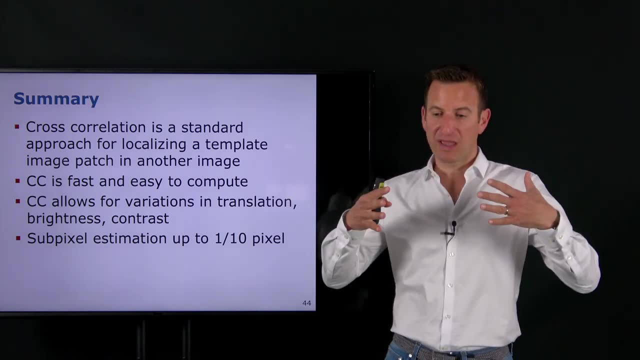 Okay, with this, I'm coming to the end. in template matching, Cross correlation is a standard way to perform this template matching. There are again four certain setups, other ways for doing this. so, for example, if you have your stereo camera and you know that there is a different, 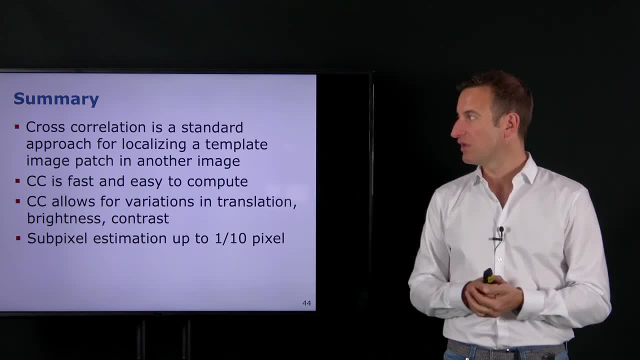 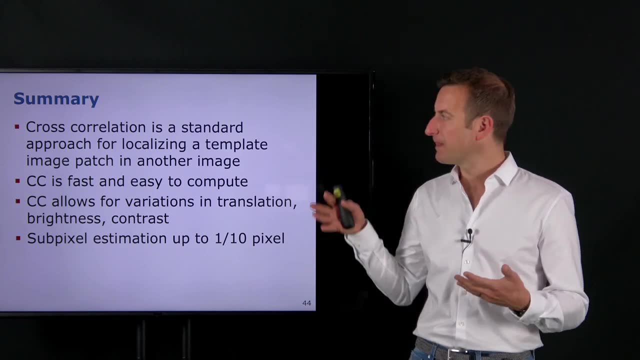 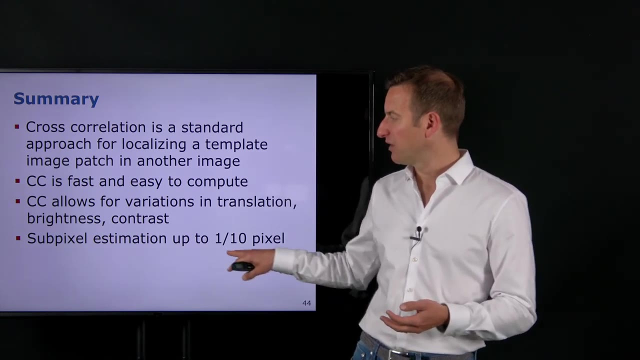 orientational change of your camera. maybe that's not the best choice to use cross correlation. you may want to explicitly take into account those rotational informations, but as long as you have only translations, that's a standard way to do it. It's easy to implement fairly fast if you only work in 2D and with this sub. 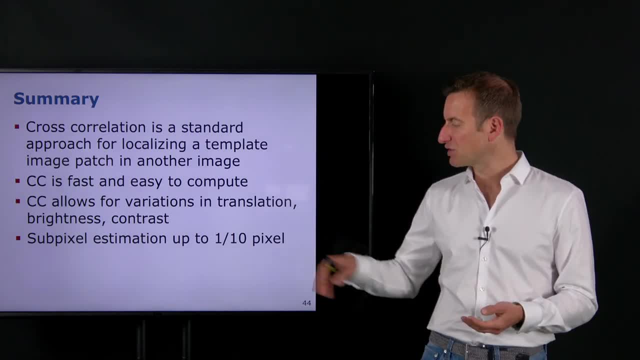 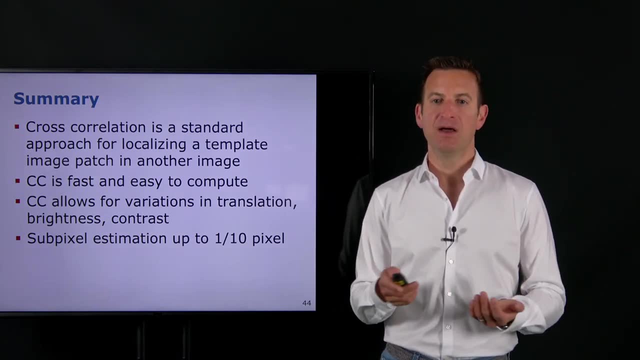 pixel estimation, which can also be done very efficiently, you actually get a quite accurate matching of up to a tenth of a pixel. With this, I'm coming to the end of this presentation, coming to the end, and I hope you learned something on how to find data.